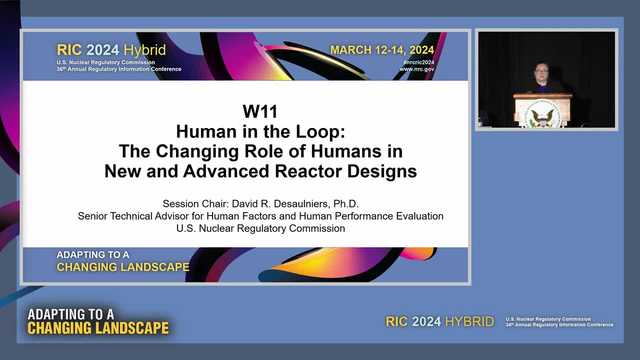 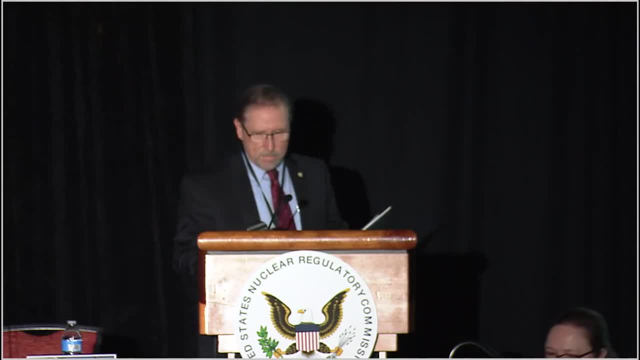 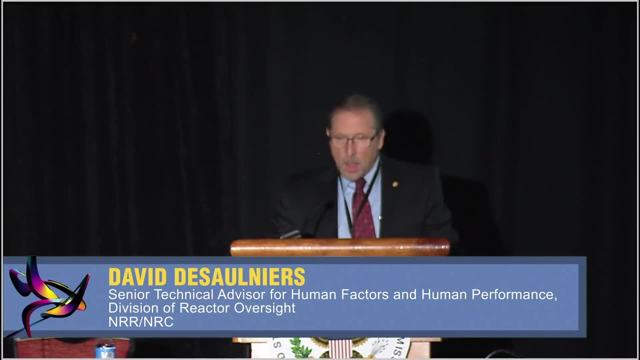 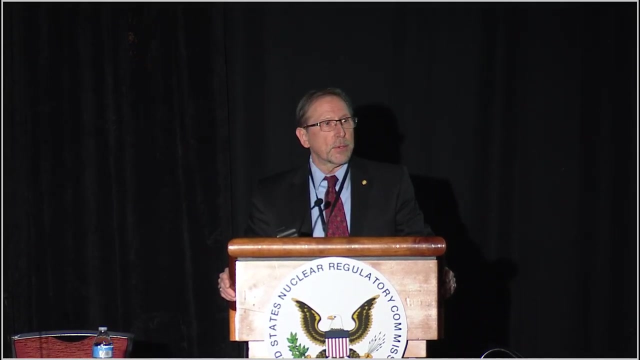 Don Miller Award. Please welcome Dr David DeSauniers. Thank you, Stephanie, and good afternoon everyone. I hope you had an enjoyable time and a good, enjoyable lunch, perhaps catching up with an old colleague, or perhaps making a new acquaintance. If it was a new acquaintance, I wish that person many years from now is. 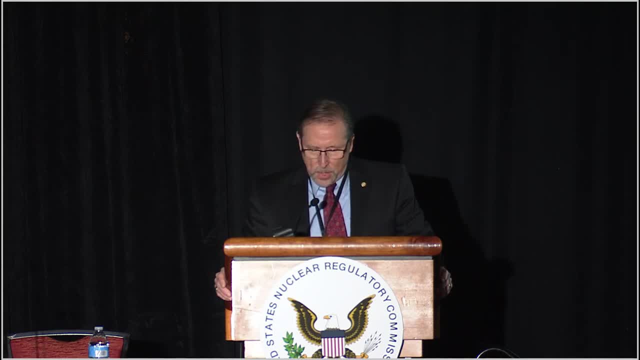 one of your old friends. The RIC is a wonderful opportunity to meet people who can enrich our professional lives and share information that help us achieve our goals. I hope you'll join me in taking full advantage of these opportunities. About a week ago, I looked at the registration for this session and was elated, and, frankly, 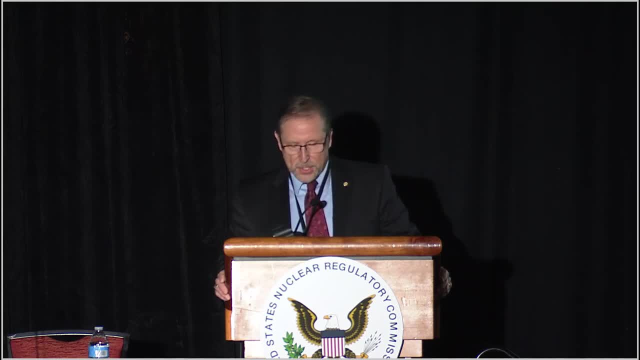 a bit daunted to see that we had over 700 attendees registered for this session, either online or here in the room, And I had to sit down for a minute and do the math And it dawned on me this audience is about 700 times larger than what I'm used to speaking. 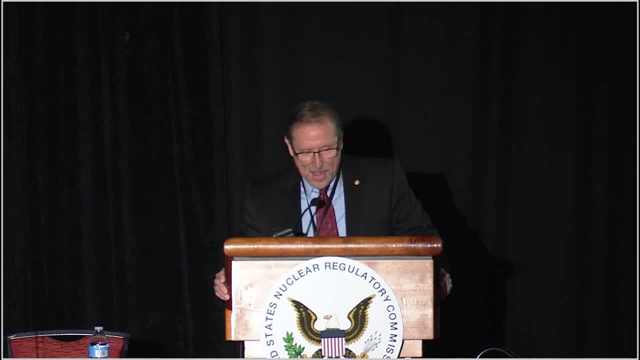 to The engineers in the audience, have probably done the reverse calculation and figured out that means he's used to speaking one-on-one with people, which is true. That's my preference, So, if you'll indulge me, I'm just going to imagine that this is a one-on-one conversation. 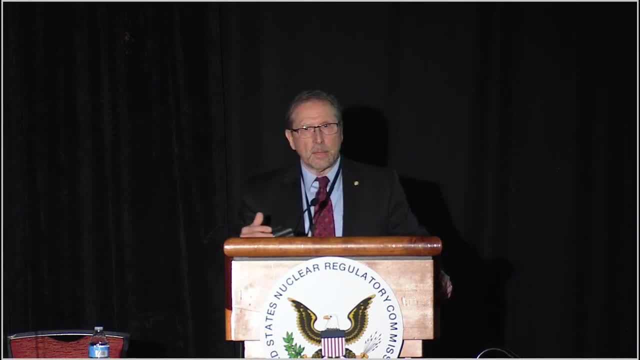 with you all- That is, 700 of you- in parallel, And feel free to do the same if it makes you feel more comfortable. It is my honor and pleasure to chair this session of the RIC. It's an honor because I get to share the stage with a wonderful panel of speakers. They are: 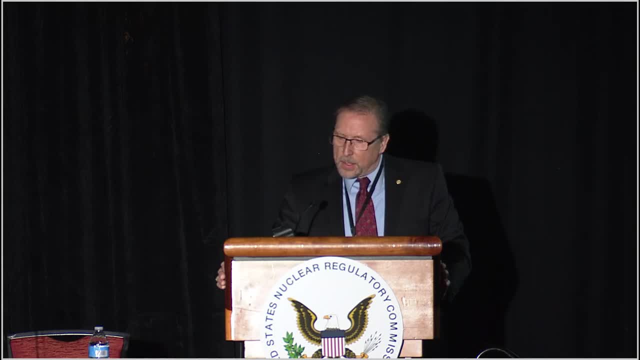 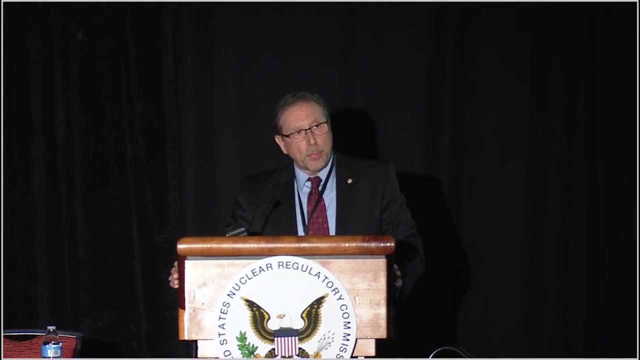 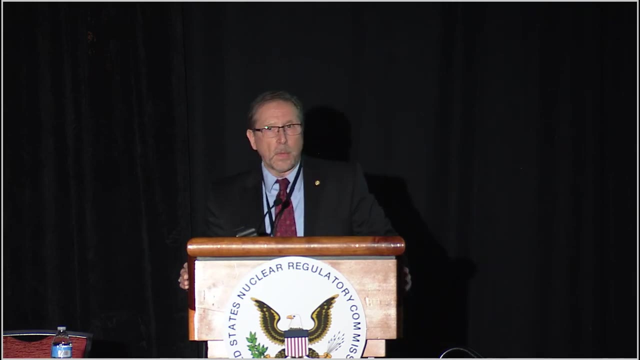 bringing to our discussions today a tremendous depth and breadth of experience in the application of human factors to the nuclear power domain. It is my pleasure to chair this session, as they will be discussing a topic that I believe is exciting, relevant and important. Those 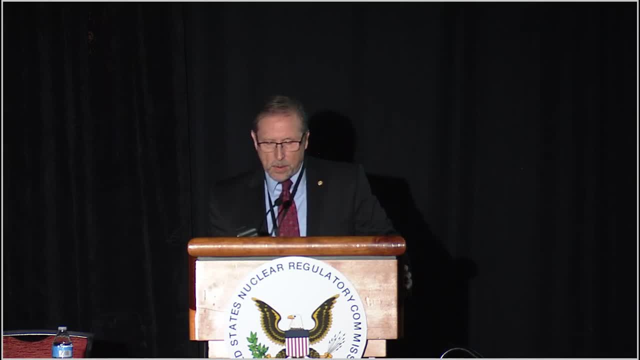 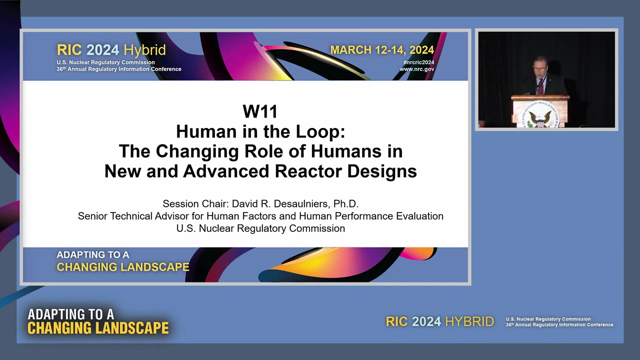 of you who have heard me speak in the past have noticed that, rather than quickly moving past the title slide, I'd like to dwell on the words of the title as a means of introducing a topic. This session is titled Human in the: The Changing Role of Humans in New and Advanced Reactors. Those of you who have been around 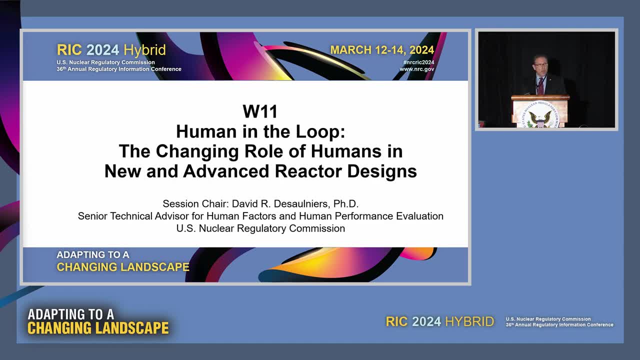 a while, either in the field of human factors or perhaps design testing, are likely familiar with the older term man in the loop. Now, we did not use that term, in part because we recognize that man in the loop is a sexist phrase But, more importantly, human is a term. 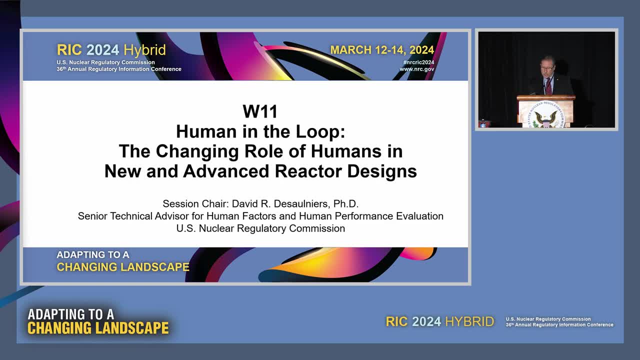 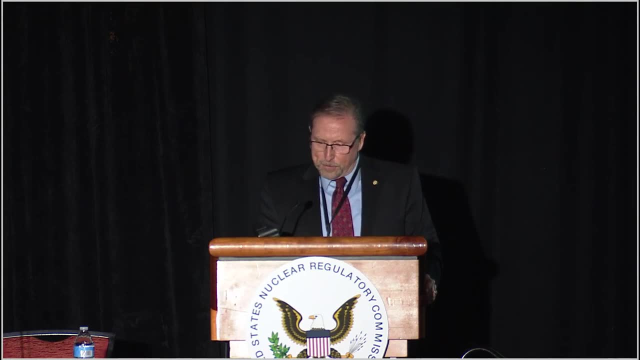 that is much better at capturing the rich and diverse considerations that should be taken into account when considering the role of individuals and groups of individuals in the operation of nuclear power plants. So why do I say that? Well, I think it's important to understand that the role of individuals and groups of individuals in the operation of nuclear power plants. So why do I say that? 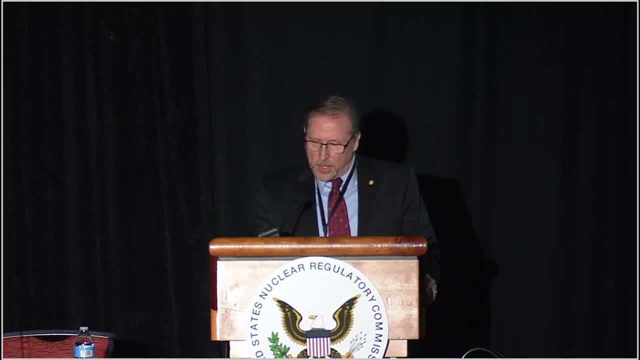 For many of you, the phrase man in the loop is likely to conjure up the rather dry list comparing the capabilities of men to the capabilities of machines. The acronym was MABA MABA. Men are better at, machines are better at, Hence MABA MABA. 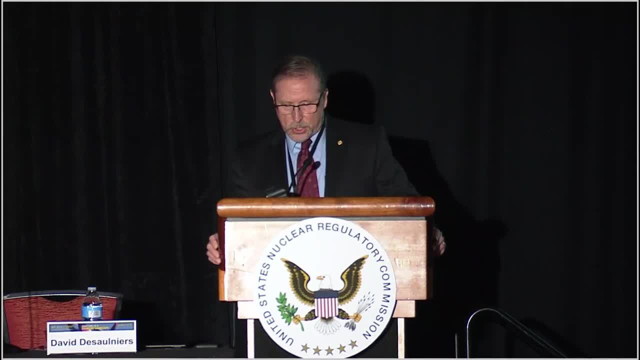 In these MABA, MABA lists, you would likely find items such as machines are better at repetitive tasks. Not surprising: machines don't get bored and their attention doesn't fade. Another example: machines are better at doing complex calculations. But now I want you to consider what might seem to be a philosophical question. 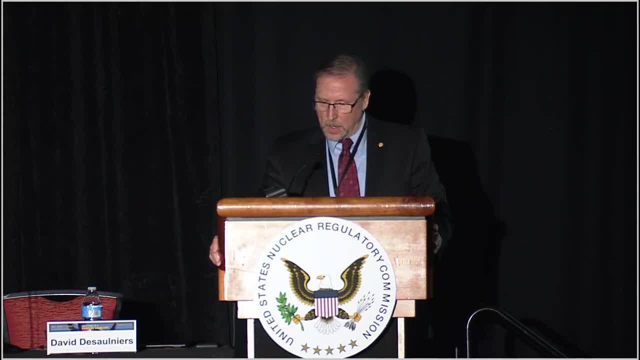 What does it mean to be human? What makes you human? Well, the answer is yes. Each of you may have a somewhat different answer to that question. Whatever the answer I expect if you now think in terms of human in the loop rather than man in the loop- 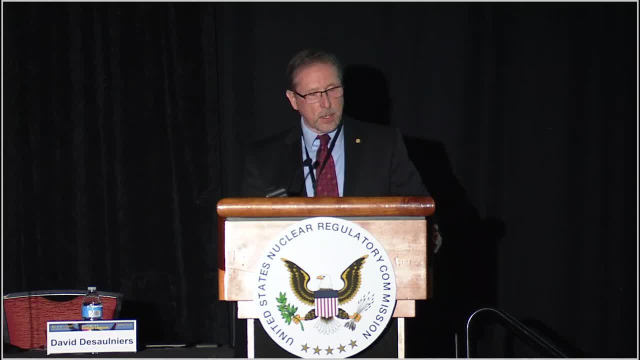 your thinking expands beyond basic considerations such as whether a man or machine is better at doing repetitive tasks. With that, I hope I have whetted your appetite for our panel discussion, Thank you, Thank you. So far I've given you the panelists' views on how the role of humans is likely to change in the operation of new and advanced reactors and what might be some of the most important considerations or implications of such changes. 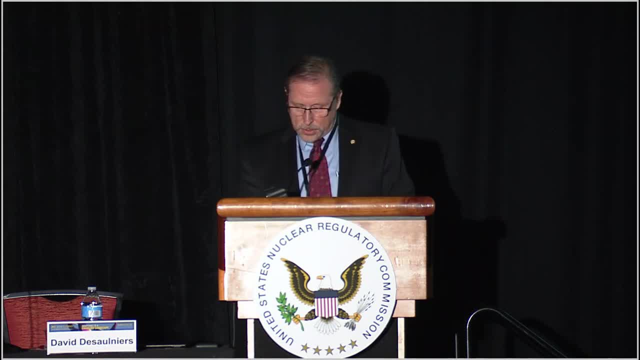 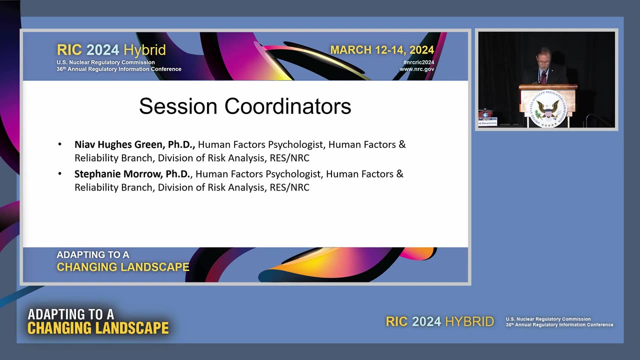 Now, before we get to those presentations, though, I want to take a moment to acknowledge the individuals that have made this session possible. Those are our session coordinators, Stephanie and Nia- would you please stand up? the coordinators for this session. these are my wonderful colleagues dr Nia of Hughes green and dr Stephanie Morrow, both. 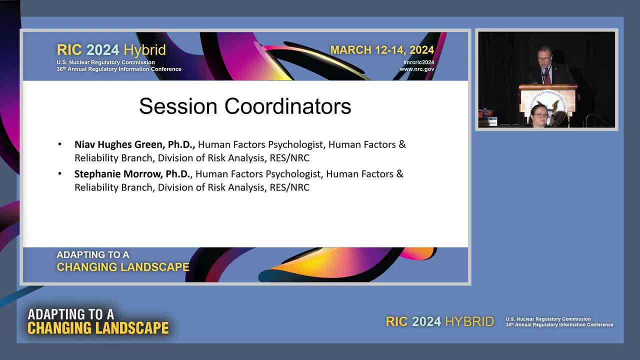 are accomplished human factors, psychologists and researchers and NRC's office of nuclear regulatory research. you've already given them applause, but let's give them another applause for bringing together this wonderful session. there is a lot of work that goes on to to make these things possible, and I really appreciate all the work they put into it. now I'm gonna briefly 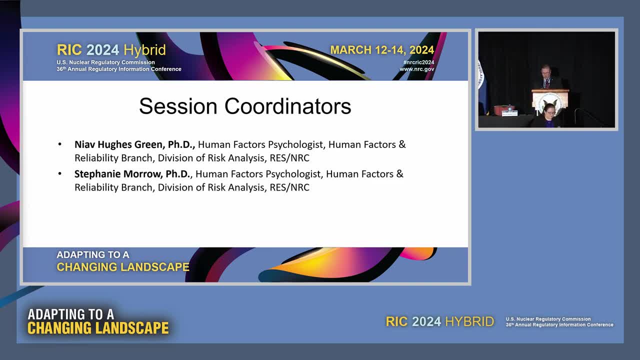 turn over the mic to Stephanie, who is going to speak to us a little bit about QR codes and other logistics. sure, can we start with the first question and then we'll move on to the next question. we have the QR code back up on the screen, please, and for this session, we encourage you to submit. 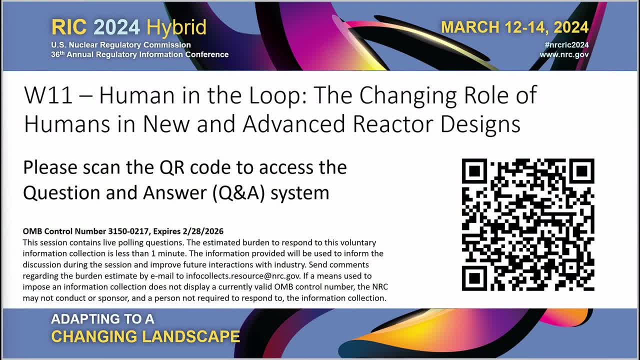 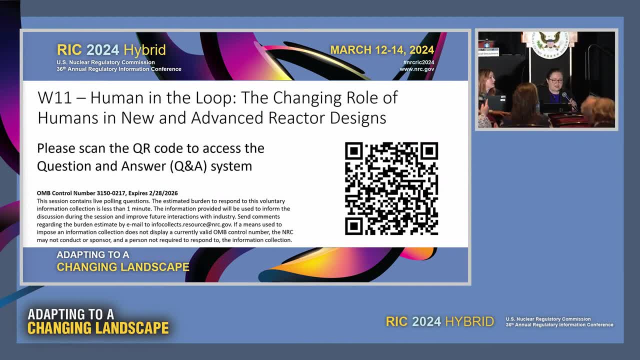 questions throughout the panel for those in the session room. please take a moment to scan the QR code displayed on the screen so that you can participate in both the Q&A and the live polling during this session. again, take a moment right now to scan the QR code. it'll be much easier as you go. 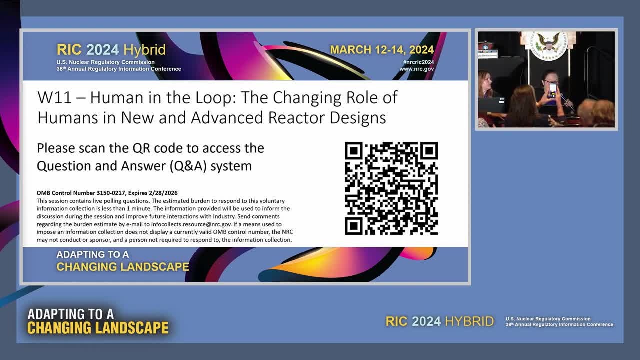 along for those of you joining virtually. you'll find there's a box to the right of your screen with tabs for electronic Q&A live. you'll find there's a box to the right of your screen with tabs for electronic Q&A live, polling and feedback. 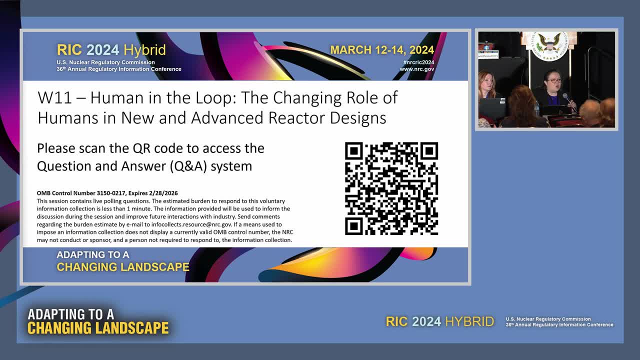 You can direct questions to either a specific panelist or what we would ask is: there is an option that says USNRC staff? If you have a question that would apply to any panelist, please select that option: USNRC staff. 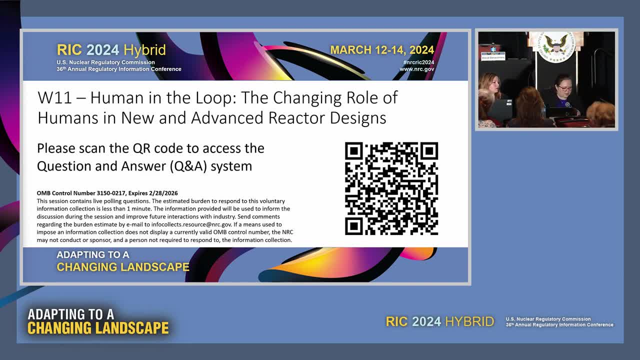 to pose a question to the entire panel. We will also be incorporating live polling questions into our session today. For those of you in the room, there is a poll option on the same web page where you submit questions on your mobile device accessed with, again, the QR code displayed behind me. 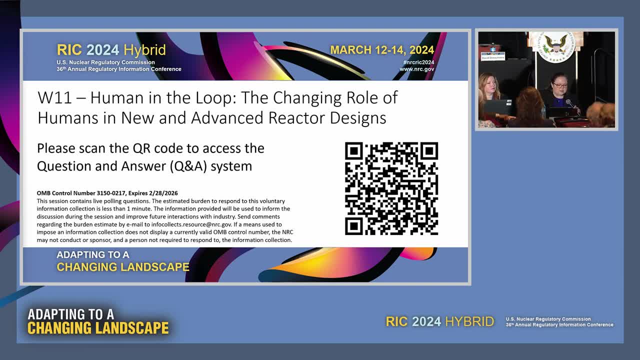 In-person participants can also participate by texting their choices to 22333.. When we introduce a polling question, there will be a slide displayed in the room with the instructions for participants to text their responses. For those of you participating virtually, once you've logged into the virtual conference platform. 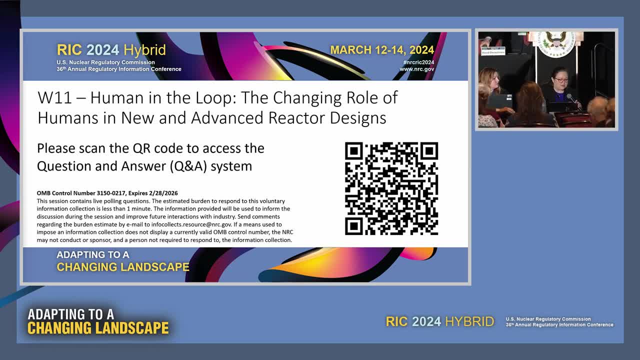 and joined the session. there again is a tab to the right of your screen for live polling questions. The polling results will be displayed on the screen to reflect responses from both our in-person and virtual session attendees. Thanks, Dave. Thank you, Stephanie. 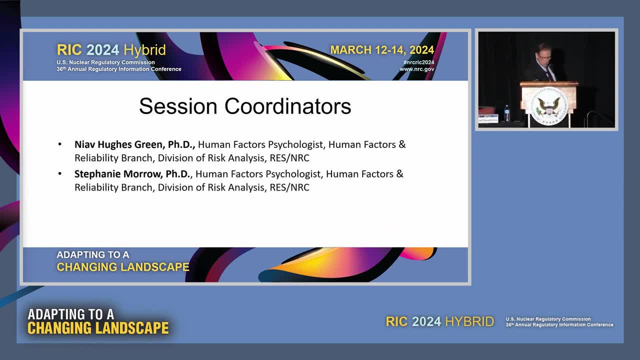 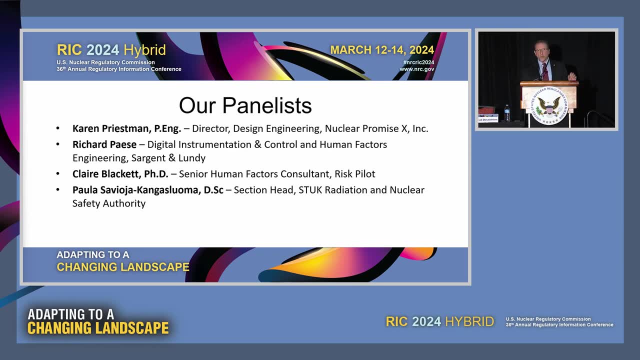 OK, hopefully you've all had your opportunity there to get that QR code, so I'm now going to move on to the next slide. Just going to, at this moment, provide a brief overview of our panelists. I will provide a more fulsome introduction of each of them. 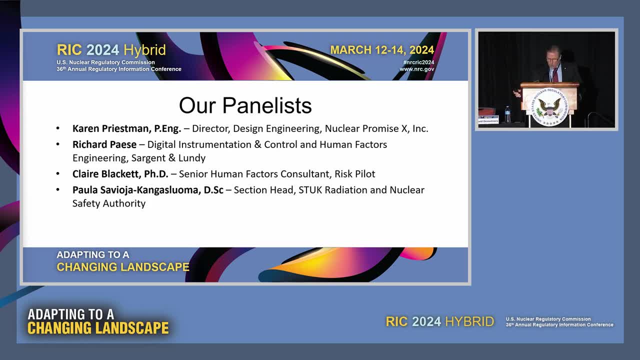 as they come to take the podium. What I want to point out at this point is that, as I noted before, we have a great depth of experience and diversity in our panel here. Kicking things off for us will be Karen Priestman of the Canada-based nuclear engineering service firm. 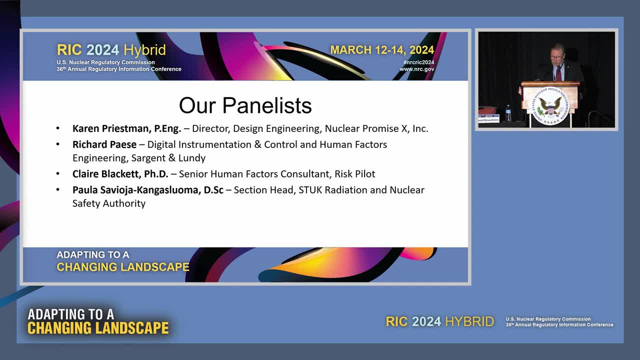 Nuclear Promise X. She will be followed by Richard Pace of the power and energy consulting firm Sargent and Lundy. Then we'll have Claire Blackett, currently of the risk management consulting group RiskPilot and formerly a researcher for the Institute for Energy. 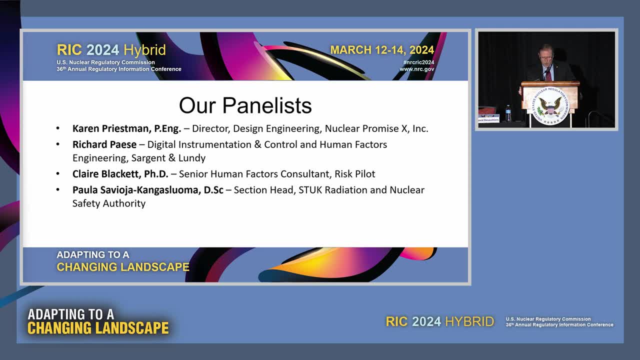 Technology in Norway And Claire will be followed by Paula Savioia of the Stuk Radiation and Nuclear Safety Authority of Finland. I will provide some remarks to follow, but again collectively, our panelists. We'll bring perspectives from their work in different types of organizations. 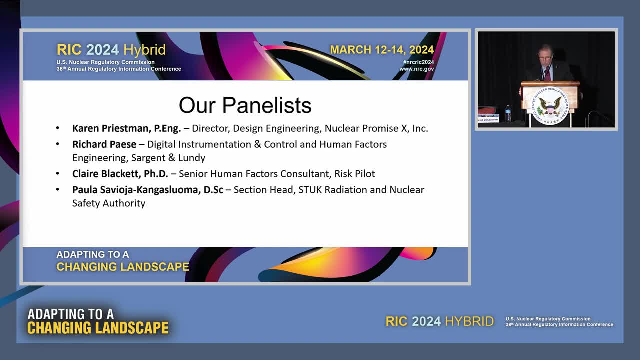 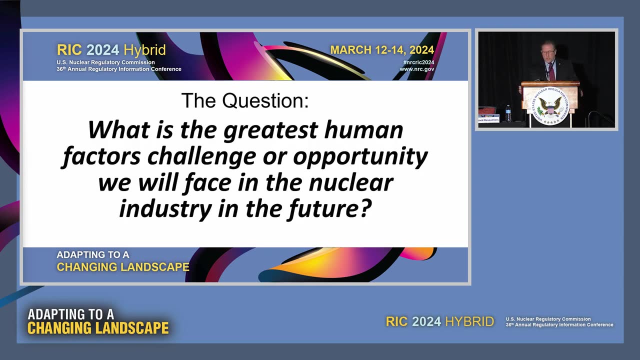 as well as different countries. Each will make a brief presentation and then we will make plenty of time available for audience questions. So those presentations that you will hear from each of our panelists- we've asked them to adjust this particular question as part of their presentation. 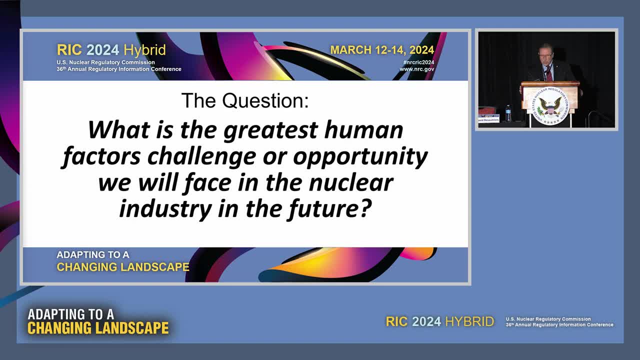 What is the greatest human factors challenge or opportunity we will face in the nuclear industry in the future? Before we begin those presentations, we have a polling question for you, our audience members. The question will help our panelists understand your general familiarity with human factors, a field of study. 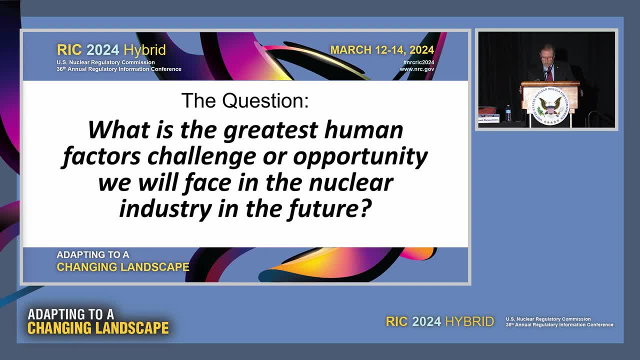 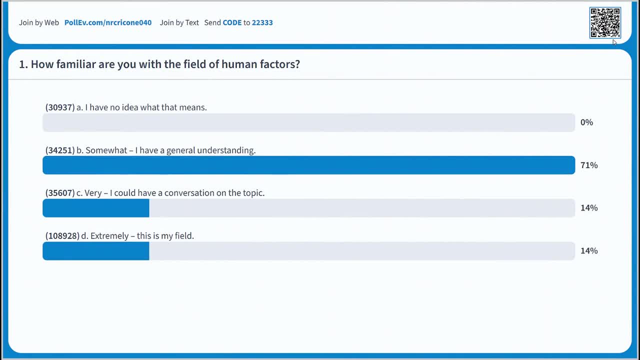 and a discipline that is central to the topic of this session. So could we put up the first polling question Please? So your question is: how familiar are you with the field of human factors? Glad to see that we have at least some understanding. 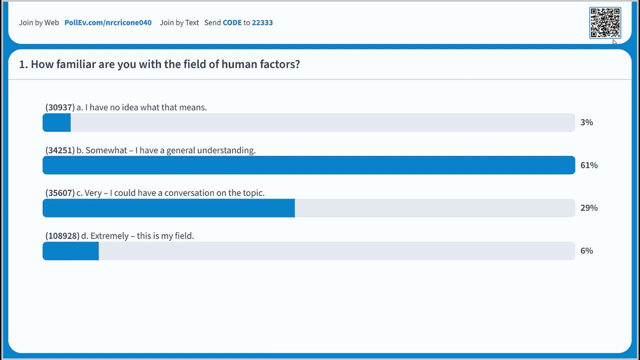 but not surprised to see if we have in some cases very little understanding, because it's been my experience over many years that there's many people out there that this is kind of a foreign discipline to them. But as these results continue to come in, 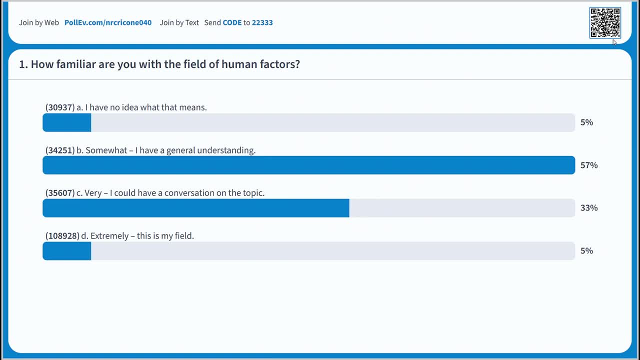 it is now my pleasure to introduce our first speaker, Karen Priestman. Karen started her career at Ontario Hydro, the precursor to Ontario Power Generation and the company currently building North America's first small modular reactor. Throughout her 33-year career, Karen's career has been, I think. 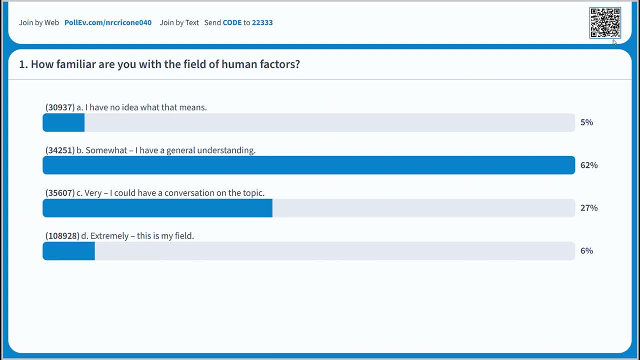 very relevant to my profession for sure. The fact is that in her career, Karen has worked and still going right 33, and still going. has worked in a wide variety of roles for consultancies, design organizations and manufacturers, and for 10 years, 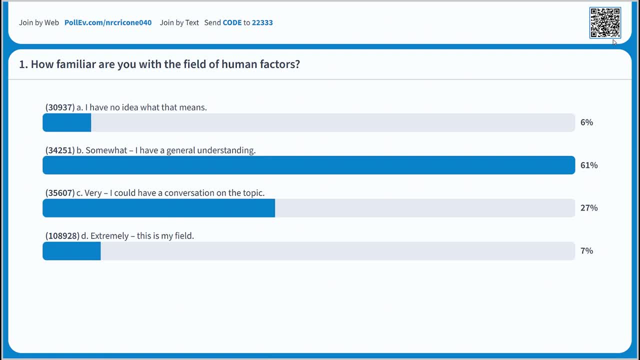 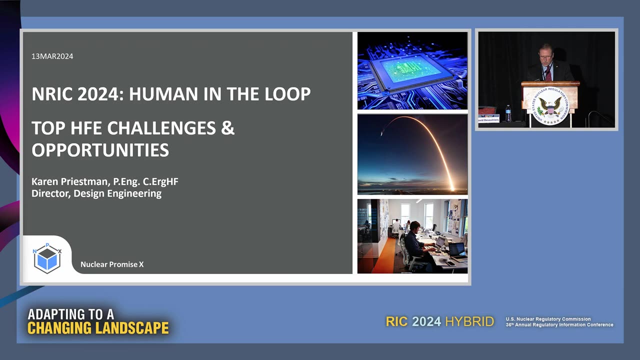 as an independent contractor. Karen's career has been a mix of both systems and human factors, engineering largely in high-hazard industries including defense, rail and oil and gas. For the past 18 years Karen has worked the civilian nuclear industry, most recently for Japan-based Hitachi GE and US-based GE Hitachi. 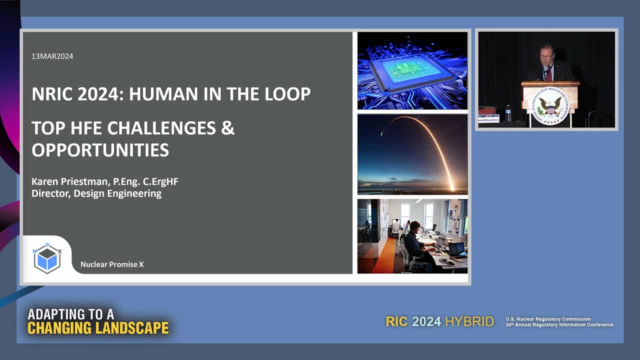 for whom she led high-profile and extensive human factors engineering programs as part of their new build projects. In January this year, Karen joined Nuclear Promise X, a company focused on supporting implementation of new digital technologies within existing and new plant designs. Karen has a Bachelor of Applied Science in Systems Design Engineering. 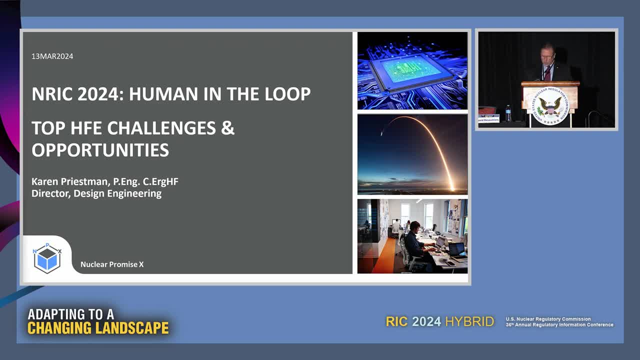 with a Human Factors minor from the University of Waterloo in Ontario, Canada. She is an Ontario-licensed professional engineer, a Chartered Fellow of the United Kingdom's Chartered Institute of Ergonomics and Human Factors and a member of the International Council on Systems Engineering. Please welcome Karen Priestman. 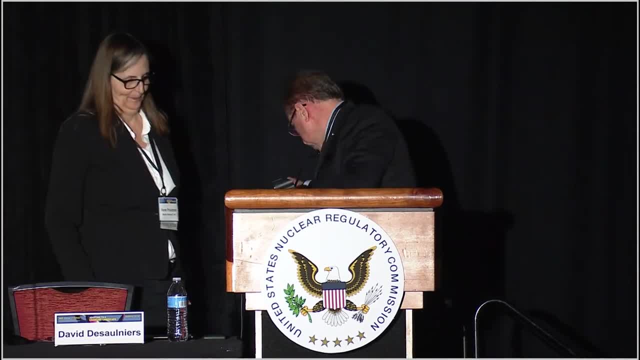 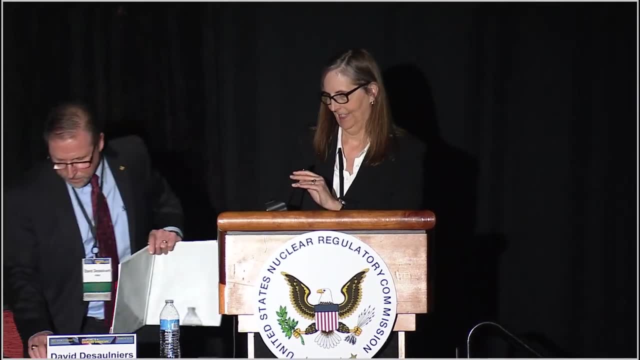 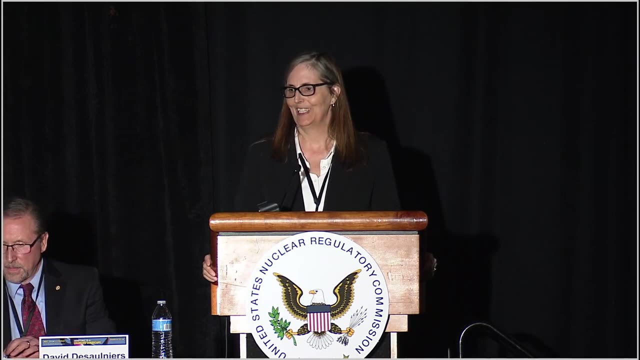 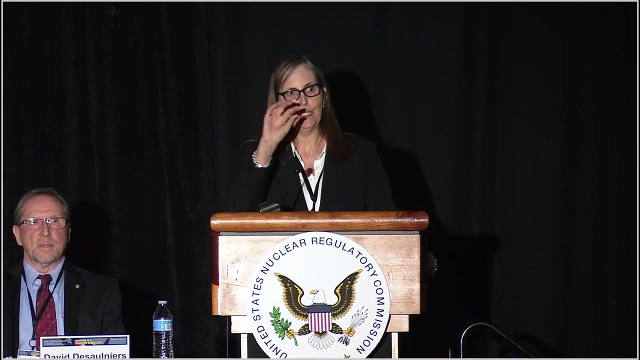 Thank you, Dave, And thank you everyone for attending this session. We know you have a choice of sessions to go to, so we appreciate you coming to this one. Dave's comment about speaking one-to-one: that light is so bright it pretty much limits who I can see, so it. 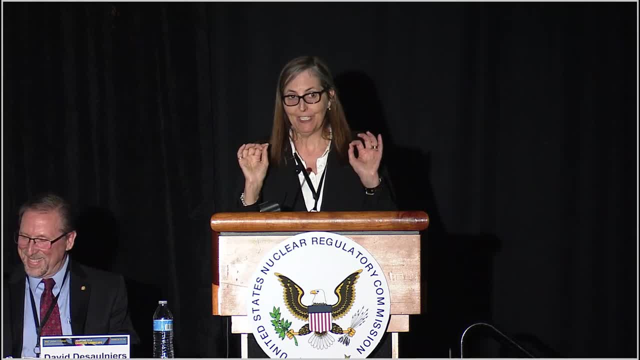 is almost like I'm speaking one-to-one. If we all have kind of a bit of a deer in the headlights, let's do that. That's why we've also got just for fun and games, we've got a timer there. so talk about. 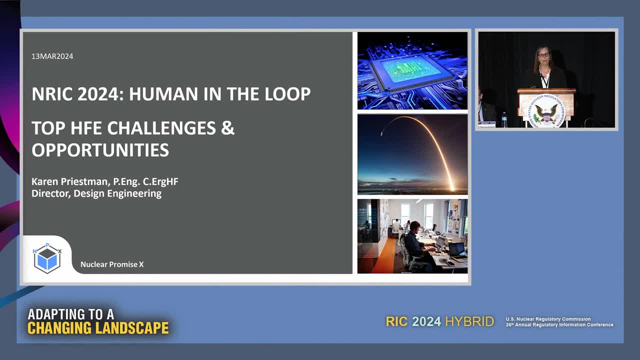 time pressure, But I will go fairly quickly through my slides. We want to leave enough time. I've just reminded Niamh to start it Through my slides. just a bit about Nuclear Promise X, because we are a new and smaller company, And then I will address the question. 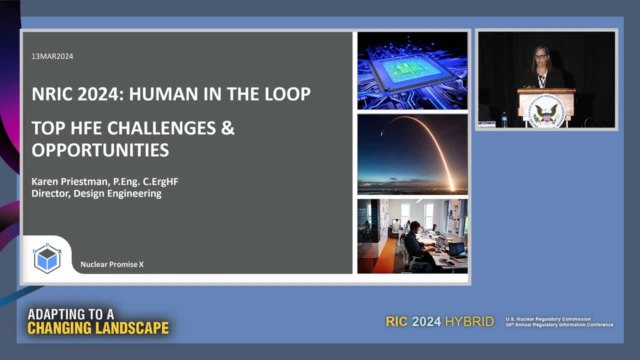 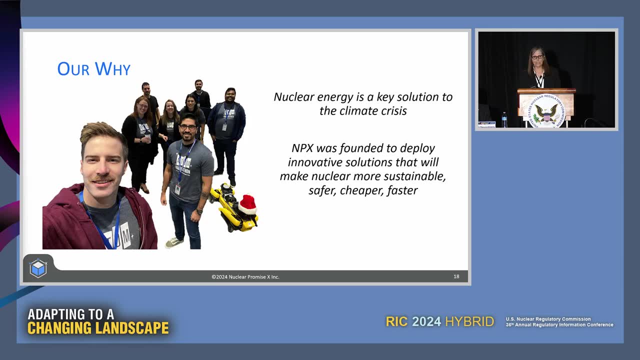 that was up on the slides, Dave's slides. Let's see if this works. Here we go. Nuclear Promise X was formed about five years ago and basically founded on the firm belief even five years ago, before this renaissance that we're going through, that nuclear was essential. 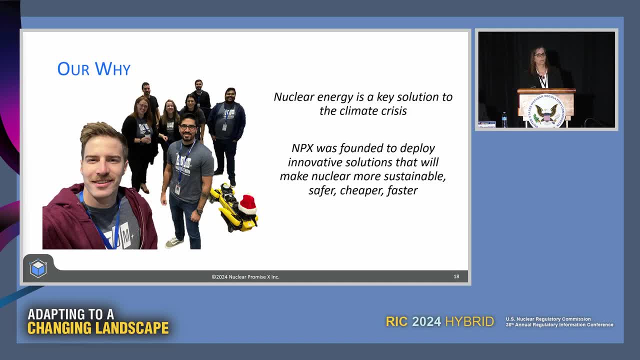 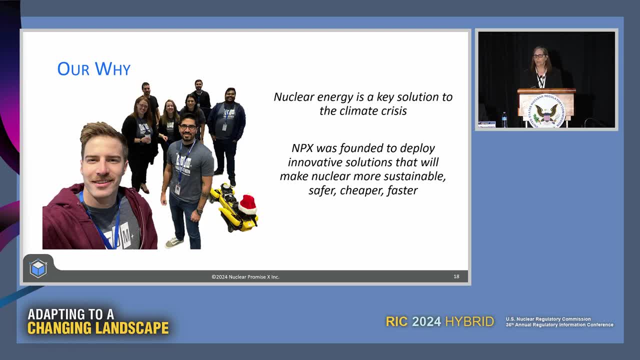 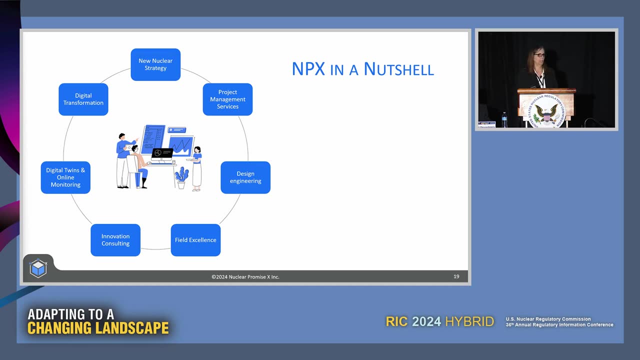 And I think that ties in with a lot of the content of this RIC. So we're pleased that that fits really well with us as a company. We started with- and I'll just move quickly through these- we started with sort of a products area, a lot of digital transformation, a lot. 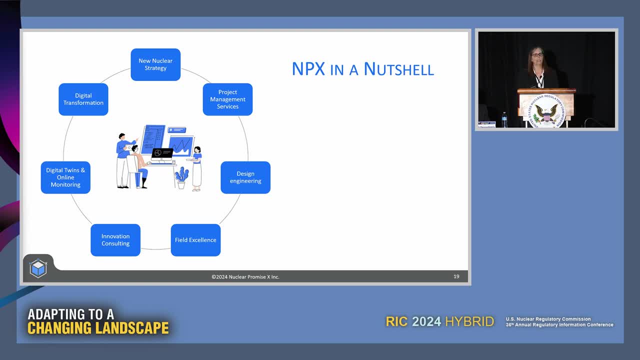 of robotics and digital twinning and even processes making highly digitalized processes that were quite document-centric before And recently. the last two years we've delved into the services We do: project management, using our digital tools, of course, and design engineering, which is now my baby And my. 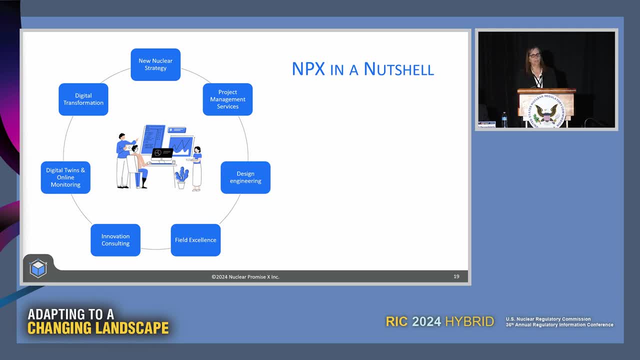 goal is to move the needle on how we do design engineering in the nuclear industry. So I have a stated agenda. I'll just put that out there And I love this conference for that, you know looking forward. So I will skip all those. And we do, you know we do a lot. 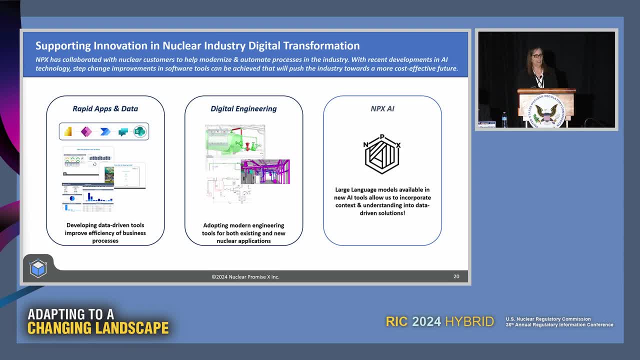 of apps and software. We do software and digital engineering. We have NPX AI, which helps to even you know engineering processes that are very data-centric. You know we can use AI in order to make those processes more intelligible and faster and efficient for people. 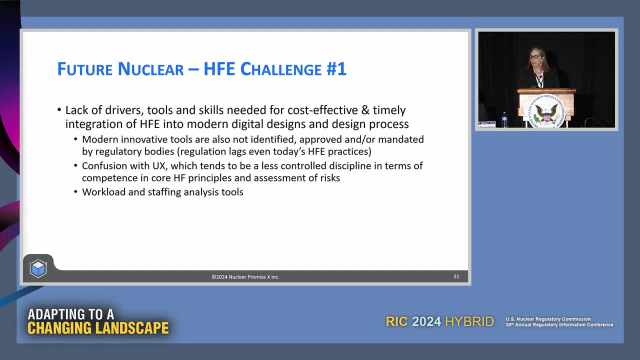 So down to the meat of the matter, HF- and I want to preface this by saying that these are both challenges. I've put them as challenges. They're challenges and opportunities. They really are, You know. yes, they're challenges because we haven't traditionally looked at these areas. 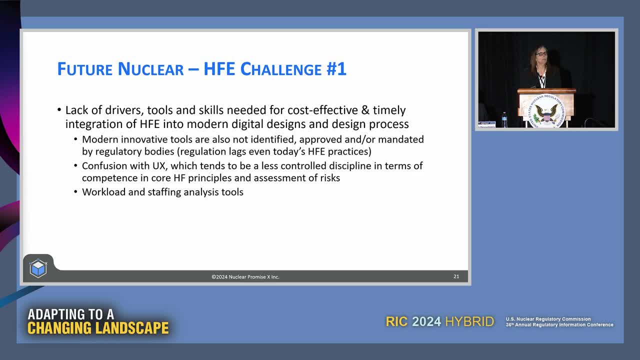 but they're opportunities because we can now focus on these areas. We have to focus on these areas If our new builds are going to be run safely by the people who are running, you know, these plants, then we've got to consider these things, And the first one is: 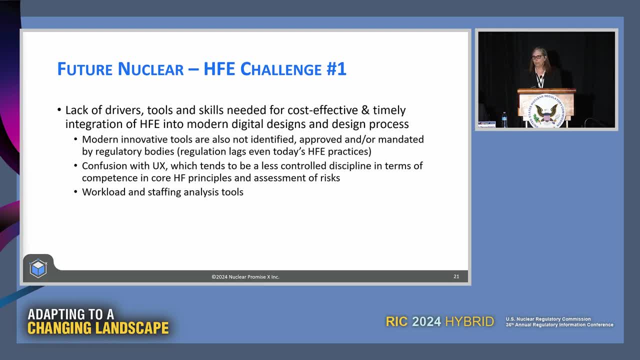 at this point there's a lack of drivers, tools and skills needed for not just doing HFE in the modern digital design world, But integrating effectively, integrating early. We have struggled with that as a profession from the very beginning. It's going to get even worse because it's going to go faster. 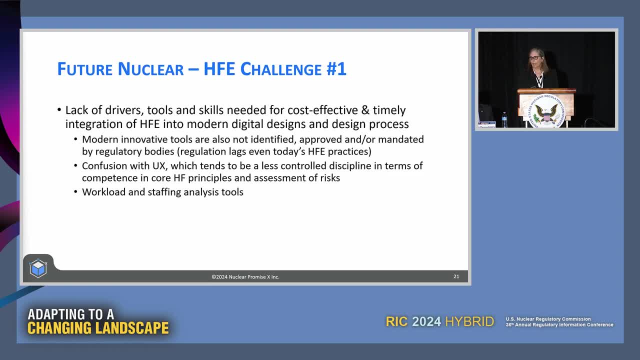 Decisions are going to be made up front that are going to have a huge impact. So, and I think that the tools we have as human factors practitioners aren't necessarily the tools we need. There are a lot more nuances in digital, you know, human AI teaming, human robotics. 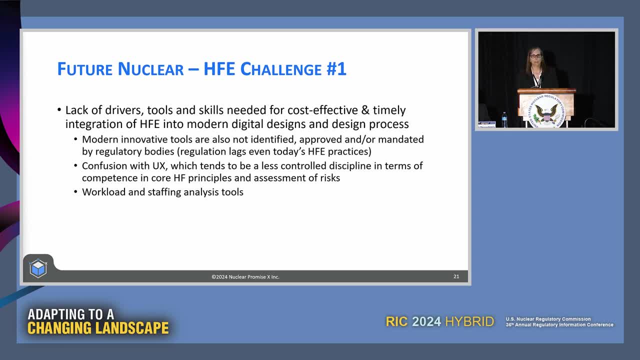 teaming and just even just digital interfaces. The traditional, you know, the traditional rules of human factors just can't be applied And the analysis we do is different too. Workload and staffing is a whole different ballgame when you're talking about highly 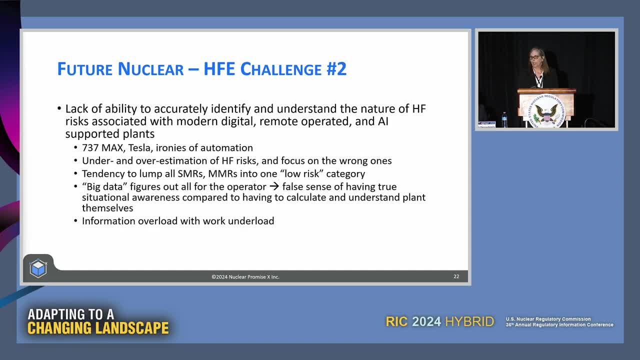 digital plants, The challenge number two, along with the tools and the skills which we're missing or that we need to get better at. I don't think we have given enough thought. Generally, people tend not to really understand or be able to quantify or discuss human factors, And so 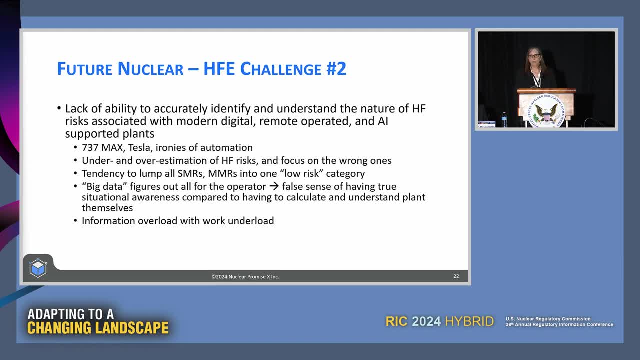 I think that's going to be a big challenge, And I think that's going to be a big challenge for us as human factors practitioners, especially future. We're pretty good at it in human factors practitioners, although even then, not across the board. I think that's just going to be. 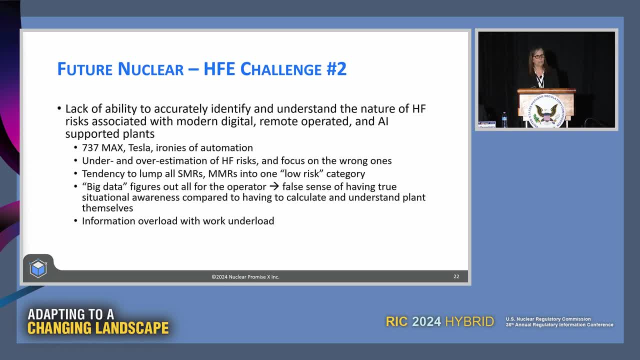 a whole other set of risks, different risks. They don't. they're not removed by removing some of the human in the loop. They're just moved to other places in the loop. We always talk about that. You don't get rid of the human, They're just somewhere else, And so 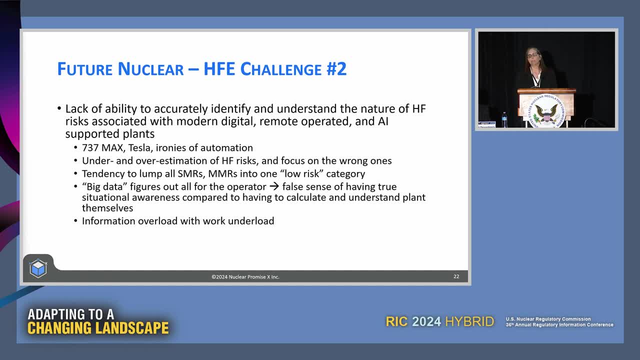 I think understanding the nature of the risk is going to be important for where we focus our human factors, expertise and effort. Because, number three- and there's some more things on the slide- some specific examples of where we've underestimated the risks And I think there is a tendency we're going to 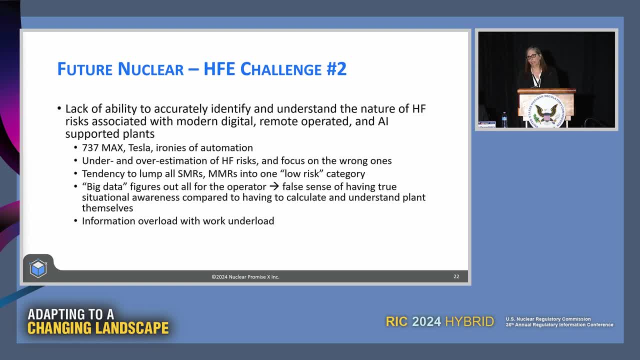 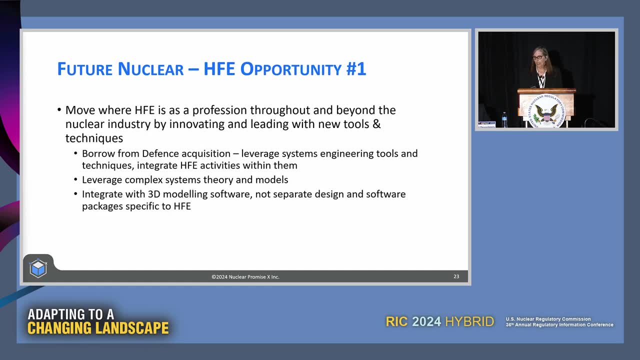 overestimate in some areas of traditional HFE. We're going to underestimate in a lot of areas. And then I think the third one is- and I had something on here too- about the people that we have and having enough people, And you know, move where HFE is a profession and start to use some of the tools and the 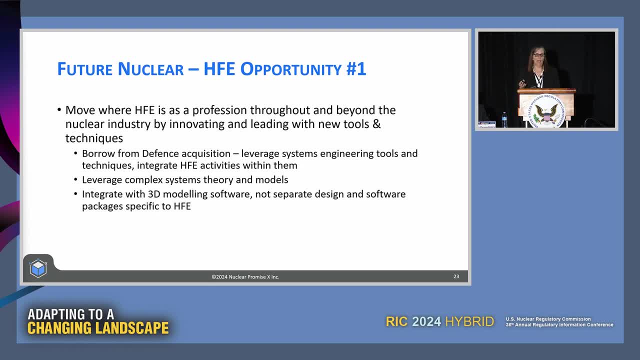 digital aids that we have that we're putting into the plants. We need to start using them within not only the people doing HFE in the design and new build, but within the regulators. You know we need to start using these digital tools but then also understanding the effect. 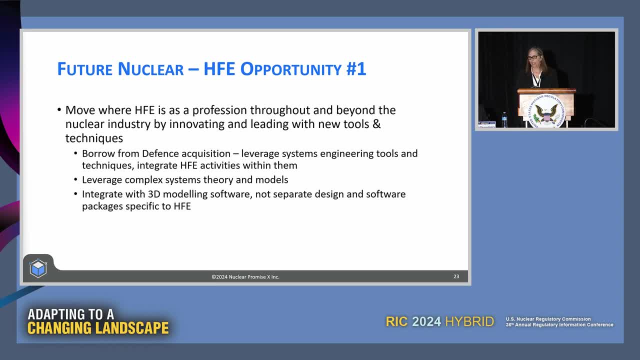 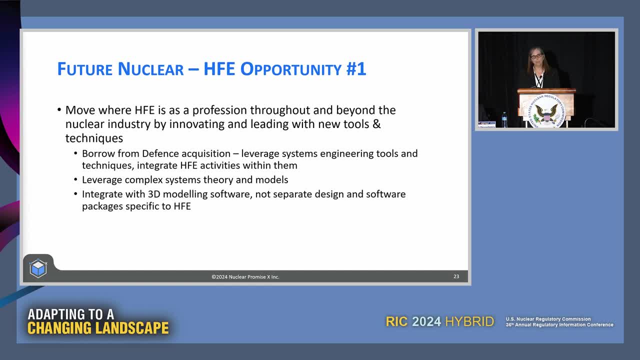 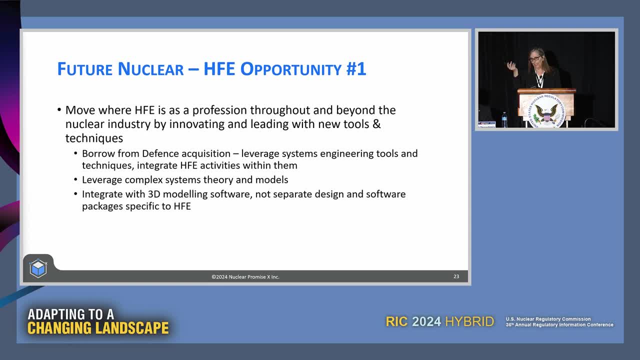 So that's my other thing. I think that the one I didn't really touch on, which was part of the second slide, which I'd like to say, it's the rate of change. that's the issue I know that all the regulators are looking at. yes, we have to modernize, we have to. 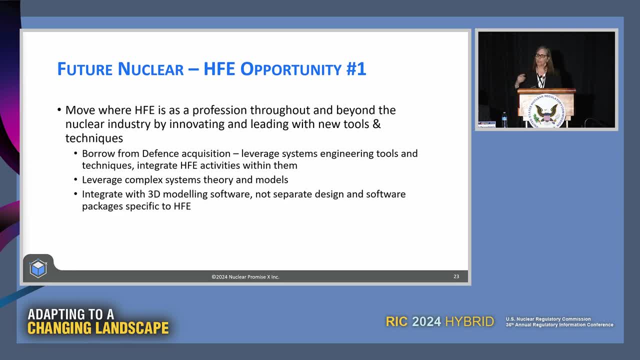 look at human factors differently. there's going to be AI, But that's only going to get quicker and I don't think we're responsive and quickly enough right now. So we need to start using digital tools to be able to pivot quicker. 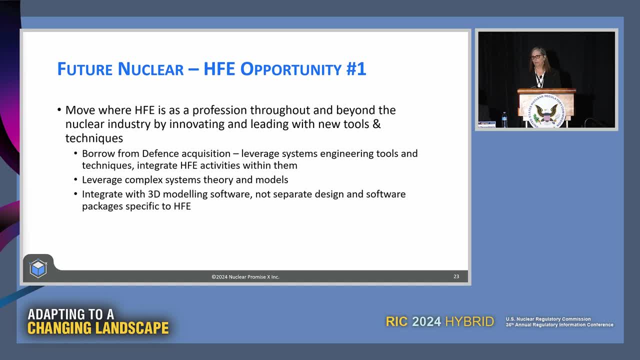 and be more agile in how we do human factors in the industry, And that's it That I do for time. Thank you, Six minutes, Okay, and if I didn't make it to the end of the session, I'd like to thank you all. 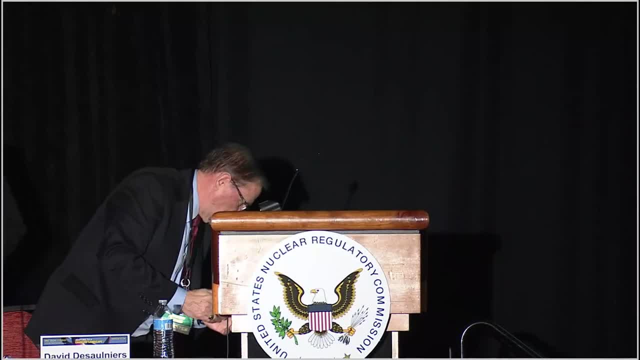 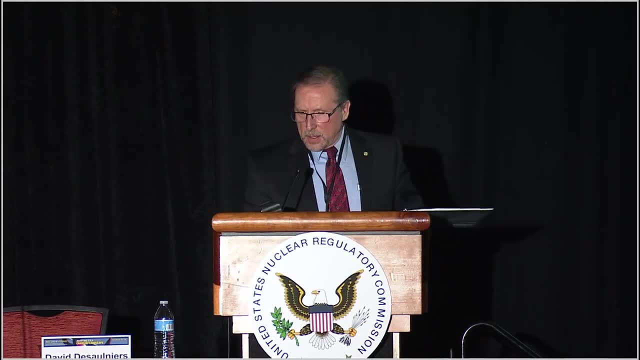 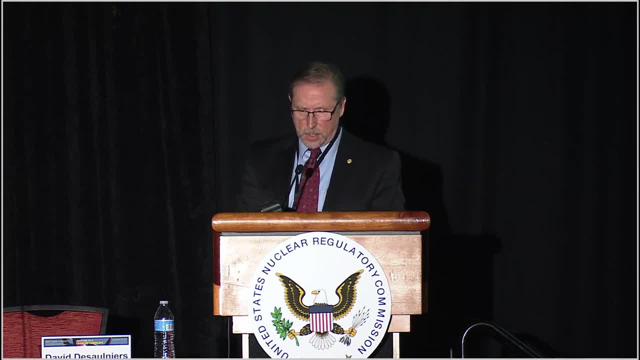 And I'll make clear up front- I don't remember what I said two minutes ago now We'll take questions at the end of all the panelists speaking. Our next speaker is Rick Pace. Rick has 13 years of nuclear experience and 3 years of human space flight operations experience. 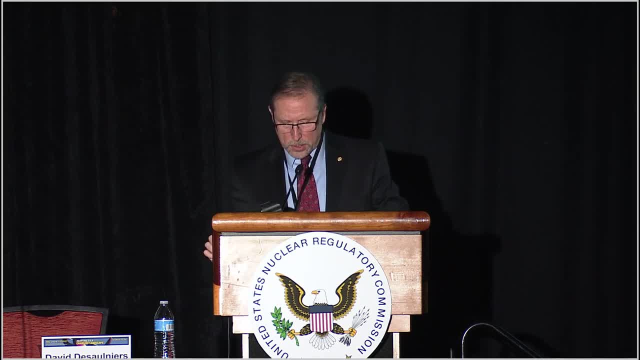 Rick is currently the lead human factors engineering consultant within the Sargent & Lundy Digital Modernization and Consulting Group. In this role, Rick is setting industry to start technical and regulatory precedents, working with multiple utilities on all current major control room design modernization projects. 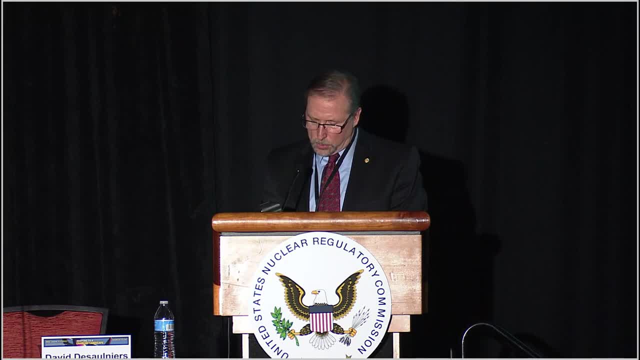 Prior to Sergeant Lundy, Rick was the lead Instrumentation and Control Human Factors Licensing Engineer for the Westinghouse AP1000, and the overall technical licensing lead for the Westinghouse EVINCI microreactor project. Rick is a member of the Institute of Electrical 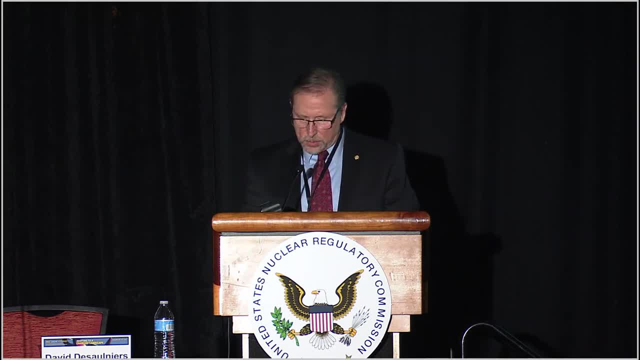 and Electronics Engineers, Working Group 5.2 on Human Factors Engineering and the Nuclear Energy Institute's Digital Instrumentation Control Regulatory Task Force. He holds a Bachelor of Science degree in Aerospace Engineering and a Masters of Science degree in Physics. Please welcome Rick Pace. 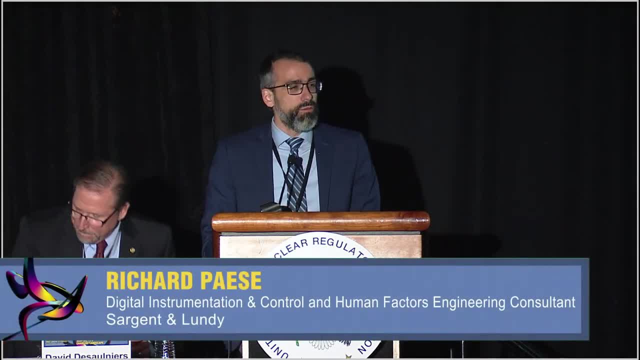 Thank you for having me. It's an honor to be here today. So today we are talking about the changing roles of humans in new and advanced reactor designs, And so we're asked to answer the question: what's the biggest challenge in this? 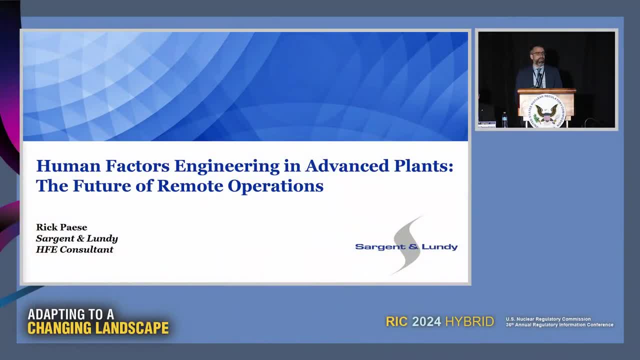 And I think there are many, but if I could name one, I think one of the biggest challenges, also being one of our biggest opportunities, is the increase use of automation within our systems, within our plants. Because as we increase the use of automation in our plants, 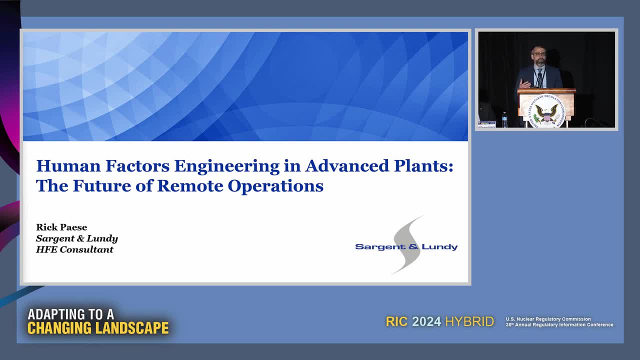 this obviously is going to have a direct impact on how the human and how the operator interfaces with this automation and interfaces with the system. And, as I pondered this question, it's not that some automation and using automation is new, it's just the increased level of our ability. now, 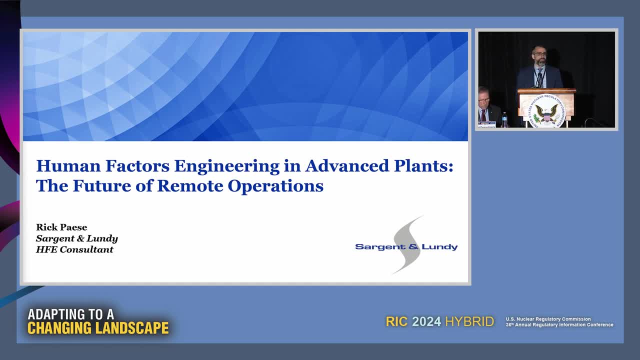 with new technology to leverage this automation to its fullest and to a greater extent, And so that's what I'm going to talk about today, and so I'm going to use my time here just to give a few thoughts on things that we need to consider as an industry. 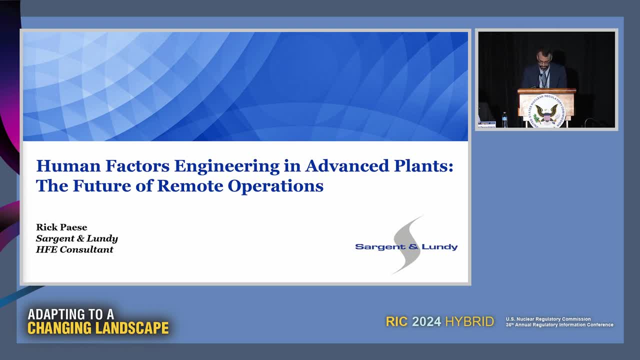 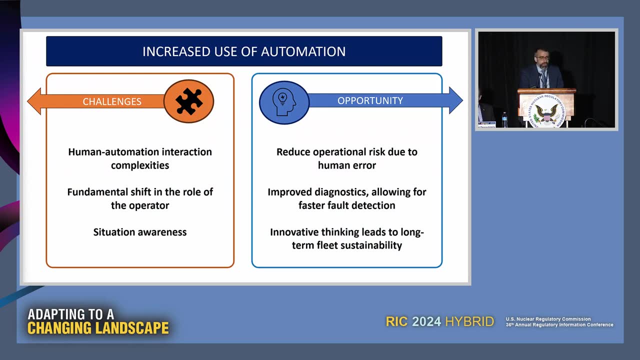 as we move forward to increasing automation, as we look forward to the future. So the first thing I'll say for the increased use of automation is the opportunity to improve the safety of our plants. So you know, one of the biggest contributors to system and plant errors are human errors. 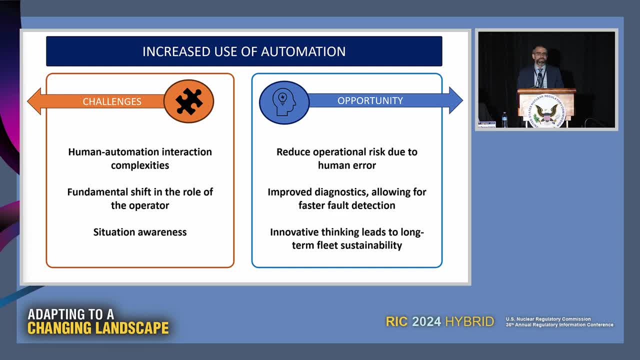 And that's understandable. Humans are fallible and we make mistakes, And so if you can minimize the amount of times that a human or an operator touches the system, you can theoretically minimize the amount of errors that get introduced. And so, as we rely upon automation, 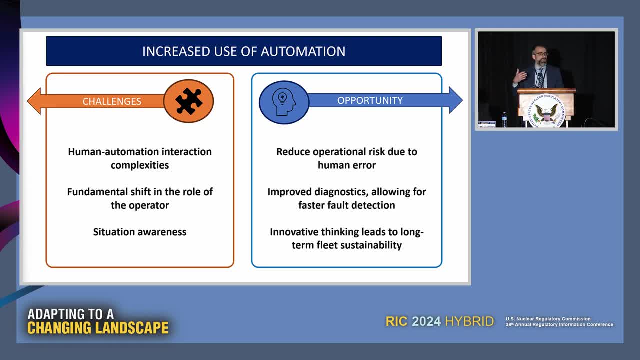 we can reduce the amount of times that the operator or the human needs to interface with the system, And so that could be a positive in plant safety. Thank you. Now, on the other side, the more and more automation that we use could introduce more and more complex systems, which 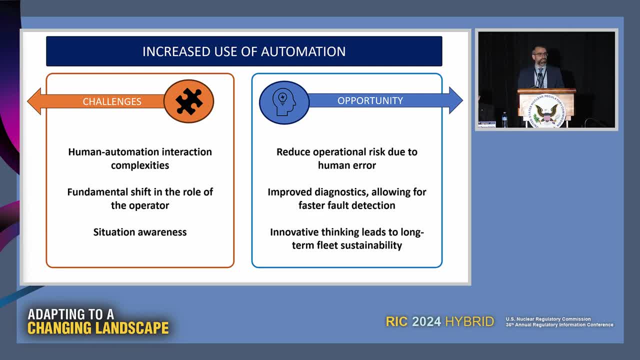 in itself could also introduce system errors right, And so there's a balance that we have to make, in my opinion, on using the right level of automation for a given system, And that's an important point I think that I would like to stress is automation. 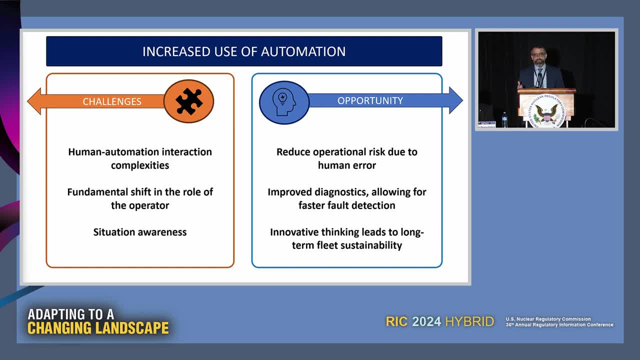 isn't an either-or thing, right? So it's not: either you're using it or you're not using it. There's gradations of the amount of automation that we could use in our plant, So at the extreme end, you could think. 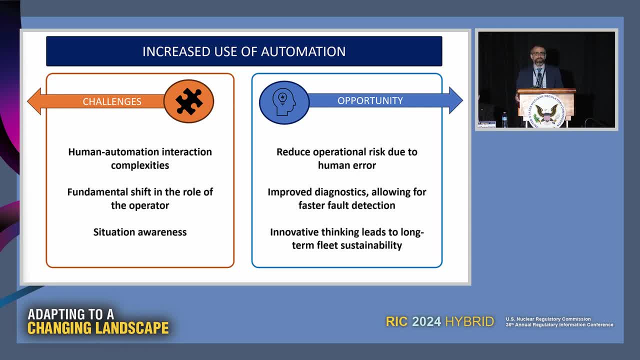 of an automation level of one being fully manual and the operator does everything that the system in the plant needs, or an automation level of 10, say, where the system does everything and completely ignores the human in the loop. Now, in reality, we're somewhere in between that. 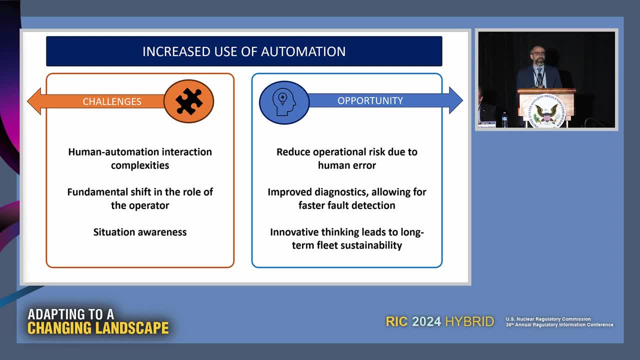 So you can consider or think of varying degrees of automation within those two extremes, such as automation with operator supervision or operator consent. Or maybe the system performs its automation and it decides when the human should be in the loop and when the human needs to be informed of something. 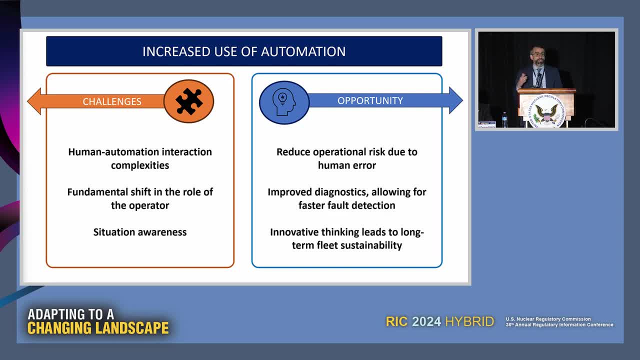 or the human needs to take action, And so you can sit here and think through, and others have the different levels of automation. I think the point here that I want to make is that as we leverage this tool, we need to think of what makes sense for the given situation. 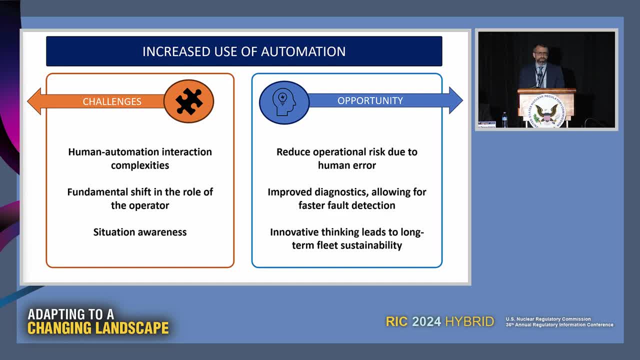 and apply that and understand the impacts, Because, ultimately, at the end of the day, no matter how much automation we do, we're going to be able to do a lot of things. So I think that's one of the things that we need to do. 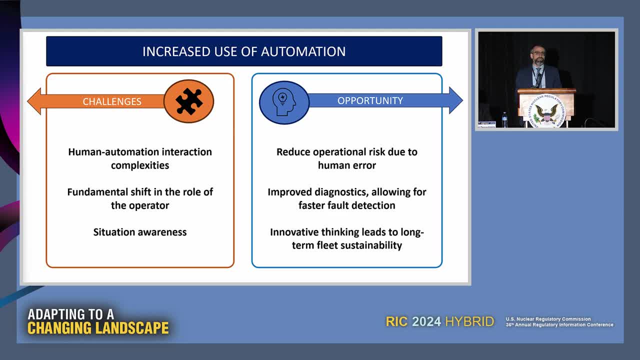 So I think that's one of the things that we need to do. I think that's one of the things that we need to do And so, ultimately, if automation we use and leverage, the operator still needs to be aware of what the system is doing. 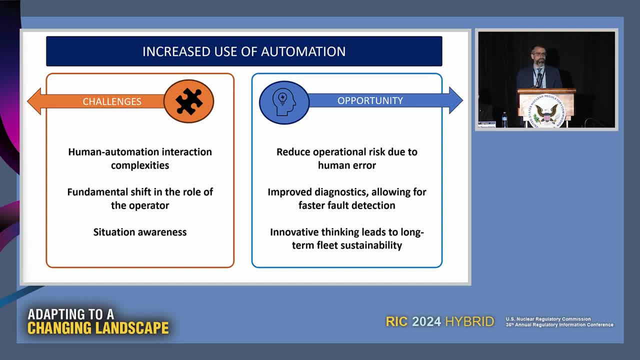 They need to be knowledgeable of the system. Their situation awareness is one of the challenges that we have to overcome with this, Because, as the system is performing tasks in the background, we always have to make sure that the operator understands what's happening with the plant. 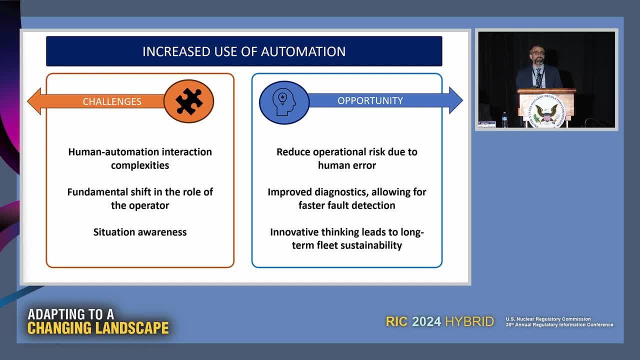 They need to be able to troubleshoot any failures And, ultimately, if automation fails, they need to be trained in such a way where they can take the appropriate action to keep the plant in a safe state, And so That's another sort of sub-theme that I'd like to point out. 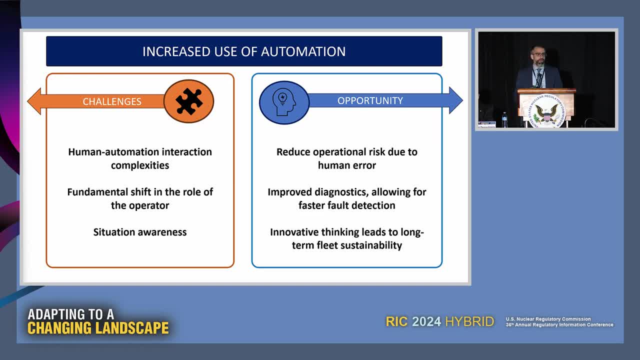 is. training is an important piece to this. The rules of the operator are going to change as we use more automation, which means that their training and their understanding of the systems are going to have to keep up with that. The last thing I'll mention here is a very positive thing. 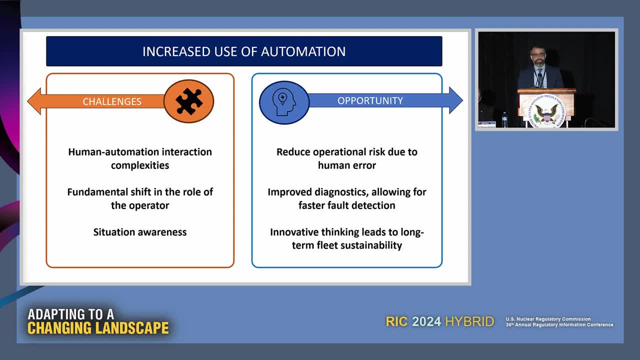 for automation is improved fault detection, So self-diagnostics in these systems can continuously monitor the system and ensure that there are no faults, And Dave had mentioned it earlier in his speech. But the system can do this more effectively besides relying solely on human intervention right. 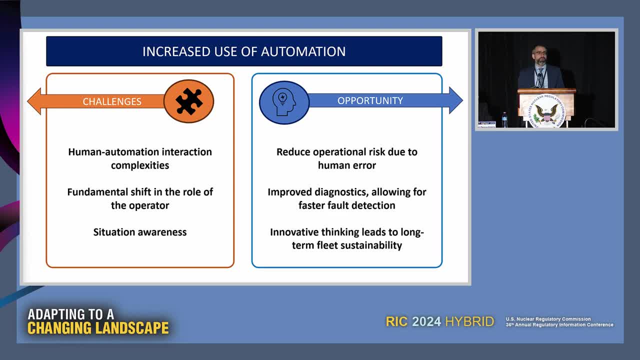 The system can sometimes see things that the operator can't see, even before they become a problem to the plant, And so there's a ways to leverage this so we can have early fault detection, so that we can take action and keep the plant in a safe manner. 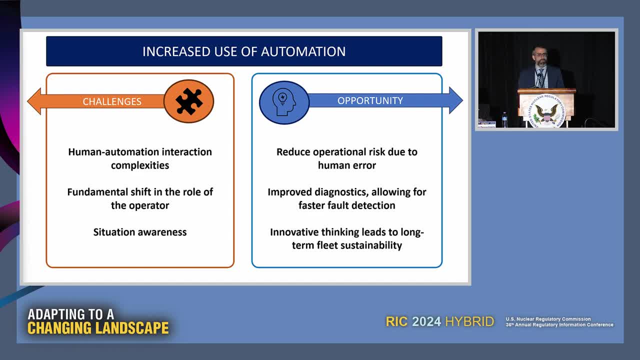 Again, the operator needs to be trained on these things and to be able to do that. We need to be able to troubleshoot and diagnose when these self-diagnostics aren't working, But we can leverage those for improved plant safety. So, ultimately, we need to think outside the box. 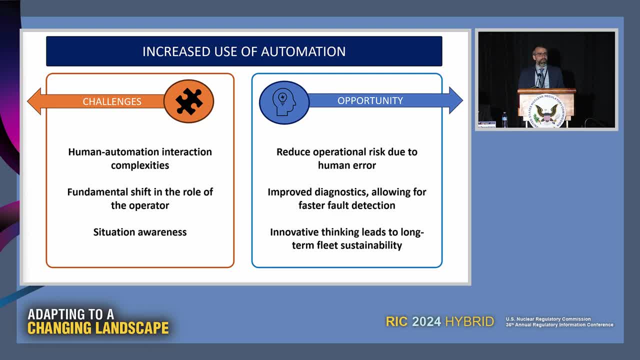 and leverage this technology. I've seen firsthand where we spend a bunch of effort and time modernizing our systems, yet we don't take full advantage of the benefits of the system that we install, And so self-diagnostics is one of those areas. 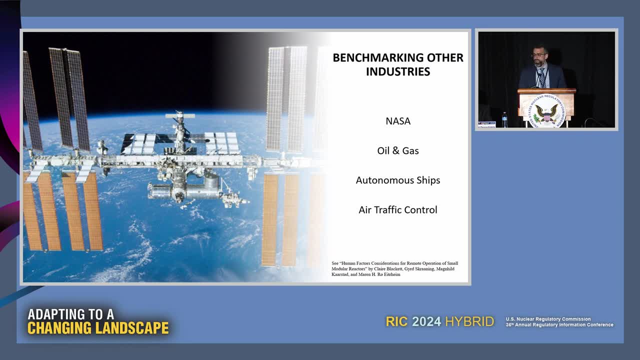 And I'll just end my talk here- Encourage us as an industry To look forward to other industries, Because other industries are leveraging automation to a fuller extent than we are And they're designing these remote operating systems already, And I know that that's the direction that some of us 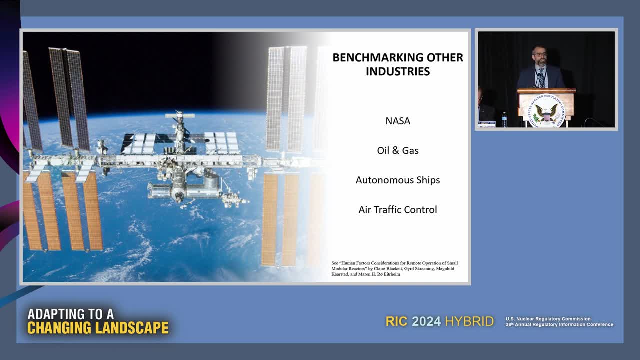 are going to in the human factors world is remote operations, And so I think that's important for us to leverage those lessons learned. Dave had mentioned that I did have some time and experience as an operator for the International Space Station And this was sort of an opportunity. 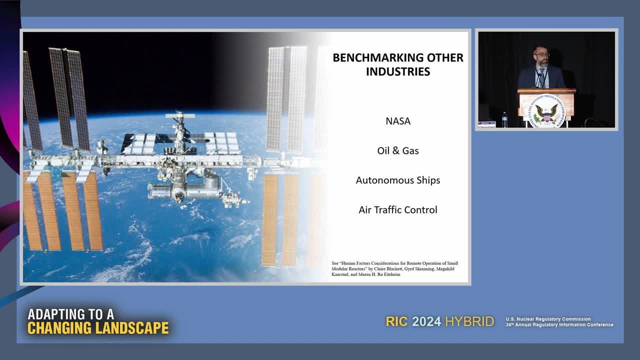 And I think that's sort of an ultimate in remote operations And that we have astronauts orbiting space in a space station And most of the command and control and monitoring is happening on the ground level And, frankly, the safety priority is the same thing. 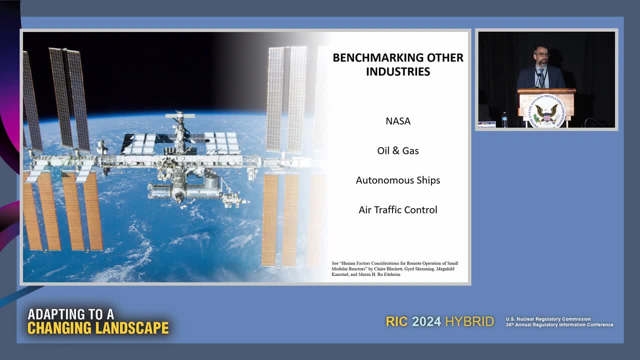 And we have as humans and people we're our number one priority in their safety. And so it's not just NASA, It's oil and gas, autonomous ships, air traffic control, I mean there's all kind of work going on in this. 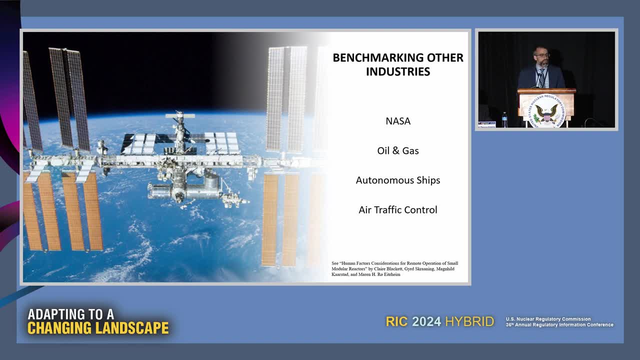 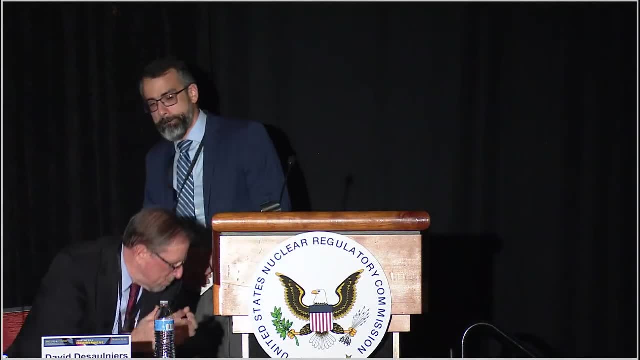 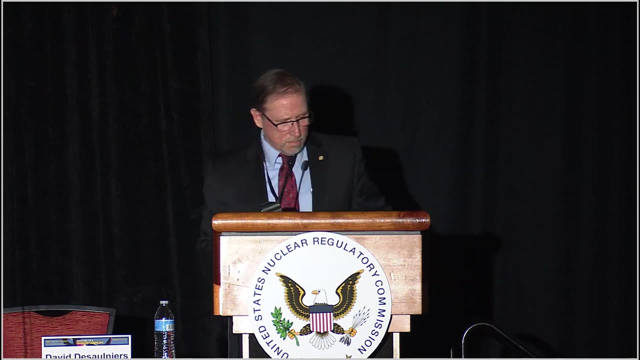 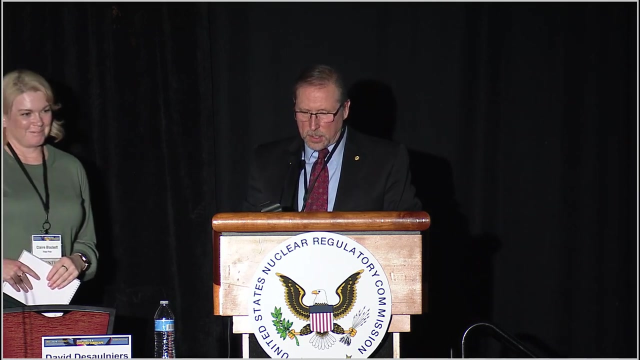 In this area that we should be leveraging as an organization. So thank you for your time And I look forward to the panel discussion. Thank you, Rick. Our next speaker is Dr Claire Blackett. She is a senior human factors consultant at Risk Pilot. 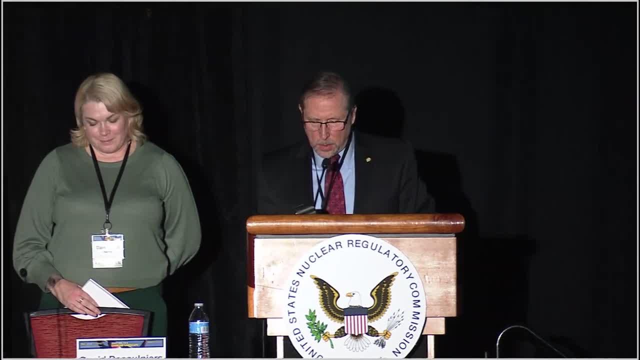 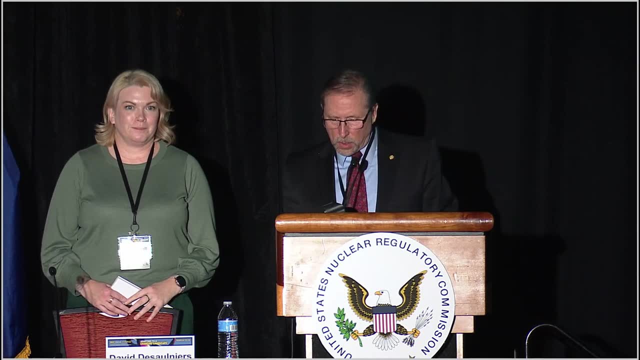 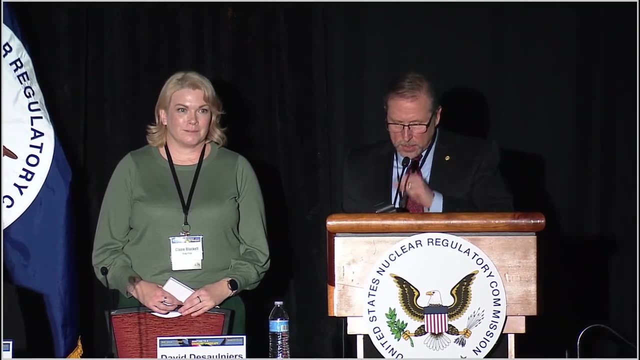 in Sweden. Claire has almost 20 years experience working as a human factors specialist in both research and industry, including 11 years as a principal scientist with the Halden Reactor Project in Norway. Claire has a background in root cause analysis for accident investigation with a PhD in this topic. 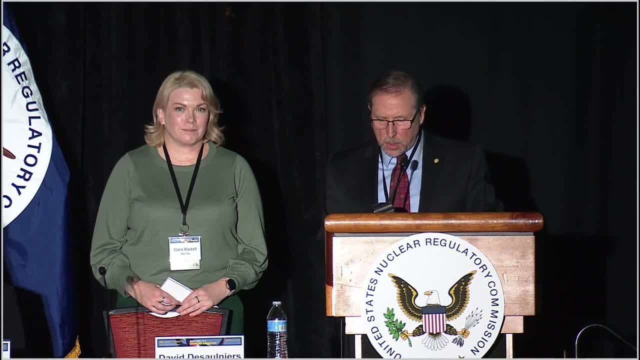 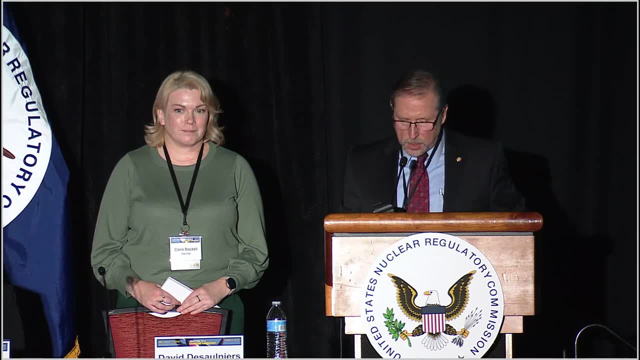 She has worked primarily in the nuclear industry throughout her career, providing human factors and human reliability analysis support to nuclear safety cases, as well as conducting human factors engineering assessments and providing input to event investigations at commercial nuclear sites. Dr Blackett also has experience from the petroleum maritime. 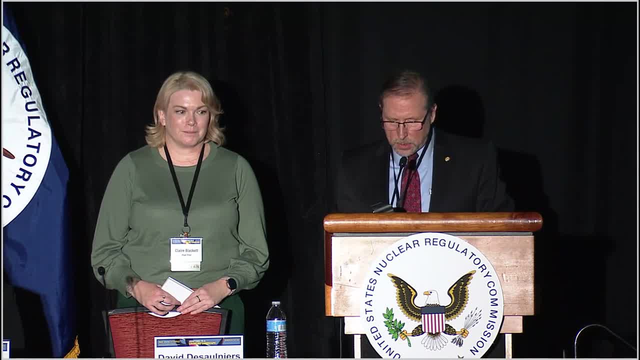 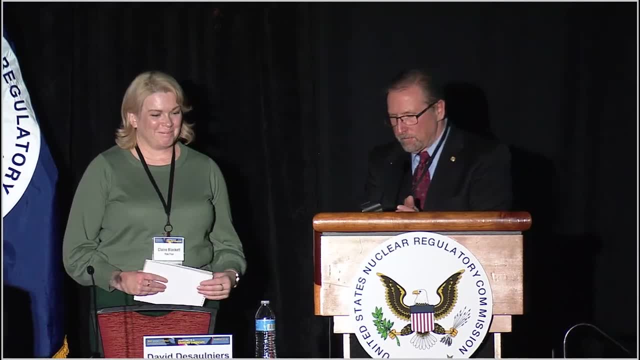 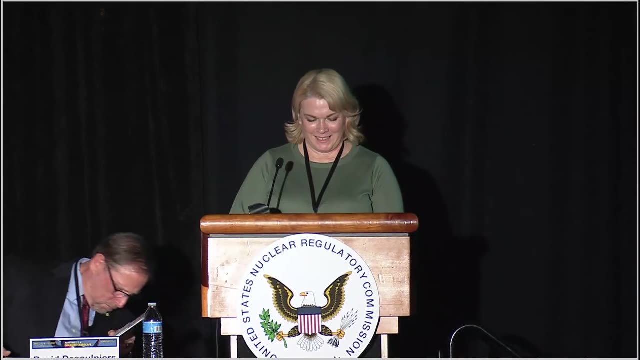 rail, health care and process industries and continues to work in all of these domains today. Please welcome Claire Blackett. Thanks, Dave, And thank you everybody. Thank you for joining us today. Just to mention, Risk Pilot, since I'm 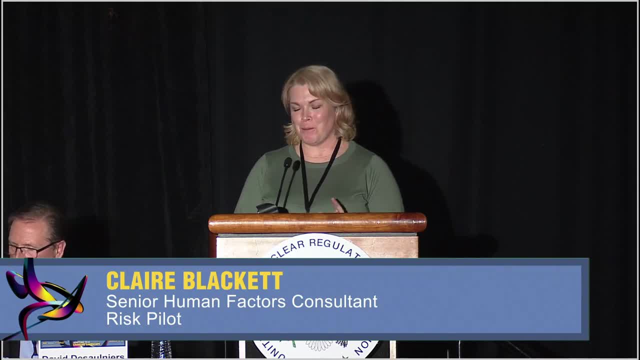 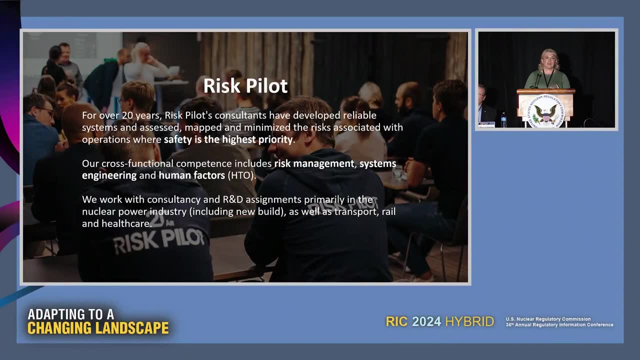 sure that most of you have probably heard of the Halden Reactor Project, so you know about that. but since December I have moved into a new role with Risk Pilot, based in Sweden, And Risk Pilot- they've been going since 2002,. 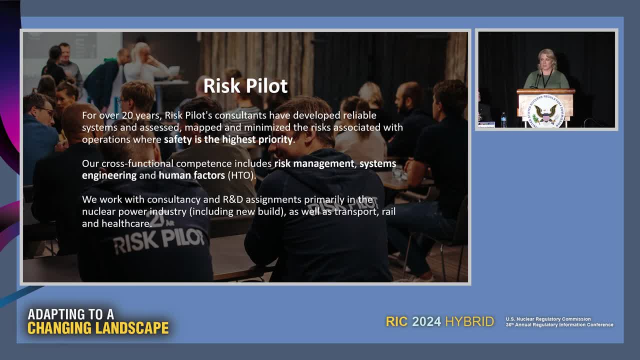 originally set up as a risk management consultancy but since then has expanded into including systems engineering and human factors, So I'm part of the human factors team there. There's nine of us. We have a very strong presence within the nuclear industry in Sweden at the three nuclear power plants. 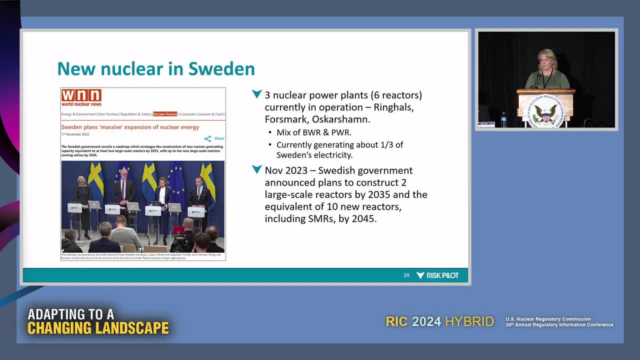 So we have most of us work on site at those plants, And nuclear in Sweden, you may or may not have heard, is going through a bit of a revolution. It's fantastic. In January this year, Sweden announced new plans for expanding the nuclear force. 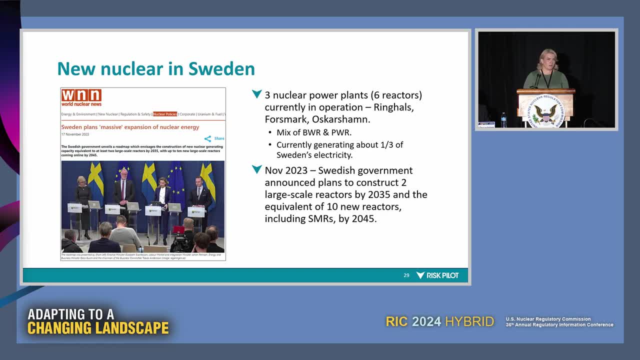 Now I moved to Sweden in December And they decided this in January. I'm not sure if it's because I moved there, but you can join the dots yourself. So in Sweden currently there are three nuclear power plants: Ringhals, Forsmark and Oskarshamn. 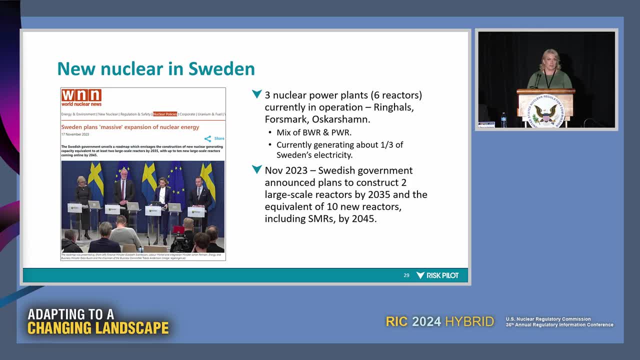 And they produce about a third of the electricity in Sweden, So they're extremely important to Sweden. But in January this year it was decided that they're going to build more, And so the plans are for building two large-scale reactors by 2035.. 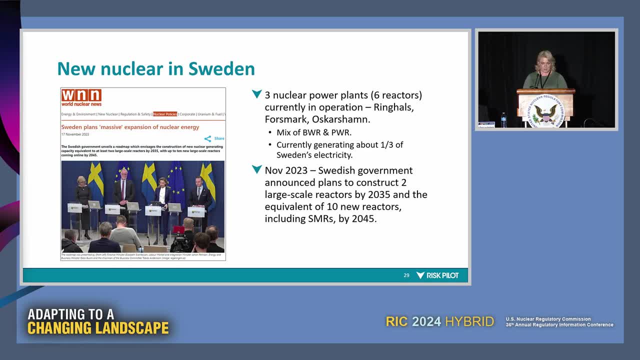 So the goal is to add an additional 2,500 megawatts by 2035, and the equivalent of 10 new reactors, or 10,000 megawatts, by 2045.. So it's a really ambitious goal, but they're very, very. 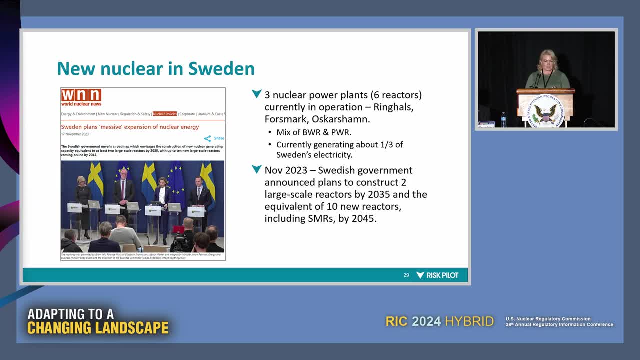 committed to actually doing this And essentially they're assuming an electricity demand of about 300 terawatts by 2045.. So they sort of acknowledge: oh, we're going to do this, We're going to manage that Between their renewables and the nuclear power. 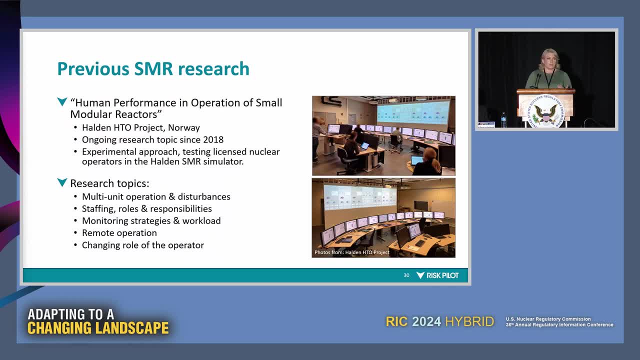 this is how they're going to achieve it. My previous work in the Halden project. towards the end of my career there, I started to focus a lot on small modular reactors And I was very fortunate to be able to work almost exclusively. 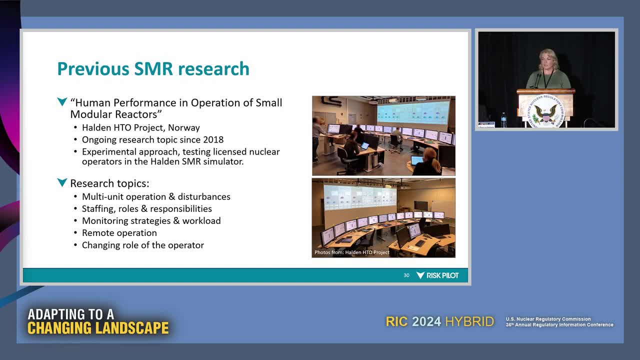 on this topic via the Halden Reactor Project, And that included being involved in the experimental program at the new Halden SMR simulator that was installed, And it was a project that was installed in 2021.. This reactor has the capability of simulating up to 12,. 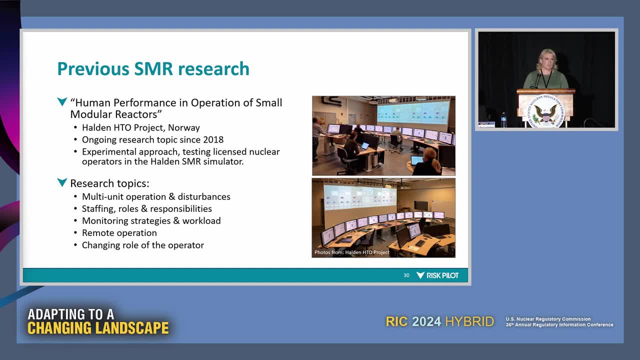 or a plant of up to 12 units. We had it set up as a six-unit plant And this enabled us to actually see how operators can run and monitor and control this plant- a six-unit plant. So we had run three experiments by the time. 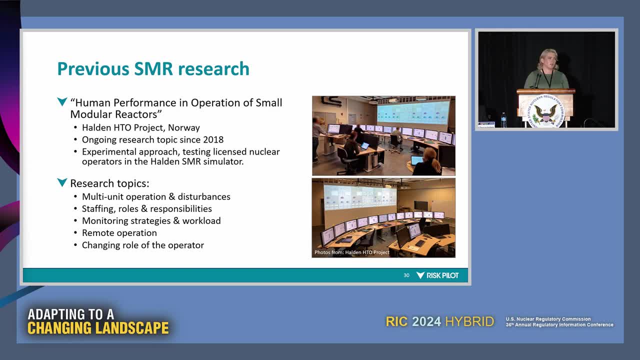 I finished my time at IFA Using Operator 2.2.2, and then we had an experiment with a new one, And we had a new experiment with a new one. We had a new experiment with operators from the US and from Sweden. 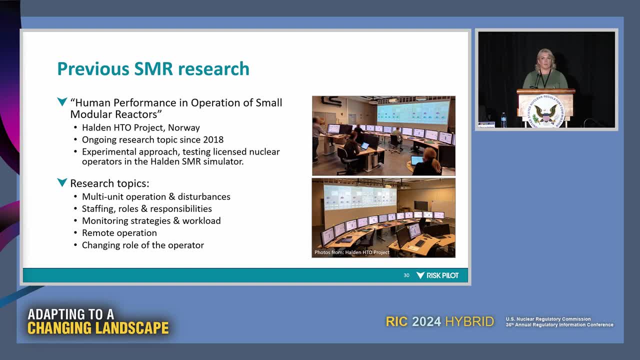 These are licensed operators currently practicing And none of them had operated in an SMR before, of course, because we don't have any commercial SMRs yet. But we put them in this situation and we ran them through different scenarios to see how does it look. 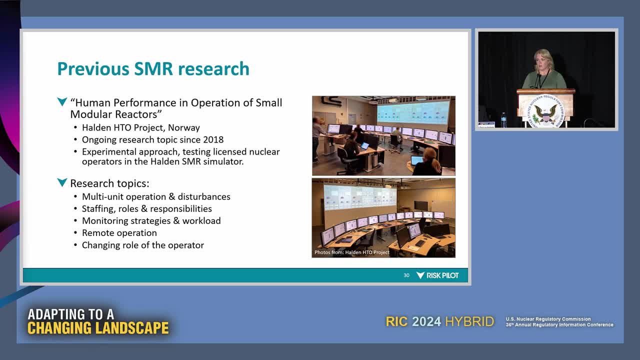 And the kind of topics that we were interested in was looking at multi-unit operation and disturbances, staffing, roles and responsibilities. how do operators monitor across a six-unit plant and how do they manage their workload? We also talked about- although we didn't do any experimental studies on remote 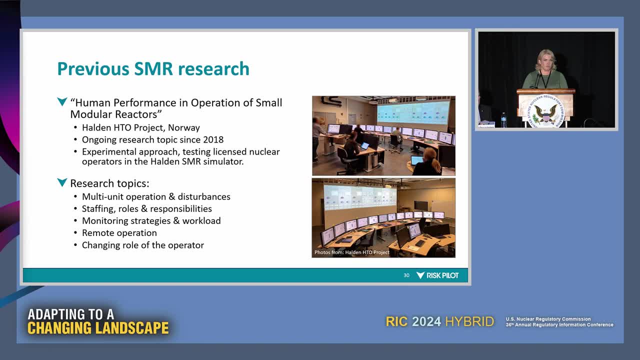 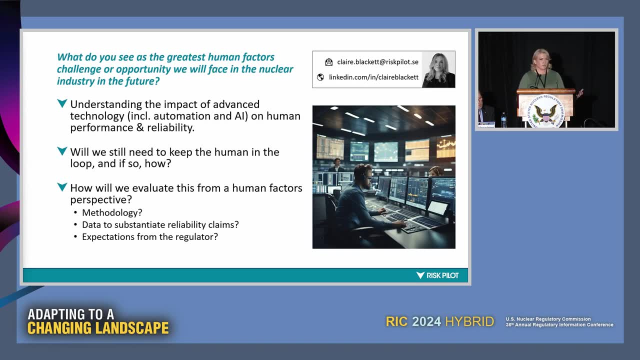 operation and very much looking at the changing role of the operator, so very relevant for this session today In terms of what I saw from the research that I have done before, and then also just thinking about where Human Factors is going, when I considered what is the greatest challenge or opportunity. again, 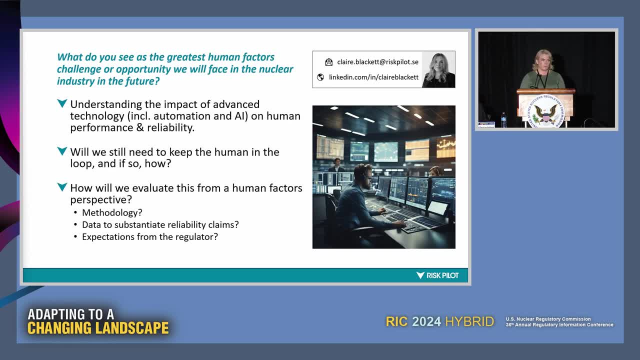 I landed on the topic of automation as being one of the main challenges. I think that when we talk about highly automated SMRs, we kind of don't really realize what we're talking about. Automation is not a single discrete thing. It's not. 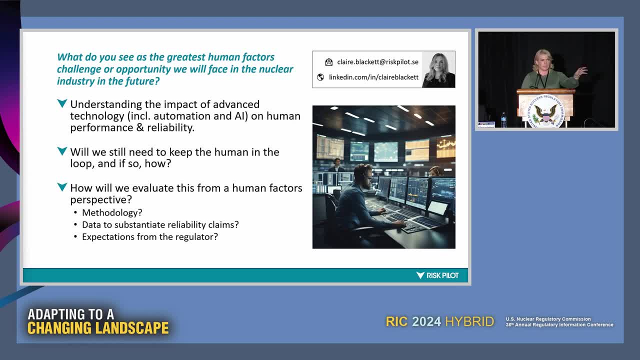 just another system component that you can plug in and then say, okay, now it's automated. what do we do? Automation is much more complex. It's much more likely that we are going to have layers of automation within our systems, and some parts of the plant may be more highly automated than other parts of the 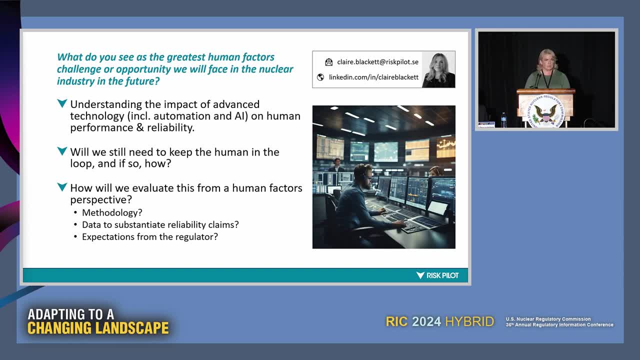 plant. So we really have to think about the complexities of automation. where and how and why have systems been automated and then need to understand and how is the human going to interact with that? We also have to think about: is this going? 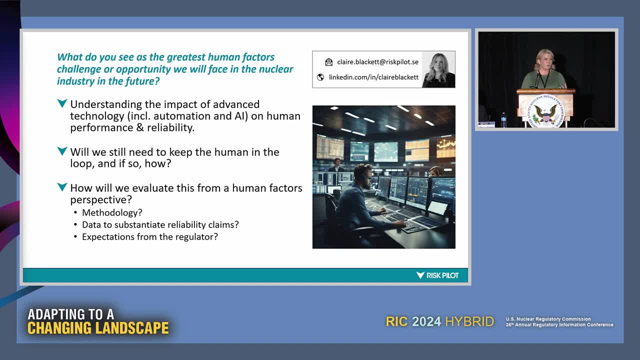 to create new types of human errors, errors that we don't see in our existing plants, And then how are we going to be able to assess those from a Human Factors perspective, from a human reliability aspect? And then, touching a little bit on what Karen said as well, is also thinking about, 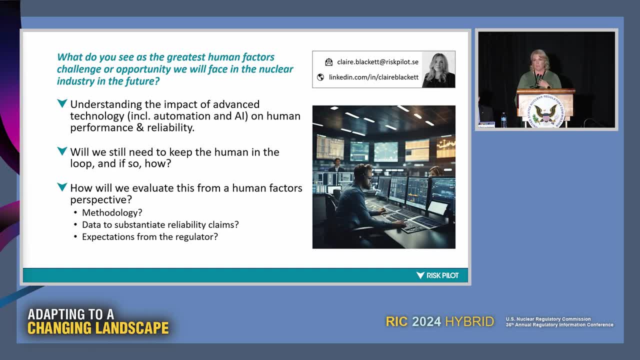 the methodological side of it, then How do we as Human Factors professionals approach these potential new errors that are going to occur? I agree with what Karen said about we need to be kind of quicker in how we do our Human Factors assessments. When we look 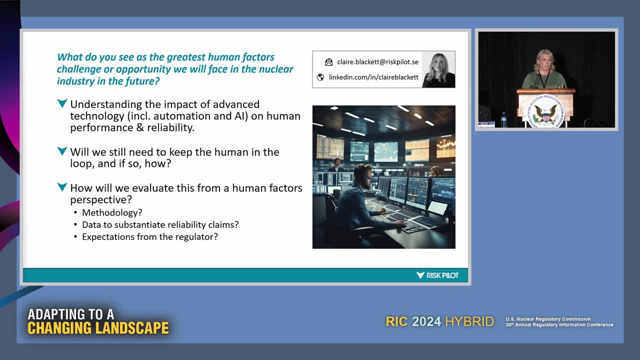 at the world of SMRs, for example, we see that there are so many vendors out there. This world is evolving so quickly. We, as Human Factors professionals, need to be able to keep up with that pace. So I think that the methodology, the approach, 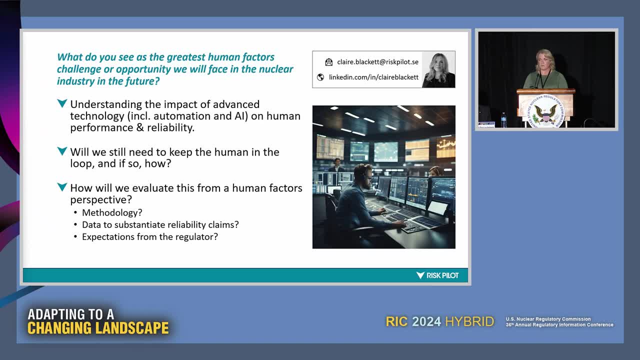 that we use for Human Factors is also going to be a challenge for us going forward. As always when we talk about Human Factors, we never have enough data. So how do we generate enough data to be able to validate designs and substantiate claims that we are making? 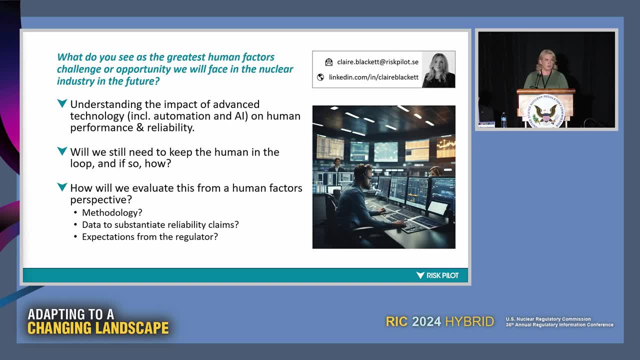 on operators And then also what will be expected by the regulator is another big question. that at least I've gotten a couple of answers on that from this this week. So in my opinion, those are the challenges that we will face. Thank you very much. 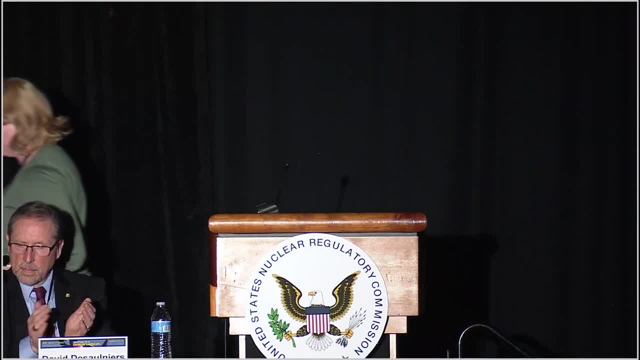 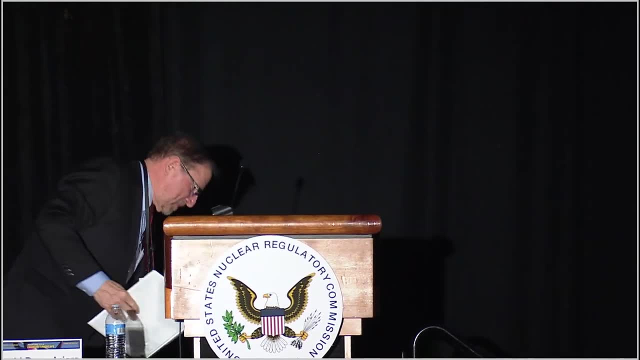 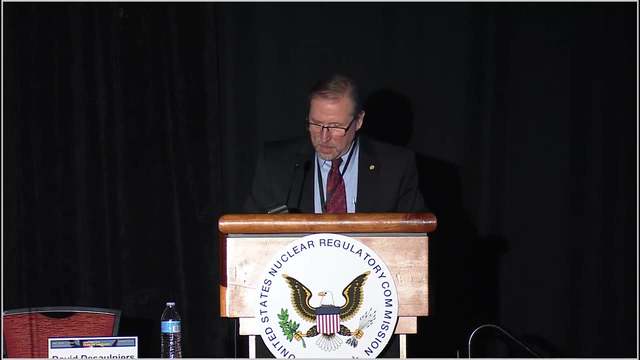 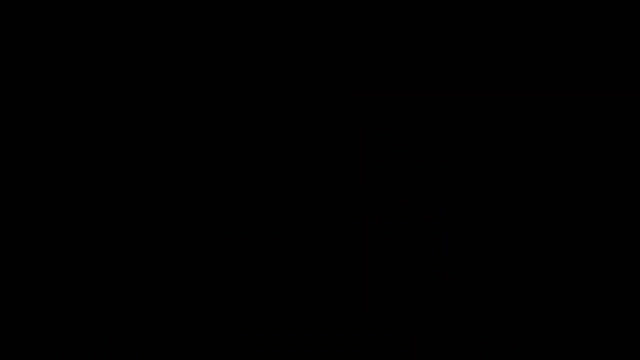 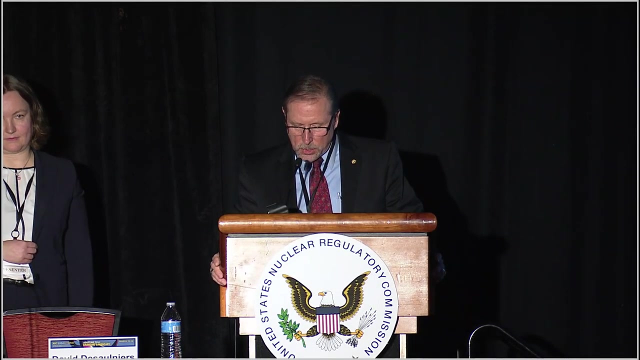 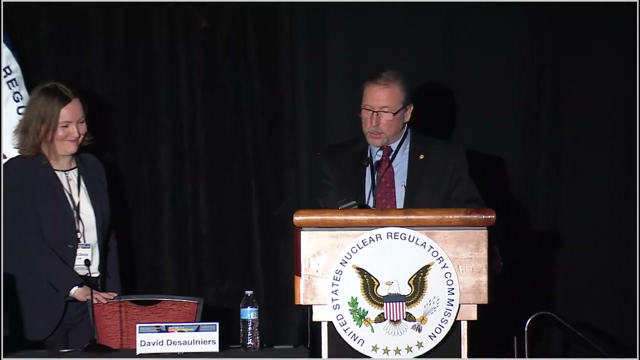 Okay, our next panelist, Dr Paola Savioia, is the head of the Operational Safety Section in the Department of Reactor Regulation at the Radiation and Nuclear Safety Authority of Finland. I have to say Paola challenged me with this introduction. 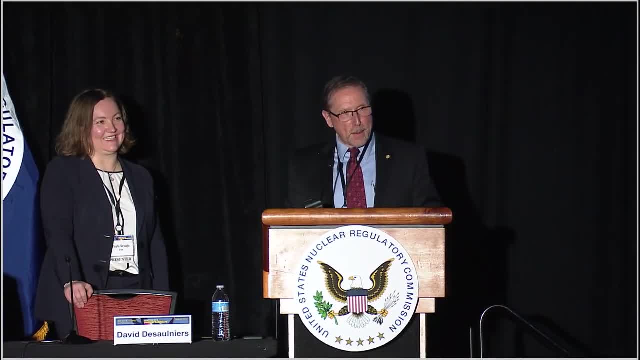 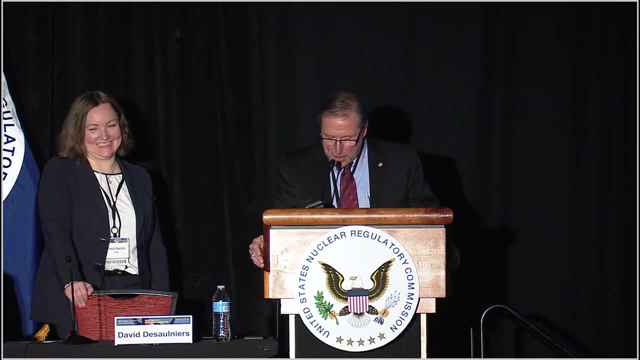 because it's got the combination of the longest institute names I think I've seen. So if I pause in the wrong spot, please forgive me here with this. From 2001 to 2016,, she was a research scientist and team leader for the Human Factors and Complex Systems team at 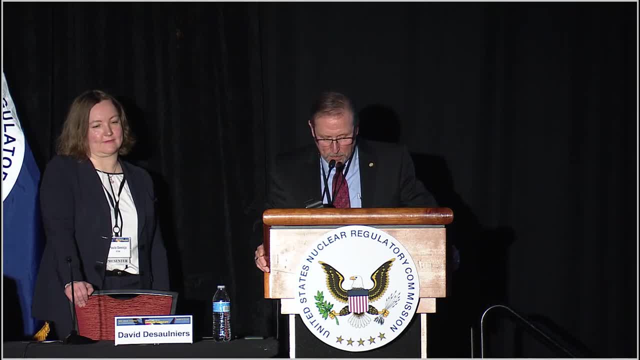 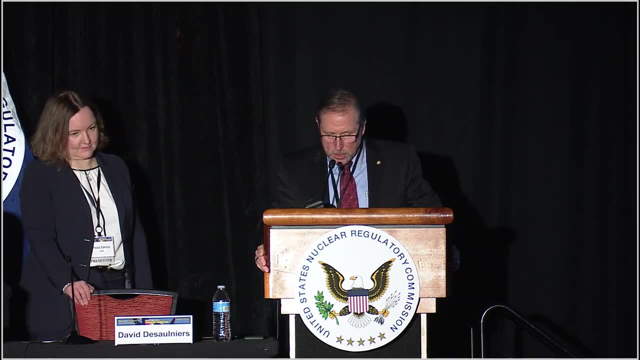 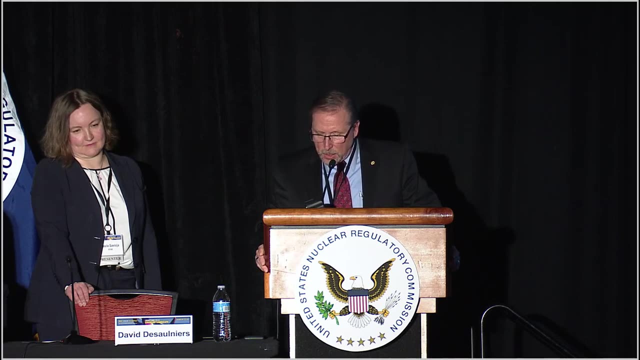 the VTT Technical Research Center of Finland. While at VTT, Dr Savioia obtained a master's degree in engineering from the Department of Automation and Systems Technology of Helsinki University of Technology in 2003.. In 2014,, she completed her doctoral studies with distinction. 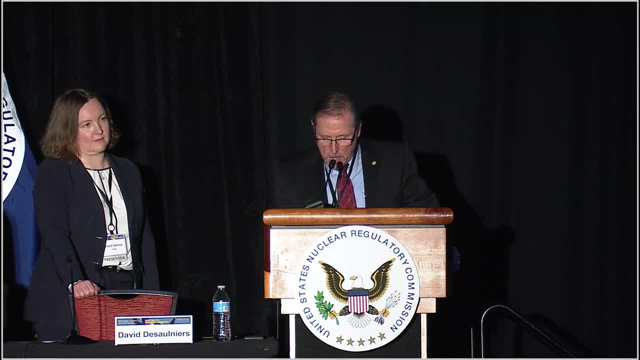 at Aalto University School of Science. In her dissertation she developed a systemic usability concept and evaluation methods to help the deployment of user-centered design approaches within complex socio-technical systems. She has expertise from several industrial domains, including nuclear power, maritime. 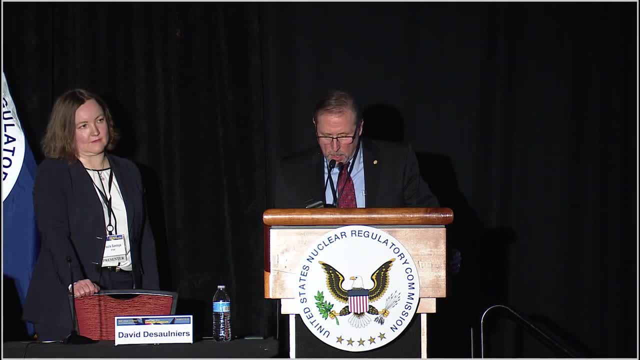 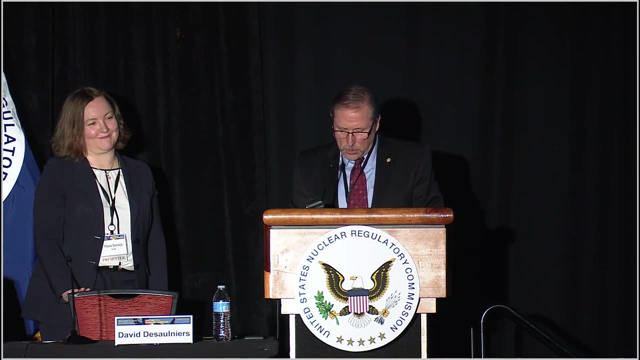 metals and machines, process control and fire and rescue services. In her current work at STUC, she is taking part in the nuclear energy legislation renewal from the perspective of operational safety. The legislation renewal is part of Finland's preparatory works for the licensing of advanced reactors. Please welcome Dr Savioia. 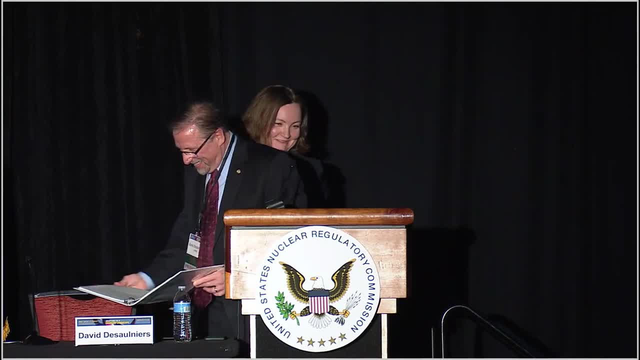 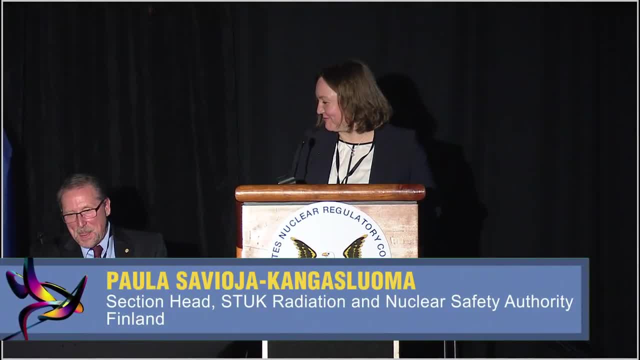 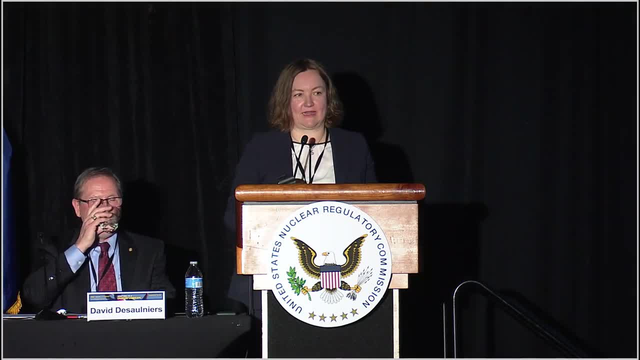 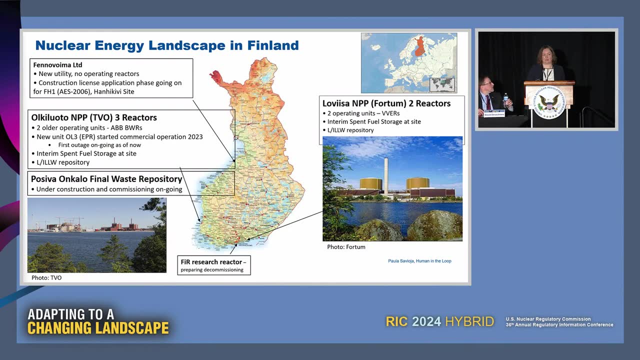 I come from STUK, the regulator of radiation and nuclear safety in Finland. Just to give you a little bit of context for what I'm going to talk about, I will very briefly say something about the nuclear landscape in Finland. We have five operating commercial reactors as of now. 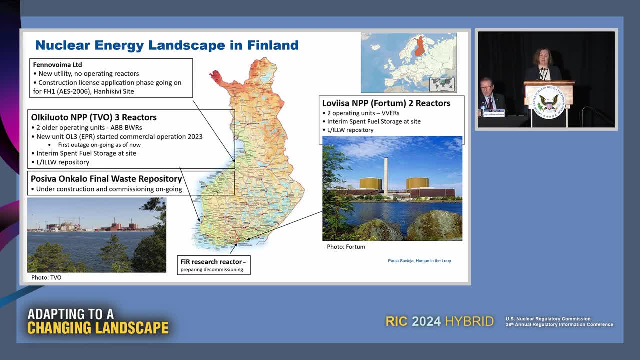 Four are a little bit older ones, dating from the late 70s and early 80s. But all those older plants, they have gone through some sort of automation, renewal and digitalization. So the control rooms in even our older plants are so-called hybrid ones. 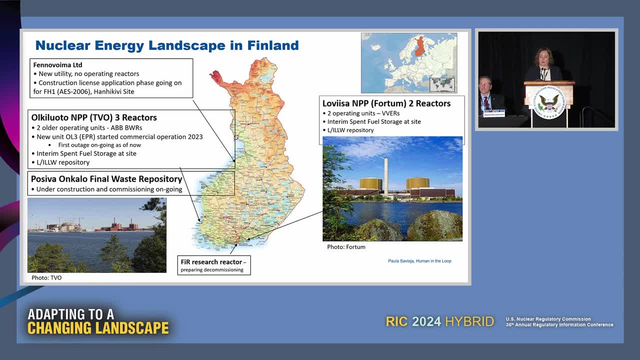 containing digital systems and analog systems. But most important experience, My experience for myself- is our new unit, OL3,, which has been in commercial operation for about a year now And it's actually going through its first yearly outage now as we speak. 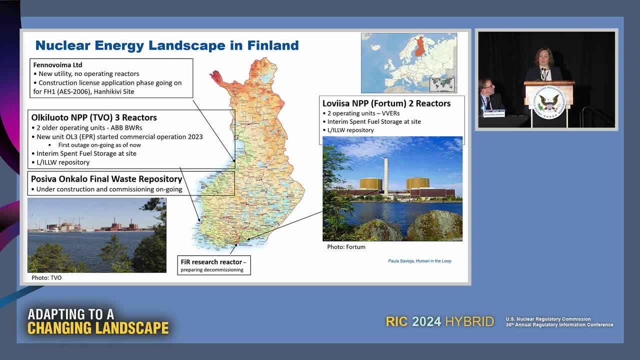 And OL3 is quite a highly automated plant. It's an EPR 1600 megawatts and it's located in western Finland. Then also, we have had One thing I want to point out from this nuclear landscape is that when we have been working in Stuk, we have had nuclear facilities in all life cycle phases. 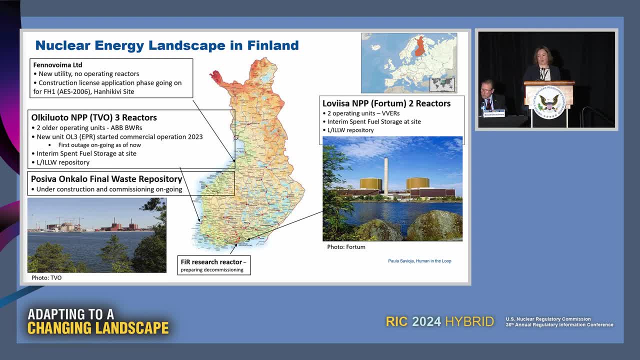 Because we have the operating plants, the new unit. We also had a construction license review ongoing for a while for a totally new plant, And then we also have a final repository project that is in construction and commissioning right now And construction license application was withdrawn. 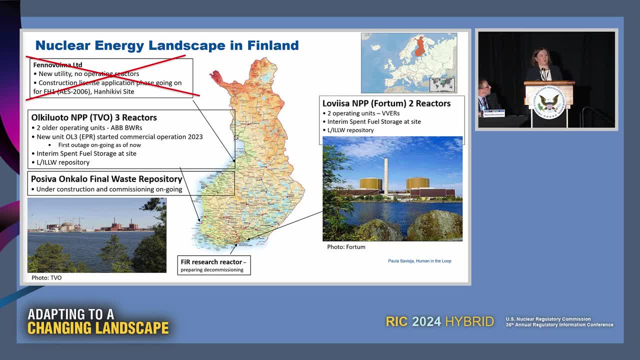 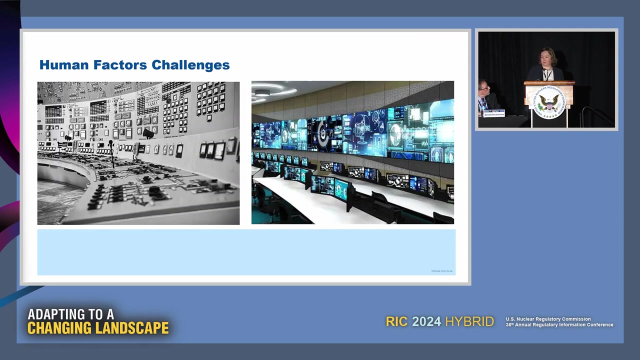 But from that we still have experience from how human factors were integrated in the basic design of a new plant. And on top of all this, like David said, our country is going through nuclear energy legislation renewal And this one goal for this whole renewal is to enable licensing of new reactor designs. 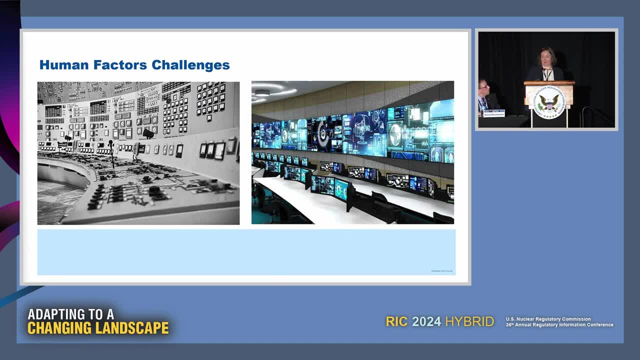 So let's go to the next slide. So what are the human factors challenges? I want to illustrate with these two control room pictures what I think is the challenge for us in this period of time. On the left hand side there is this old control room from where we, as human factor scientists, have a lot of experience with. 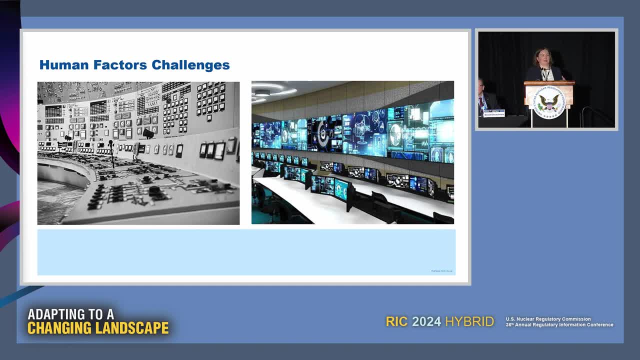 And we know what are the human performance issues and what to look for in evaluating the suitability of such control room. But as we are moving towards this more modern era, we don't have so much experience. We have some research experience but not real operating experience from these. 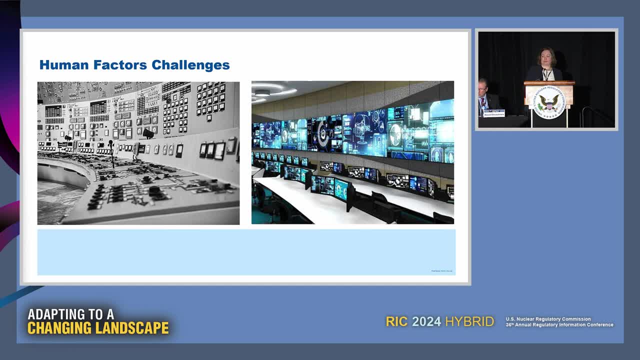 And for this reason I think that our human factors methods- we cannot be sure that our methods that we are using right now are such that they can actually point out from the modern control room what are the real threats to human performance. So it's a challenge for us human factors experts to develop our methods in a way that we understand what are the vulnerabilities of the modern control rooms that we are going to face in the near future. 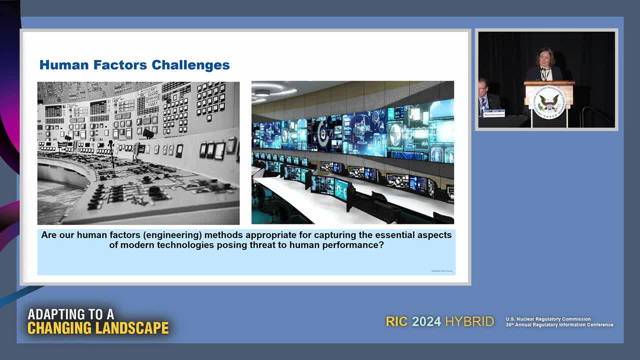 And in addition to this, the human factors engineering methods that I've seen being used in the industry are very much focused on the control room issues. Even I put the control room pictures there to illustrate this. But from my experience with the new builds I've seen that there are quite interesting human performance challenges also out of the control room. 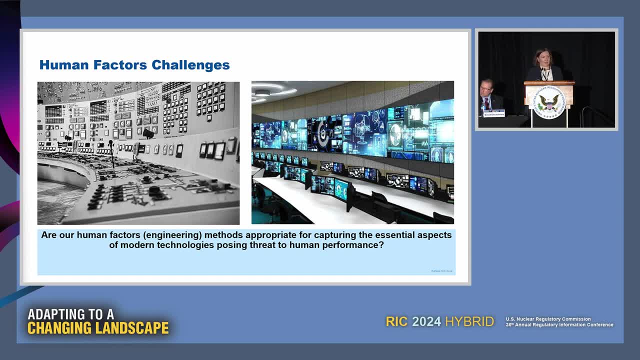 Especially there are the field operations, but there are also human activities like maintenance and assembly, testing, surveillance activities that take place on the field And what I have seen from the projects that I have been working with- human factors engineers- have not paid attention so much to these other human activities that are still quite safety critical. 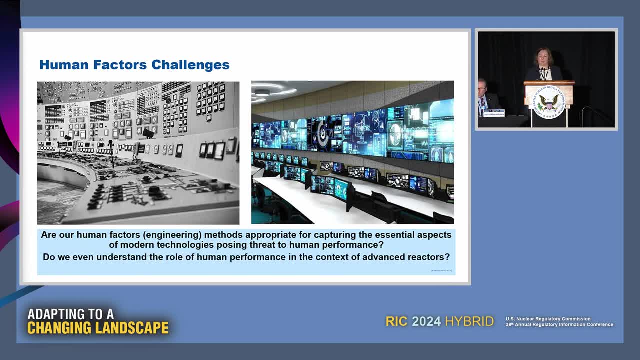 So my other challenge relates to this, that do we even understand the role of human performance in the context of advanced reactors? Do we know what are the safety criteria? Yes, There are safety critical human activities where human factors should be concentrating on. Surely there will be those control room issues. but there must be something else too. 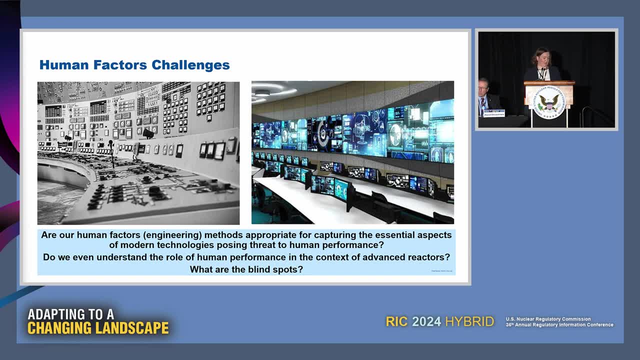 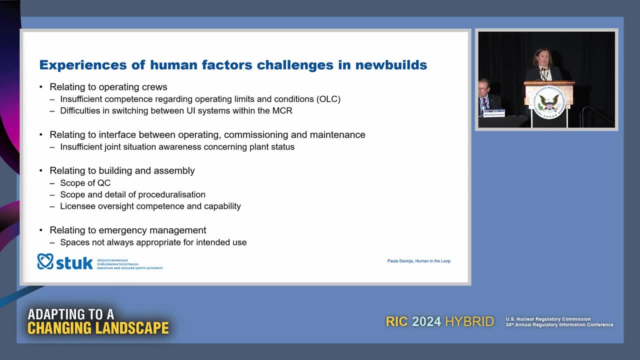 So I think there are some blind spots that we don't even know about yet. My last slide is a little bit of experiences that we have gained on these other safety critical human activities. Some of these were surprises to us And some were something that could be expected. 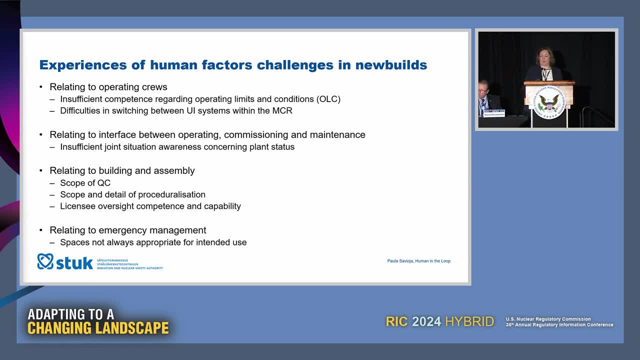 So, for example, relating to operating crews, we saw some competence issues, but they can also be interpreted as design issues relating to procedures and administrative procedures, And these are activities that the safety significant is not necessarily direct, but it's indirect, But there still is the safety significance. so, human factors, engineers should pay attention to designing the tools for different kind of functions at the plant. 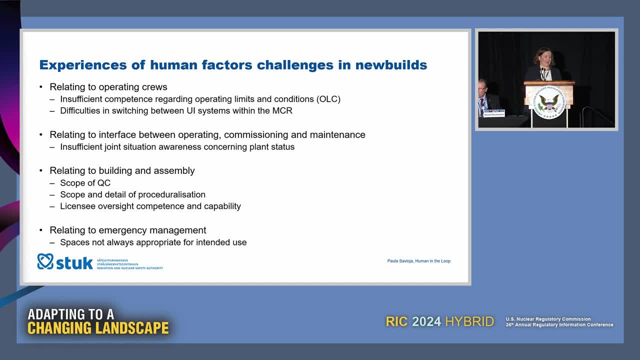 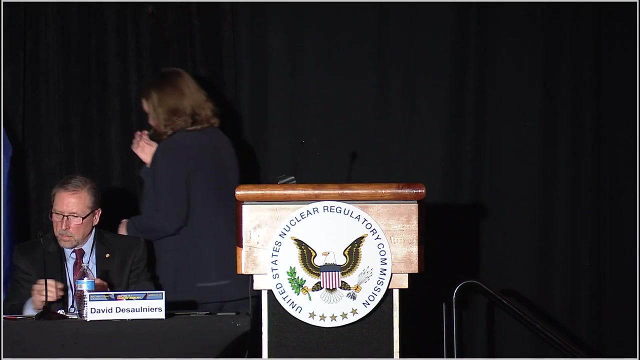 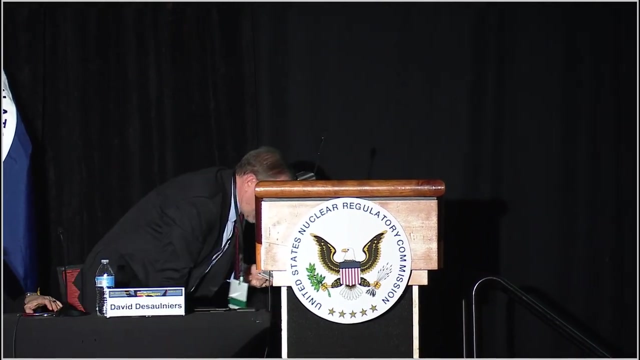 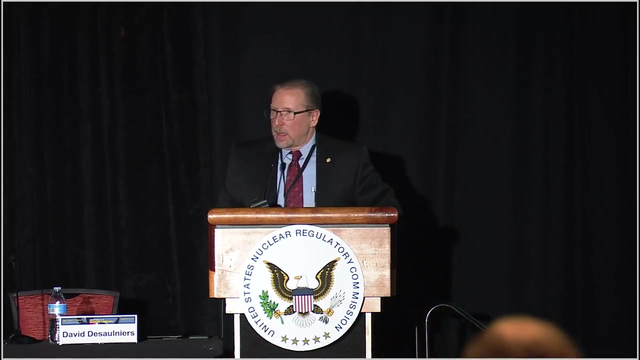 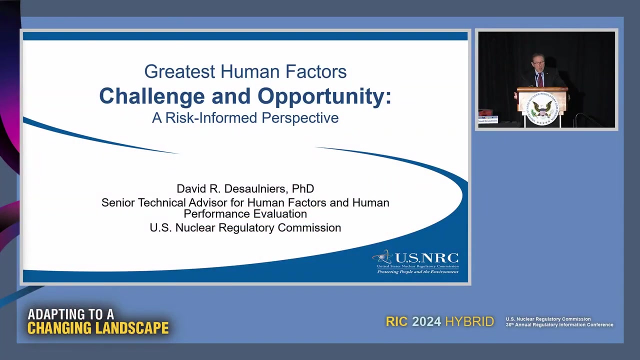 The last point there concerning emergency management is just an example that other functions, not only the control room operations, might become such that human performance is threatened. Thank you, Thank you, Paula. All right, my turn went up. So what do I believe will be the greatest human factors challenge? 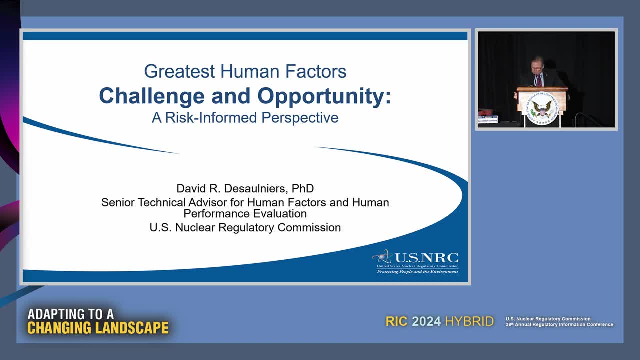 And opportunity that will be coming to the nuclear power industry. I will start by noting that I did not include in the future in my title. here, as I will assert, the greatest challenge and opportunity are here and now. You will also note: let's see, yeah, it's there that I included a subtitle: a risk-informed perspective. 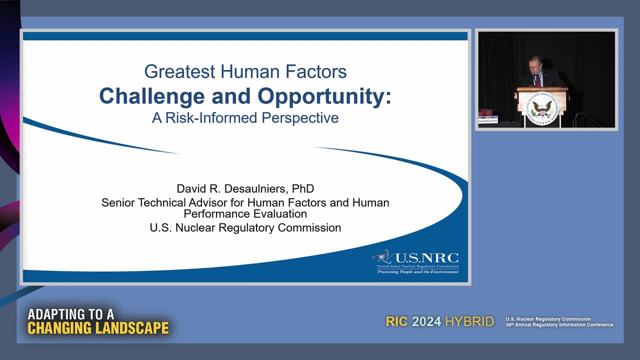 I'm perhaps regretting that I put that in the title now that I see Dr Apostolakis sitting in the front row, So, but I did plan to qualify that and that it's qualitative assessment. Admittedly, it was hard to discern between the futures that I saw what was going to be the biggest consequence. 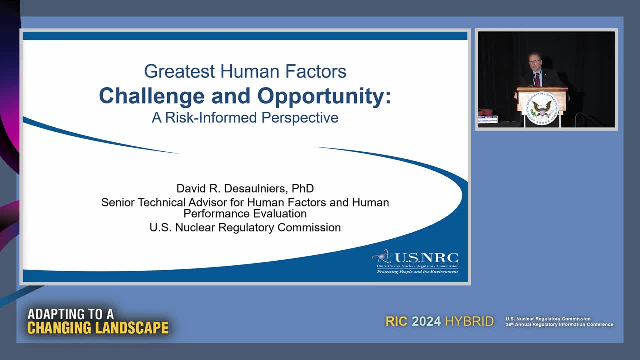 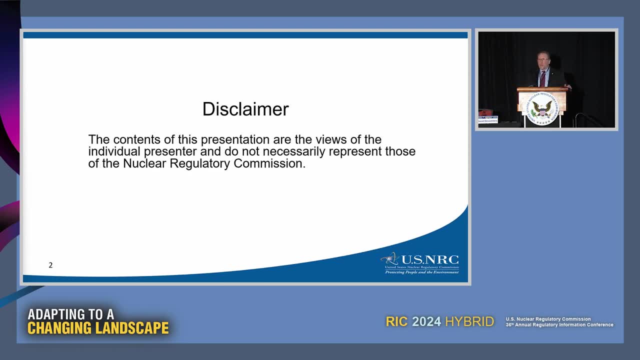 So I really focused on likelihood: What was the probability of what's to come forward? I need to provide this disclaimer because, unlike most presentations where I'm really just handing out the facts of what the NRC has been doing, these are really my views. 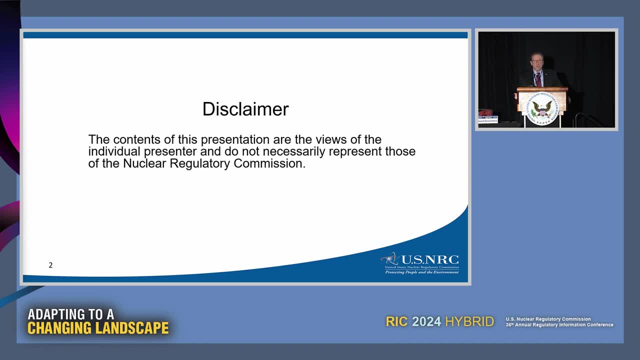 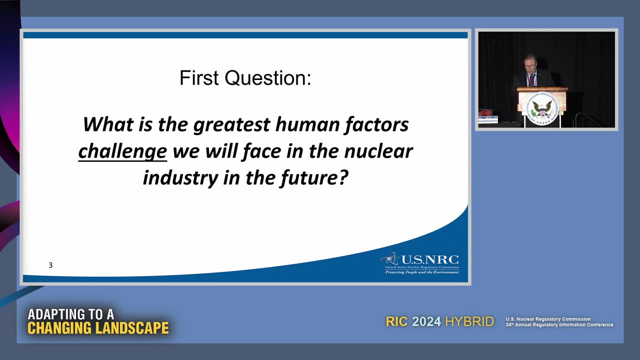 And so in no way should these be interpreted as necessarily representative of the US NRC. Thank you. So, beginning with the first question, the greatest human factors challenge, I started to think about the trends and topics that are getting the most attention in the human factors literature and in the nuclear domain. 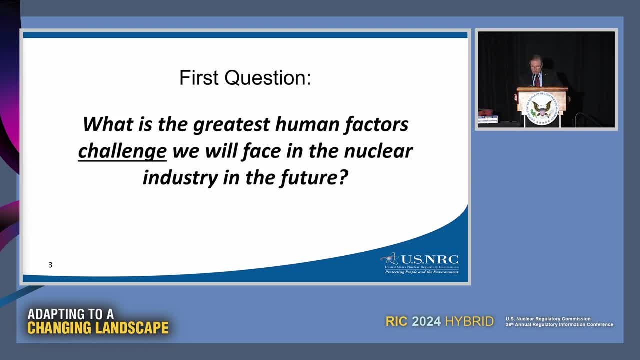 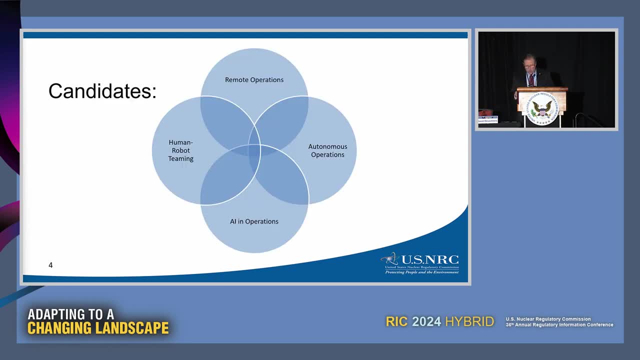 And the result of that reflection is what I've depicted on this next slide. Starting at the top, we have remote operation of nuclear facilities, And it was just a few weeks ago the NRC hosted a workshop on remote operation of nuclear facilities And in that workshop we heard a range of plans for remote operations. 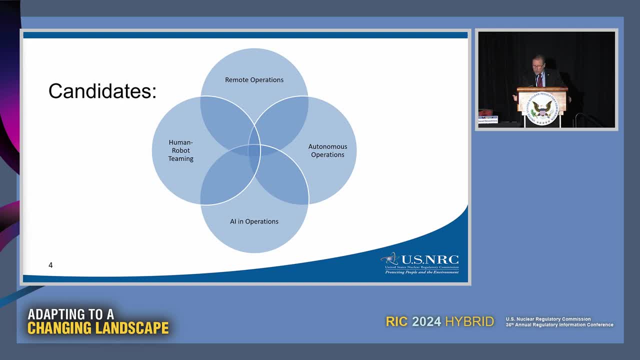 And in general, I think it's possible. we could be seeing proposals for constellations of small reactors being monitored and controlled from a centralized facility that may be far removed from the reactor site, Progressing clockwise. another development we could see is autonomous operation of nuclear facilities. 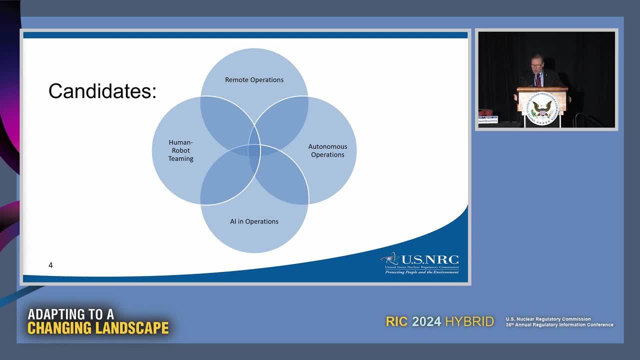 Facilities that have the capability to maintain steady state operations, handle plant upset conditions and shut down to a safe and stable state with little to no human intervention. A third development would be the use of artificial intelligence in the operation of nuclear facilities. AI applications are already in development for optimizing nuclear plant design, maintenance, corrective actions and operator training. 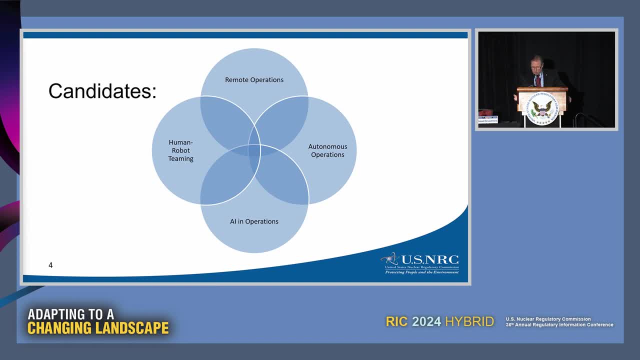 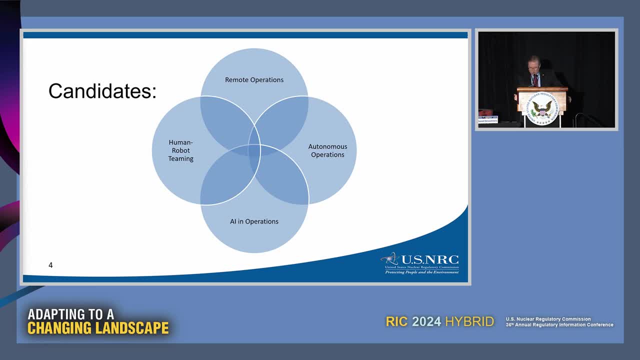 The fourth development depicted at 9 o'clock in this diagram is human robot teaming Robots have been used extensively in nuclear cleanup operations and now free roaming robots are gaining employment in the performance of nuclear facility surveillance tasks. I expect that successful performance in these applications may lead to future deployment and security in operations applications. 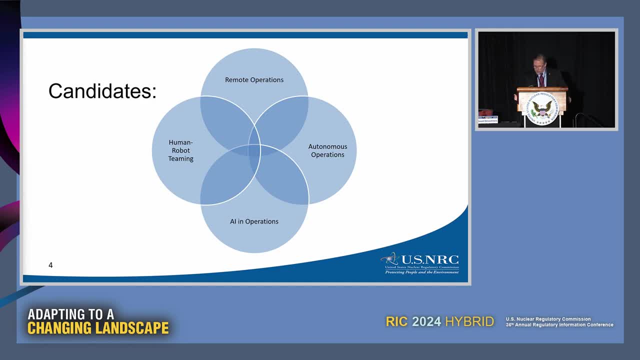 Now I could choose one of these futures as the greatest human factor's challenge, but the probability or consequences of developments in that area would likely to be open to debate. Rather, I ask you to consider the intersection of these developments. What they share in common might be our greatest challenge. 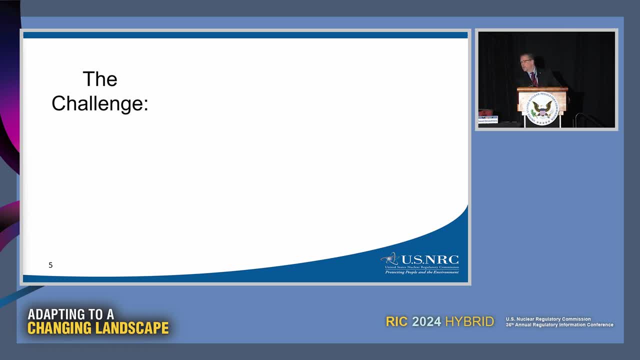 Hmm, Hmm, We have, Oh, So there it is. Could that be our challenge? The human factors professionals Might be surprising for me to say that Is it a conspiracy? No, it's simply a matter of numbers. The human factors community is small. 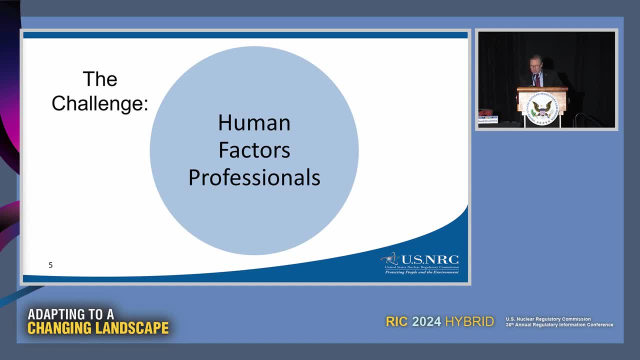 relative to other engineering disciplines and extremely small when you consider only those with deep knowledge in the nuclear power domain. At the same time, we are seeing new vendors and innovative designs entering the market. The individuals you see before you as panelists today are what you might call unicorns. 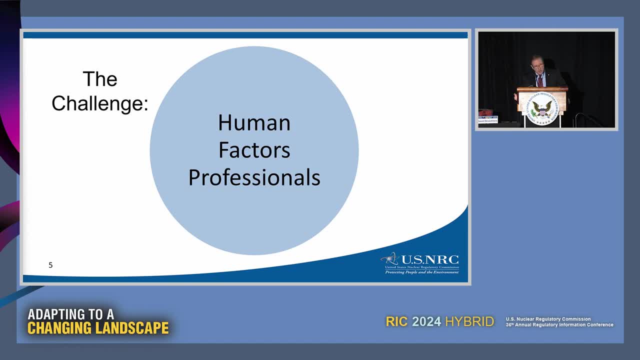 They are quite a rare breed And they are the type of people you will need to move something forward, And they are the type of people you will need to move successfully into any of the futures depicted on my prior slide. It is easy to fall into the trap of thinking that, as we move forward, 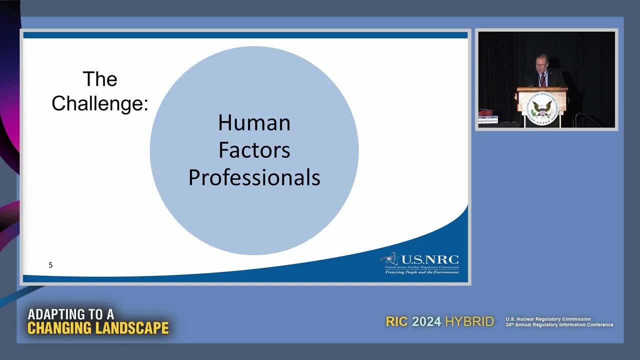 into a future where operation of plants is less dependent on human operators, that there will be commensurate decrease in the need to consider the role that humans play in ensuring plant safety and human factors engineering. I am cautioning you that such thinking would be part of a recipe. 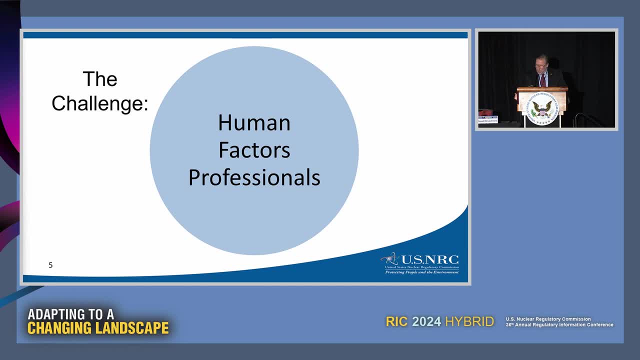 for bad output. If you consider each of those futures deeply, you will recognize that they are not really eliminating the role of humans in ensuring safety, but rather they are transforming the when, where and how. So how do we come to this situation? 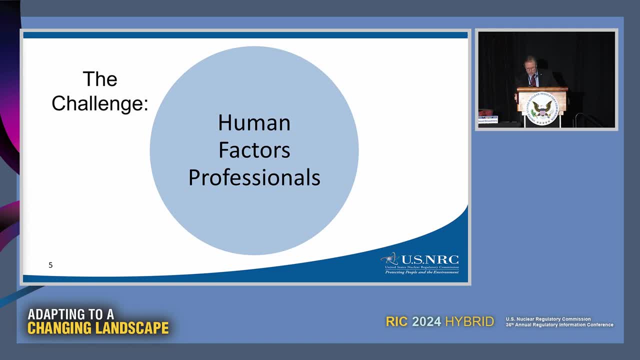 In short, the old post-TMI talent with nuclear industry experience moved on to other industries that were more rapidly evolving. They have now largely retired and sadly, many, I regret to say, have passed on. The new talent coming out of universities are being drawn. 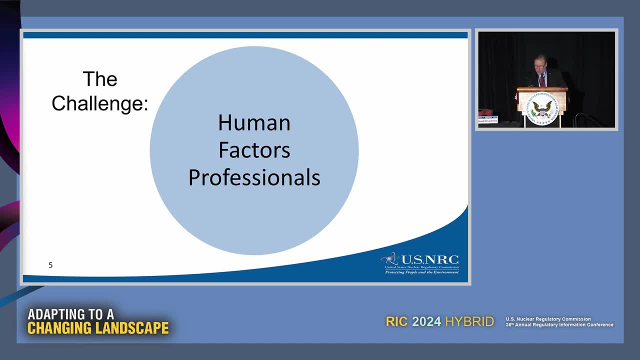 to those industries that are consistently funding research and innovative technologies, such as aerospace, telecommunications, defense, medicine. The flow of human factors talent to the nuclear industry is currently a trickle, And this limited supply could result in advanced reactor design solutions that are delayed or, worse, ill-conceived. 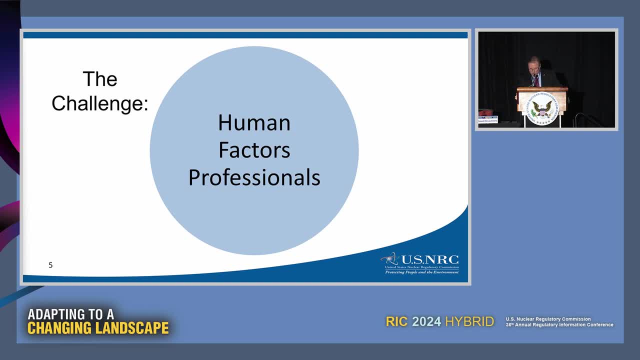 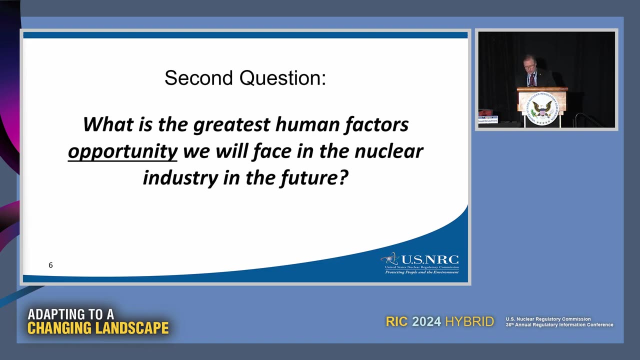 If this challenge is not met, If this challenge is not given due and timely consideration. With that cautionary note, let's move on to a brighter topic. Okay, so what is our greatest opportunity? Let's begin again with the same four areas. 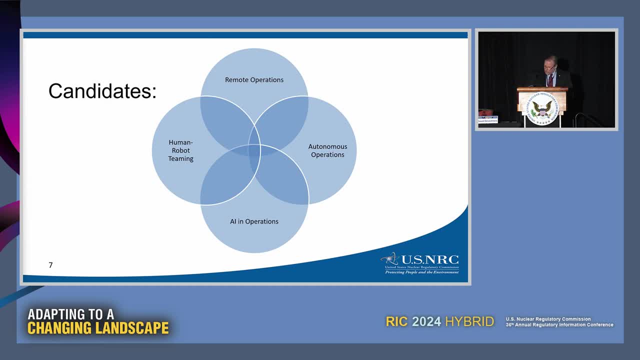 I believe it was just yesterday that Chair Hansen noted that optimists see challenges as optimists Opportunities. so our challenges and opportunities here are the same And again we could make an argument as to which of these holds the greatest promise as an opportunity. 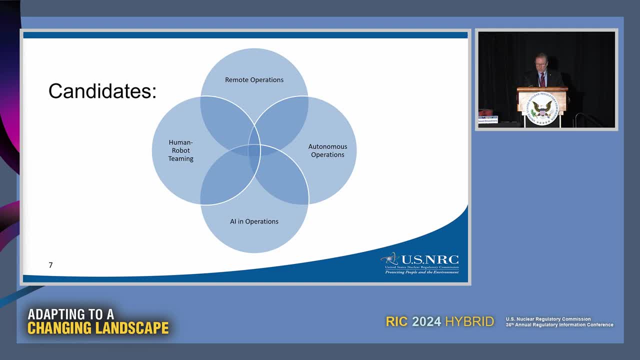 But, as before, I'm going to hedge my bets and look at the intersection of those futures and consider their commonality. Whichever direction or directions one might head, the greatest opportunity is the same And the good news is, you know we're going to have to do this. 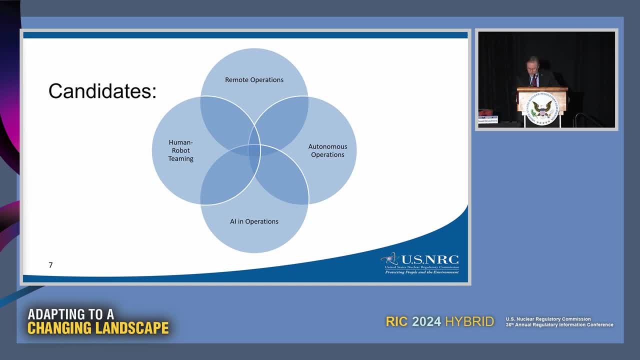 And the good news is that it is here. it is now. you don't have to wait. In fact, if you wait, you'll miss the opportunity. Perhaps I should just pause then for the next slide to build the dramatic tension, but I'm running over in time. 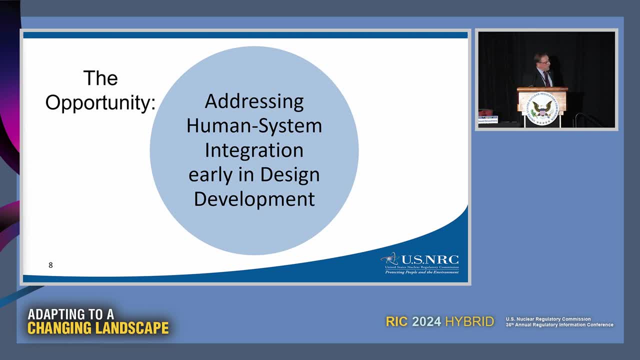 So the opportunity is addressing human system integration early in the design process. I think you've heard that from my other colleagues here in other in their presentations earlier. So for those of you who may not be familiar with the term human system integration, I would like you 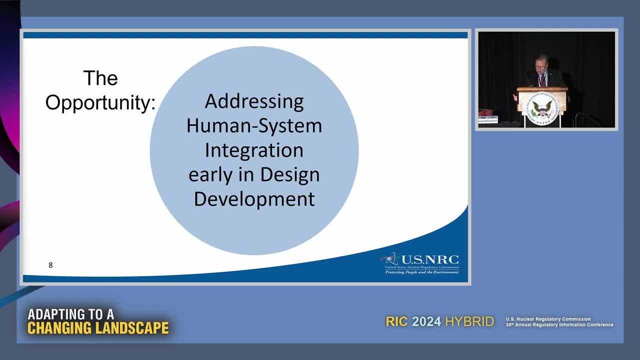 to think about it as one of the primary objectives of human factors engineering. Put simply, from my perspective, it's the process of optimizing a design by respecting the needs and capabilities of the human, the hardware and the software elements. So it's an opportunity to build a system. 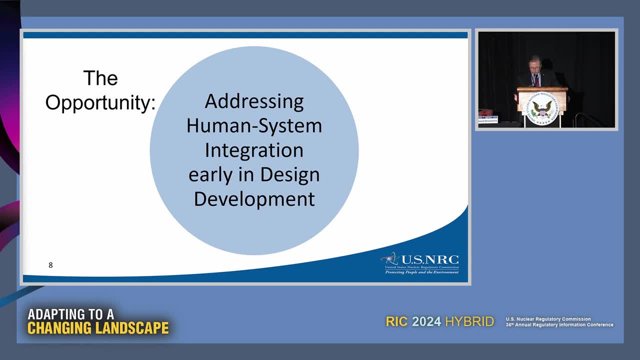 that has the capacity to meet the needs and requirements of a system such that they work seamlessly together to achieve the system's mission objectives. I noted earlier in this presentation there was a big uptick in human factors following the accident at TMI. Those human factors efforts were important and worthwhile. 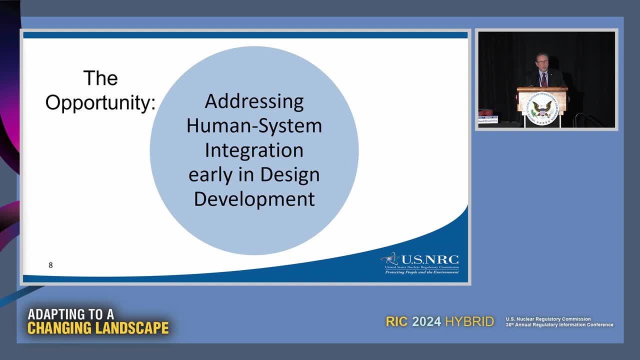 but they were tantamount to building lifeboats after the ship had set sail. It's not what I would call a recommended practice, Addressing human systems in a way. you know that we could. you know, system integration early throughout the design process will provide the best. 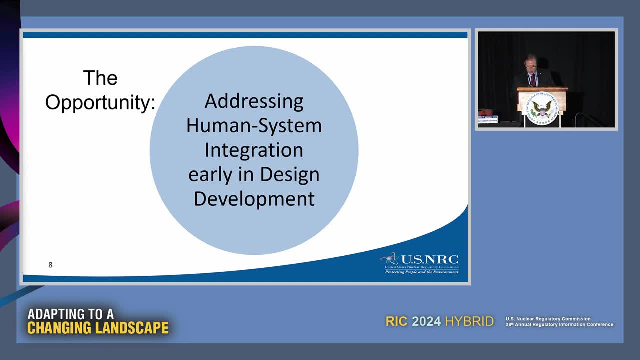 opportunity to identify and implement optimal design solutions and minimize rework. As such, it will pay dividends not only during the design process, but throughout the operational life of the plant. It can be your most cost-effective path forward towards safe and efficient plant operations. So this concludes my 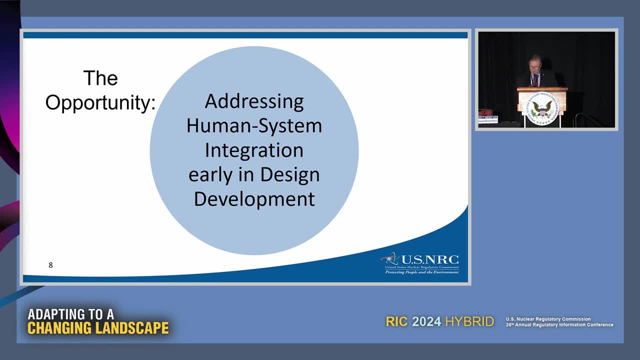 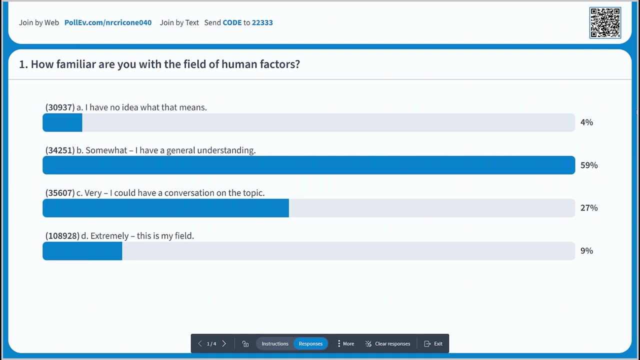 remarks, and I think at this point what I would like to do is perhaps go back- and I know we put up a polling question before. Can we put up the results of our first polling question? Okay, so we had very few that have no idea what human factors means, and that's. 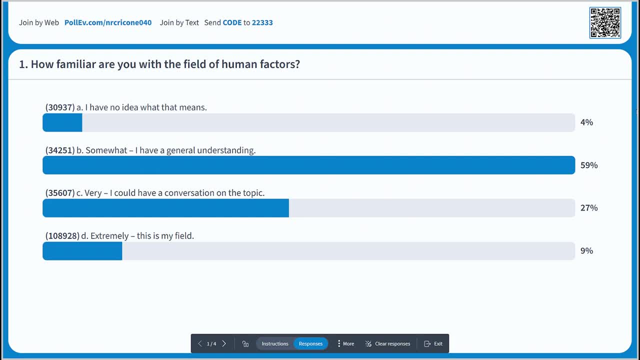 that's. it's probably a little bit more complicated than I thought. it would be Probably a skewed audience, given that he came here to this session, But I'm going to ask if any of my panelists would care to, just for those that may not be. 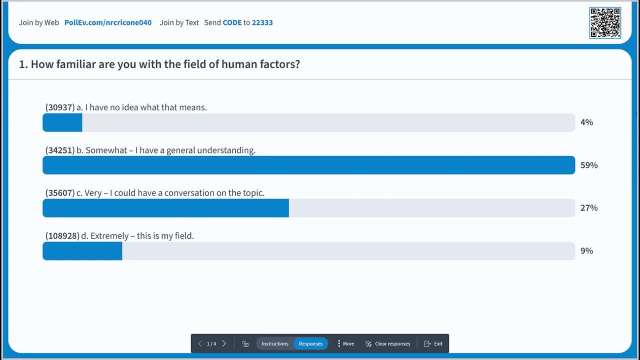 familiar with human factors. how would you explain human factors to your friends or family as a discipline? Anyone want to take that one on. Well, I'll say you know, as I explain it to my, my wife and my family, I usually use my phone as an example. You know, I think we've 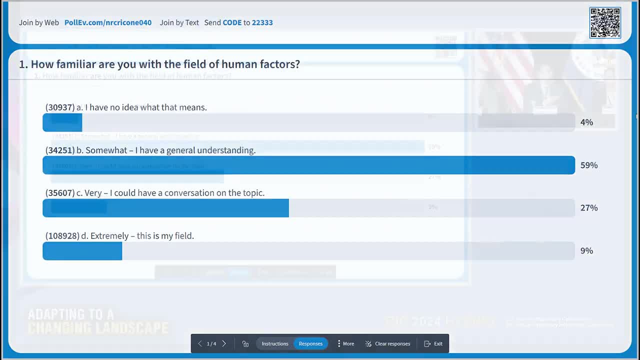 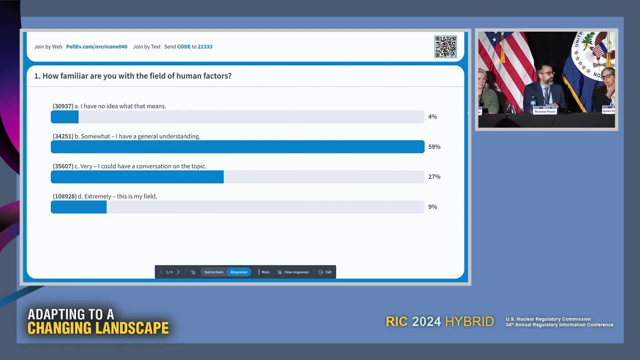 we've- all of us- have been in a case where we have no idea we want to do something on our phone, and whether it's an app that we can't navigate or we can't find out what information or where the information we need is, you know the. 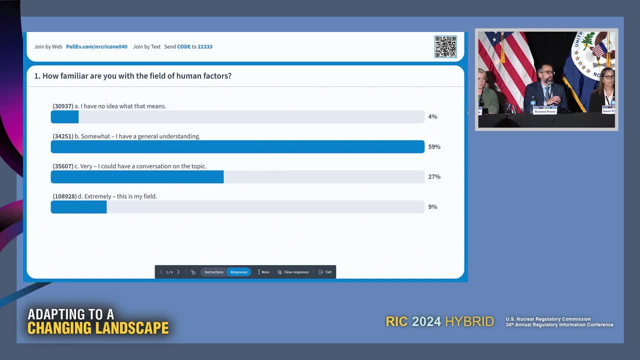 design of that interface is is where human factors comes in to make things, technology, your phone, more easily usable. and so, to me, human factors is, you know, designing systems and workplaces and phones with humans in mind, with our capabilities and our limitations and how we think, and so that's my simplistic. 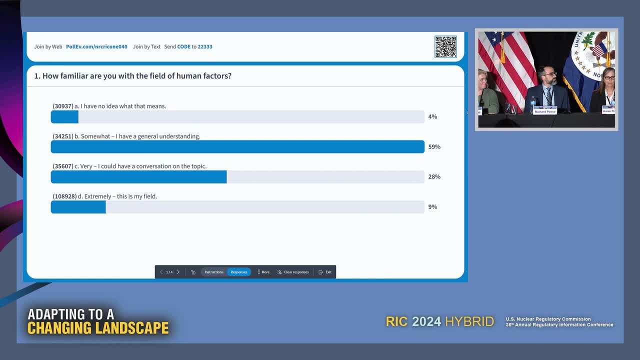 explanation of human factors. Good thanks. Anyone else want to add or amplify on anything? Rick said Good summary and you know I think I've explained it to people in the past in ways that were probably more focused on how we treat it here in the nuclear industry, because 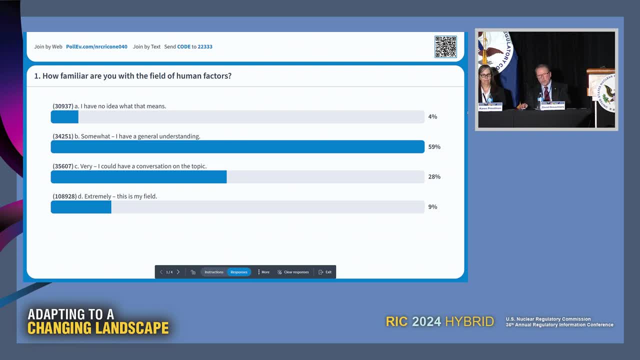 I always made reference to complex technological environments, but human factors really can be applied to the most basic of tools. We tend to focus on a rather complex tool, a nuclear power plant, and so I usually find myself explaining it in terms of the challenges addressing, the challenges of dealing with. 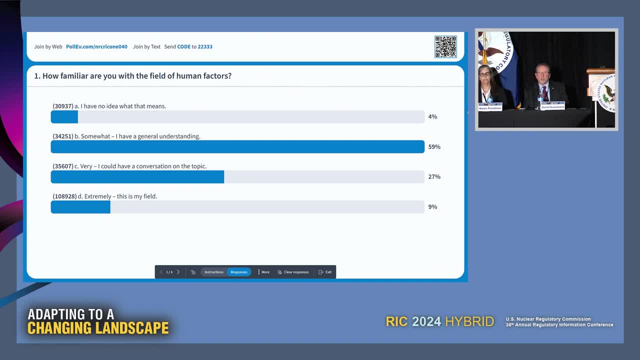 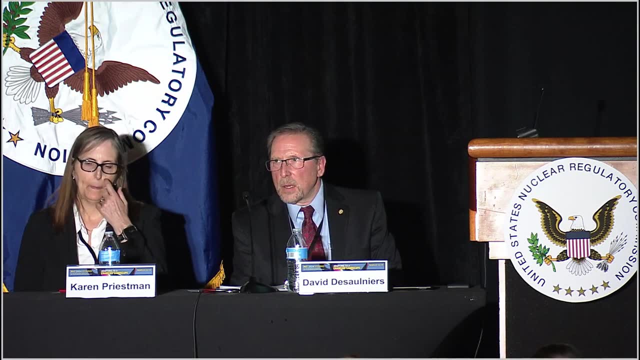 human limitations and capabilities in a complex technological environment. but it probably shouldn't be thought of as just limited to that. Also, thinking about it, we tend to also focus on just the cognitive aspects, because most of the work in a control room where we have focused historically has been the nature of 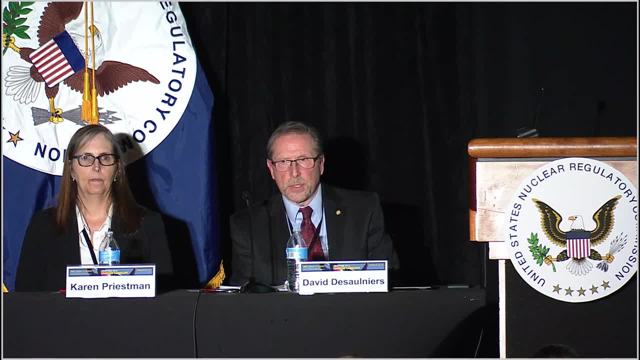 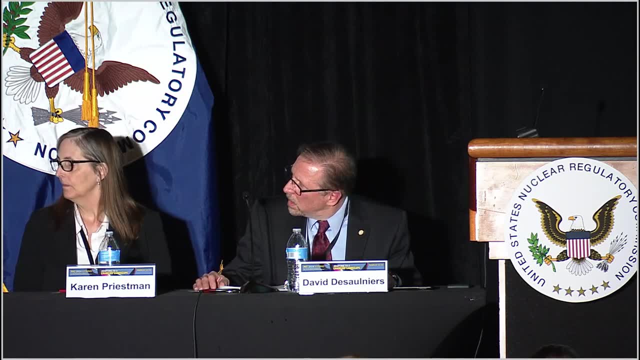 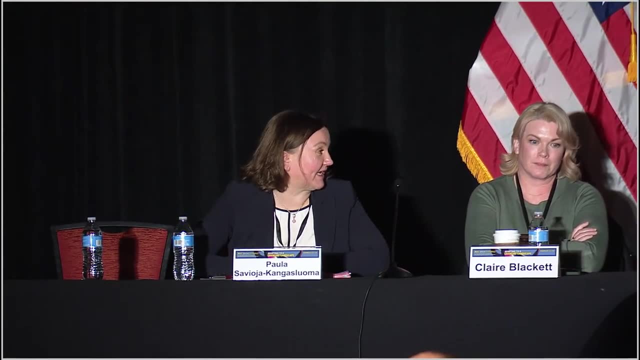 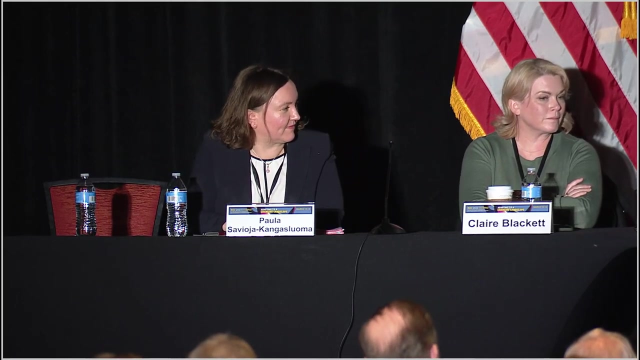 cognitive work. but human factors also encompass that, That physical aspect of human capabilities and limitations as well. To that I would like to add that also social aspects of human activities must be considered. so humans as team working and communities- Yeah, absolutely, and we find more and more in our community. 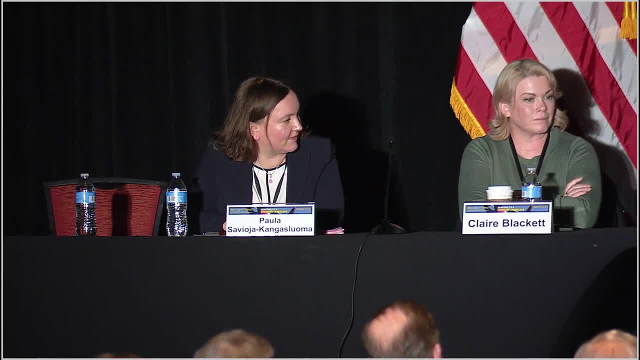 We try to incorporate- at least we've been doing this for a long time. but we try to incorporate- at least we've been doing this for a long time. but we try to incorporate, for example, within the NRC, our work in the area of safety culture. 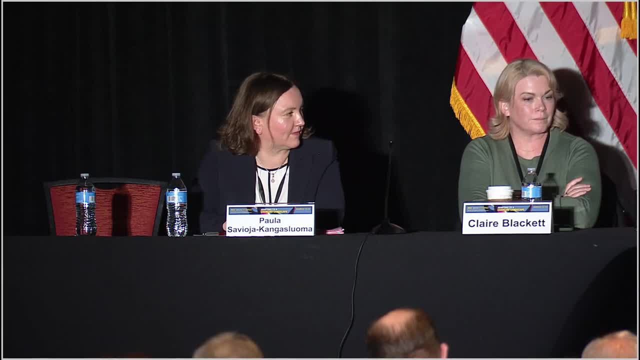 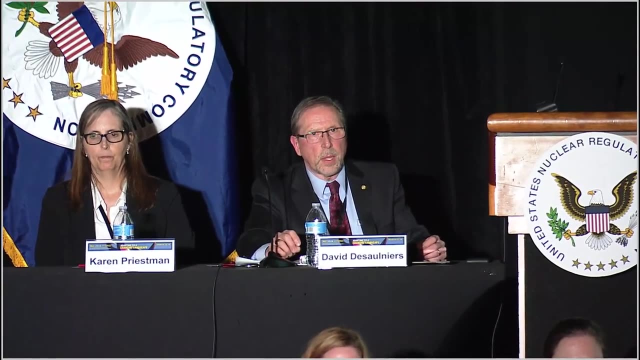 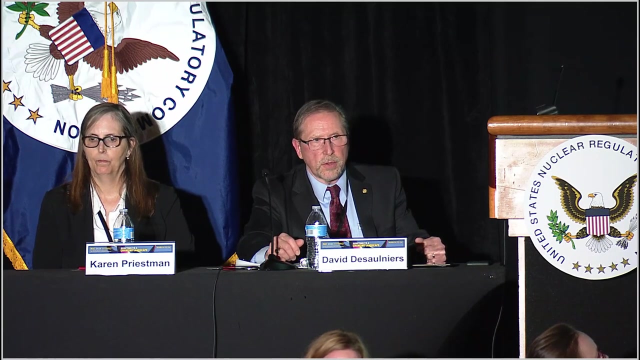 It all ties in as well as other organizational aspects. I'm going to ask that we put up the next polling question, and that was. the audience has now heard from all of our panelists in terms of their views on what they considered to be some of the most significant challenges. 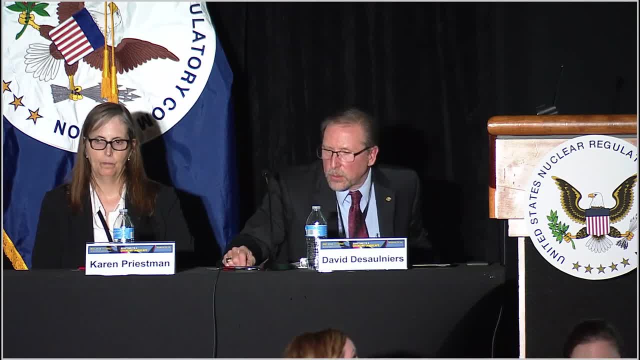 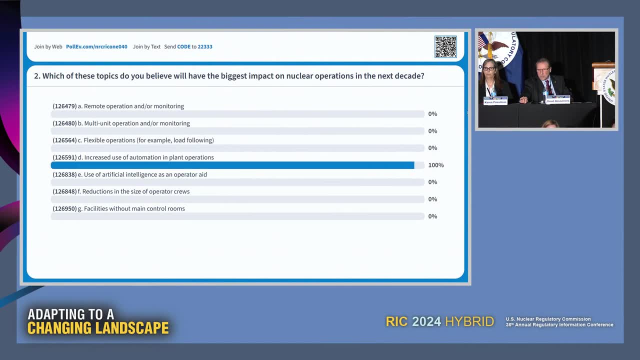 I heard some threads, comments throughout those presentations and some interesting differences. It'll be interesting to see what our audience thinks, so give a moment here to see what has resonated with our audience. Okay, And I'll just note that while that's coming in, clearly, this poll was created before I. 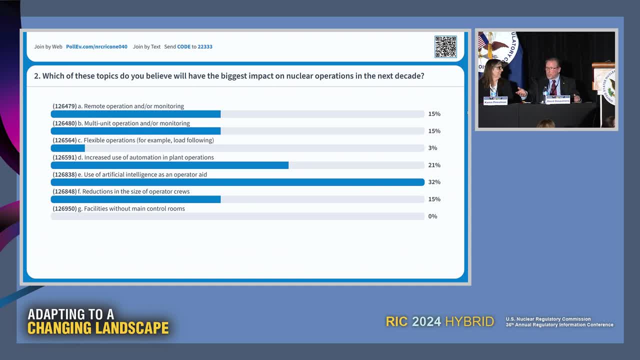 developed my presentation, so none of the options that I happen to suggest are on there. so I guess maybe that's saving me from embarrassment of finding out that my views just did not hit home with our audience. but let's see what comes up here. 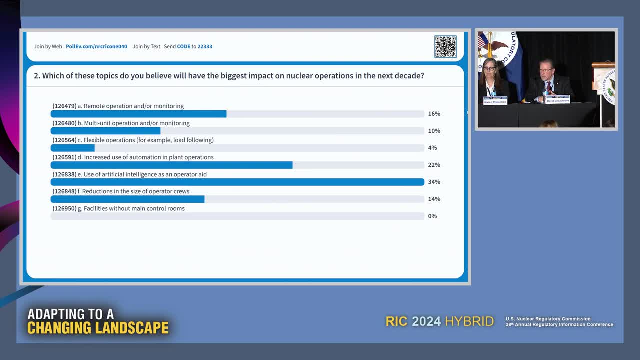 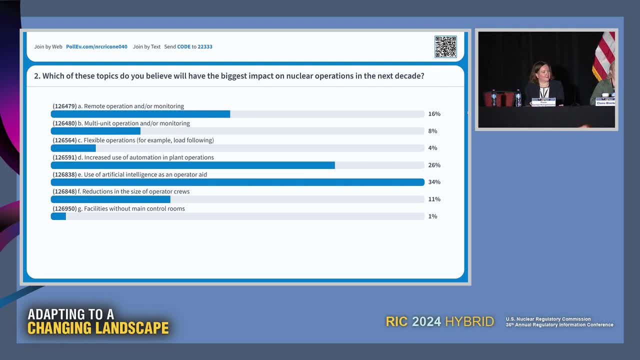 What are you thinking of the poll results here? Any reactions to either what's coming in, low or high, Any surprises you're seeing? I'm thinking that it's really difficult to predict what will happen in the future, And if any of those challenges or topics become reality, they will transform the way nuclear 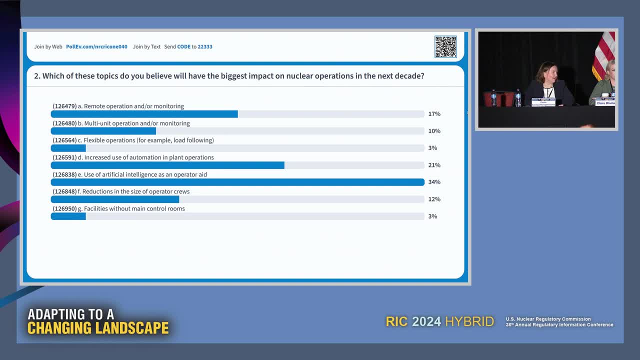 power plants are operated, So they will create challenges for human performance. But maybe it is the use of AI is- I kind of tend to agree with that- that it has the most potential for a complete transformation of the human role. It's not working. 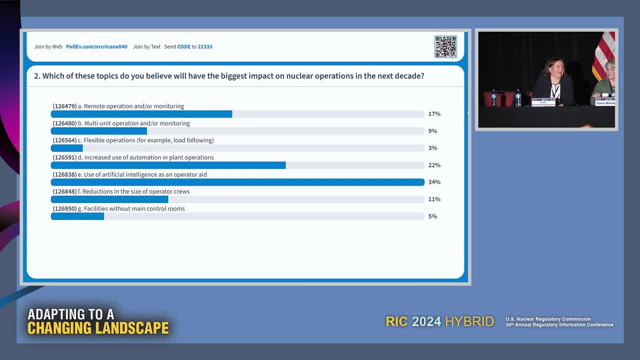 Oh, sorry, Done, Maybe I don't repeat my whole answer. Okay, Thanks, Claire. What's your thoughts? Yeah, Yeah, I agree with Paula that it's not exactly surprising to see things like AI and automation coming out on top. 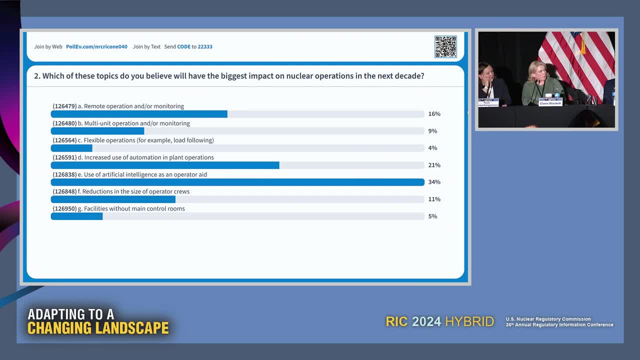 I think it reinforces the message that you gave, Dave, about the need for early human factors involvement. That's one thing that I think we've seen with the rapid increase in the development of AI over the last couple of years is that it's kind of advancing at a pace that is almost 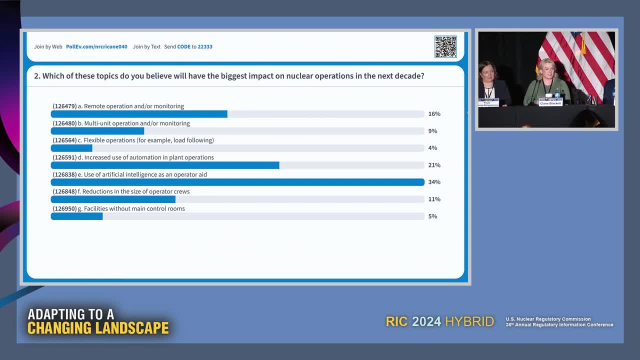 outrunning us And it's clear You can see clearly where people have taken a human-centered approach versus where they haven't. There are a lot of issues around AI when it's not designed with a human-centered approach, And I think that's one thing that we've seen with the rapid increase in the development. 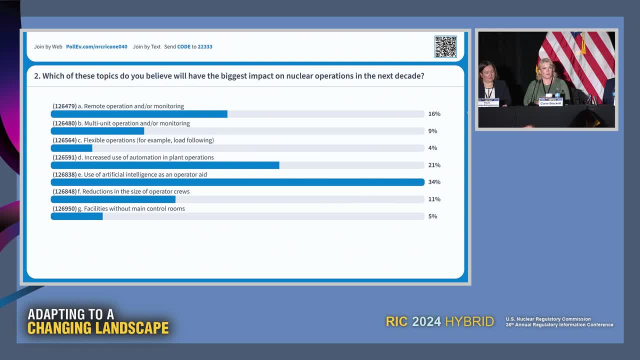 of AI. over the last couple of years, We've seen that AI has a critical role in the development of AI And there's a firm sense that it's moving in the direction of human-centered approach, Both in terms of how it can be used, how it can potentially be misused. 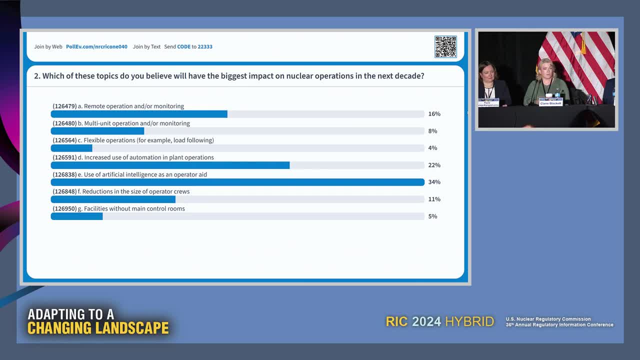 And that might not be an intentional misuse. It might just be an artifact of the way it is developed. So I think that if we do start to see AI coming into our nuclear power plants- and I do believe that we will- we need to think very carefully about why we are introducing it and where. 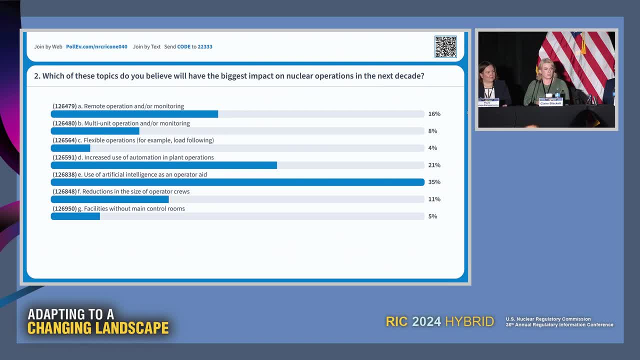 we are introducing it Right sure that we understand how operators will actually interact with this and use it as a tool to avoid any potential pitfalls. That's a very negative opinion, but it's human factors. But to add a little bit, I think it also means a significantly different competence requirements. 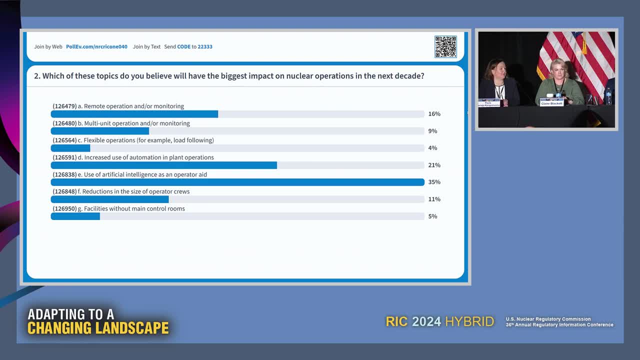 for our operators in order to understand how the AI is working and why the justifications for the decisions that AI might be suggesting So significant competence requirement changes for operators in any of those, but particularly with AI. Yeah, I think. I think the pooling is right on with the AI thing. 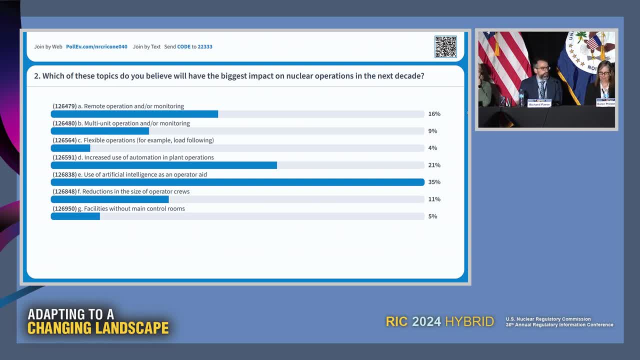 One of the principles that we have for our safety systems and our plant is that they're deterministic, meaning that we understand, if we give it a certain input, that we're gonna get a certain output from the system, And with AI it's not like that right. 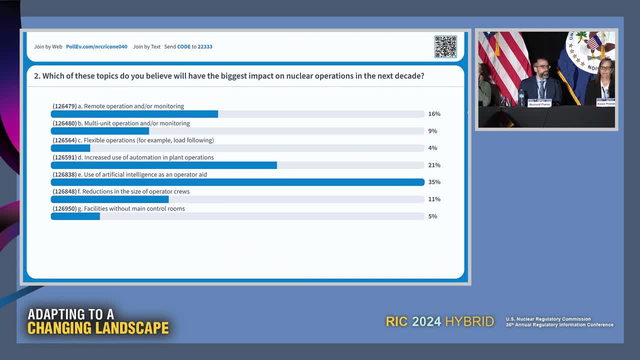 Sometimes the activity or the automation that That we get from AI could be unpredictable. My experience, admittedly, with AI is limited to chat, GPT and other interfaces like that, But I know that if I ask a question into chat GPT, sometimes you get different answers and 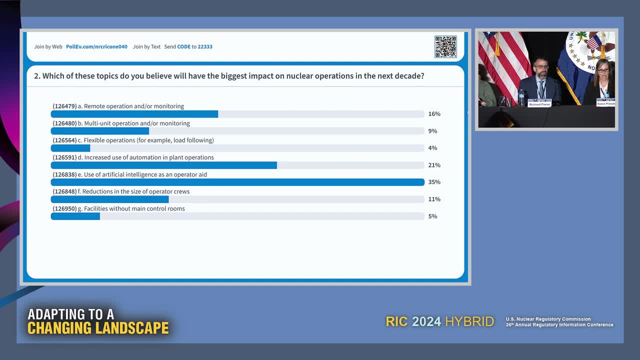 it's not a predictable response And so, as someone who's not an expert in that field, that's one question as a layperson with AI would ask and would be questioning is the predictability of the response of AI. I think that's a great point. 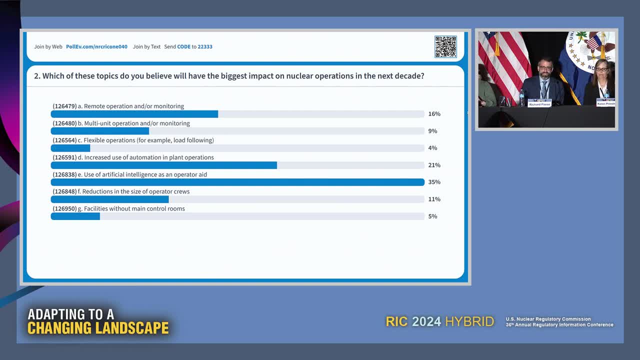 I am a little- Maybe I should be, but I was a little surprised to see facilities without a control room lowest on the list- or at least the pooling data I'm looking at right now is almost the lowest. I think that might be one of the one items that we actually have a general design criteria. 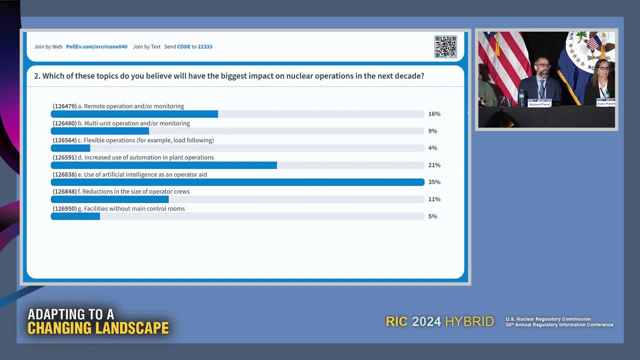 for our plants is to have a control room. That is actually one of our regulatory requirements and that appears low on the list. So again, maybe I shouldn't be surprised, but that was interesting to see that people don't see that as one of the top challenges. 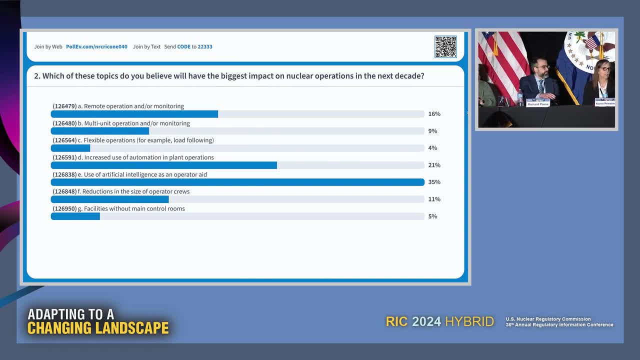 So those are my thoughts. So those who You want me to just: It's okay, Yeah, go ahead, Yeah, please. Those who know me won't be surprised to know I have a little bit of a different take on this. 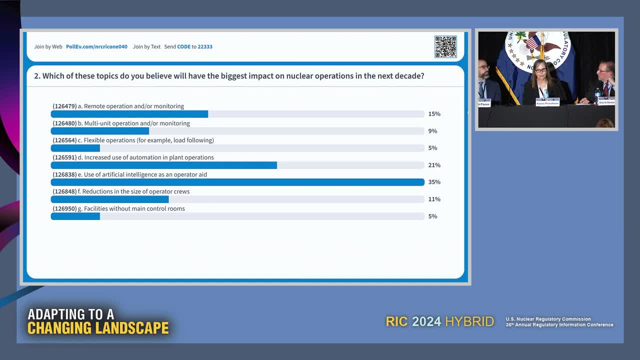 I would suggest that the biggest impact is the fact that all of these things are going to come together And we aren't going to have just AI. We aren't going to have to just consider AI. That's why we have to think about this in a totally different framework. 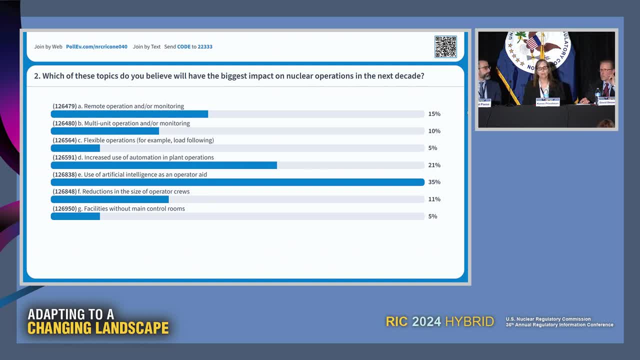 We're going to have all of these things Possibly in the same plant, and we aren't prepared for any of it. So that's where the impact is going to be. That's where the challenge is going to be. We have to consider it as a whole. 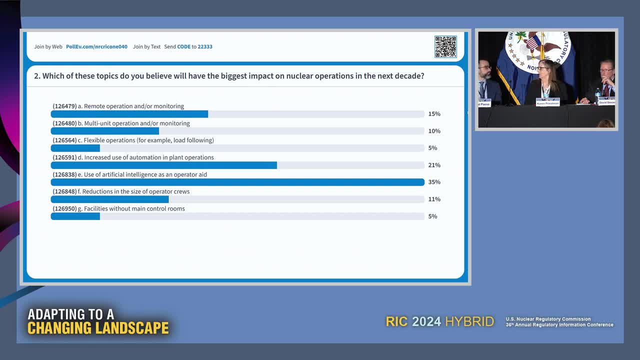 And so it isn't just AI, And it also surprises me about the facilities without control rooms, And I think maybe people think it's because there's no humans in it, but that's It's like the Tesla driving itself When they have to step in. that's the biggest challenge too. 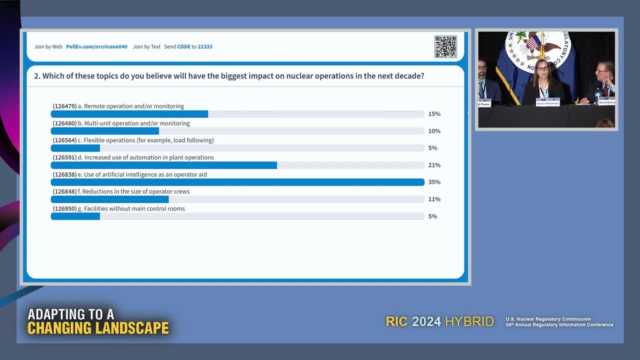 So, yeah, I think it's the fact that all of these are going to come together And then multiply exponentially. So, Yeah, People, We don't have enough people, Dave. Yeah, I think I would agree with Karen's comment there. 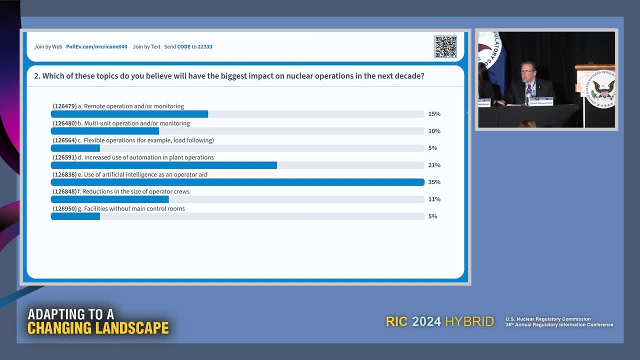 It was one of the reasons why I opted, when showing the potential futures or future technologies, to show them in a Venn diagram. I had to kind of cut my comments and didn't have an opportunity to note that, as you look at these, some are. 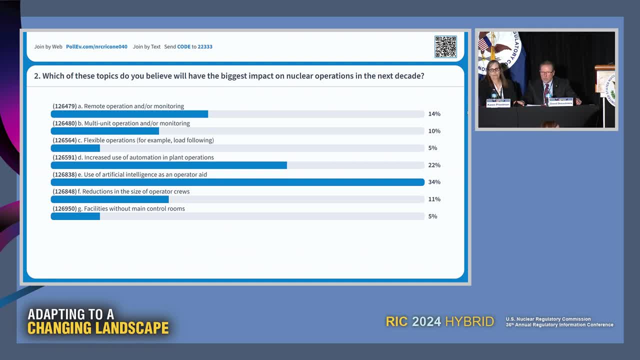 Can be considered enabling technologies for some of the other futures. So I do think that we will see those in combination. You know, the AI piece was one of the reasons why at the beginning of my presentation, or at the introduction of this workshop, I said: think about human in the loop as opposed to. 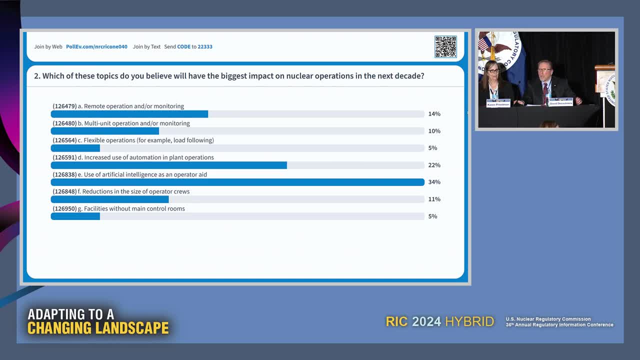 man in the loop, Because when you think about AI and its tremendous capabilities, the one challenge that we know still remains is that How do you use it? How do you build morality into an AI? And that may be one of the things that some of you thought about in terms of the difference. 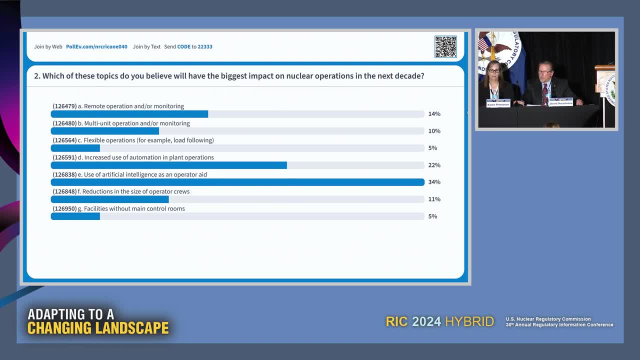 between humans and machines. So I'm going to pause there so we can move on to some other issues. But I guess, before I move off this topic- hopefully you've all noticed that directly following this session- And we did this on purpose- is that there is a session that will be on AI. 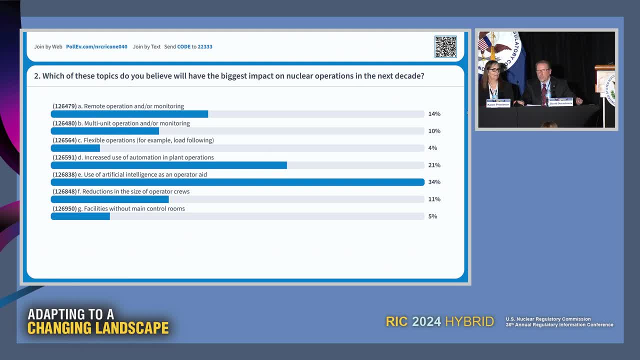 And so if you have a particular interest in this topic, please attend that session. We wanted to make this a broad discussion of advanced concepts of operations, not just AI. There are a lot of other interesting challenges to be dealt with, and they'll go much deeper. 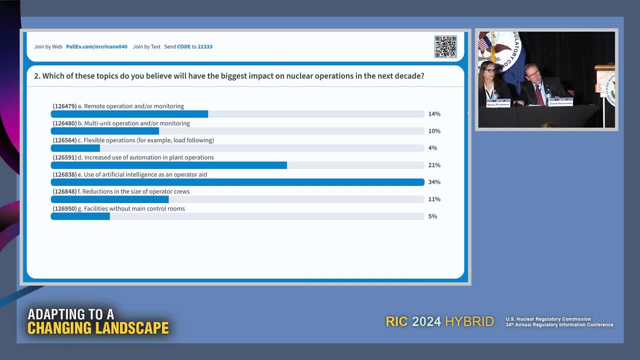 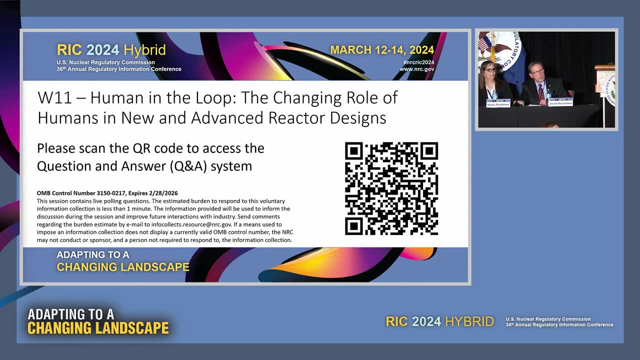 into this topic in that subsequent session. I understand that we have a question from here In the room or a comment that wanted to be made, so I want to acknowledge Dr Apostolakis. Maybe it's not a good question for this session, but we keep talking about the AI as an operator. 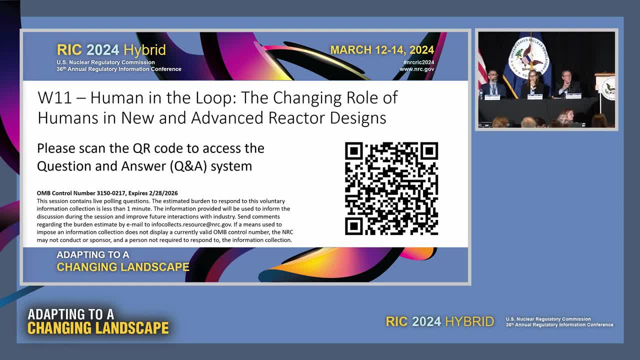 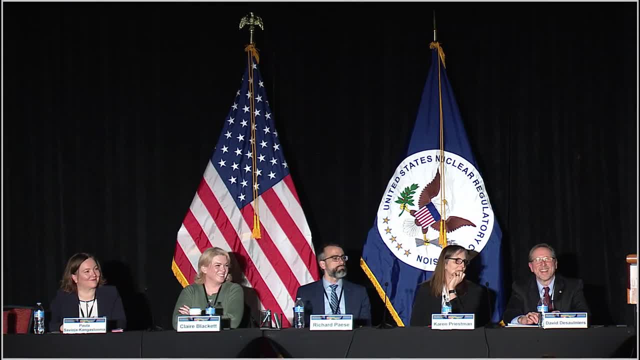 aid. I don't know what that means. What can AI do for the operator? Maybe it's for the next session, But we keep talking about it, Thank you, And I don't know what AI does. So one of the areas where it could be considered an operator aid is as a decision support. 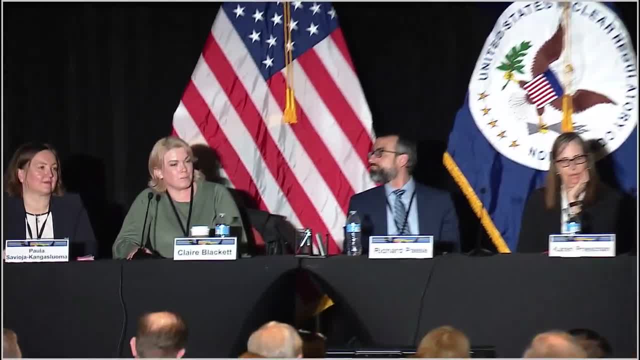 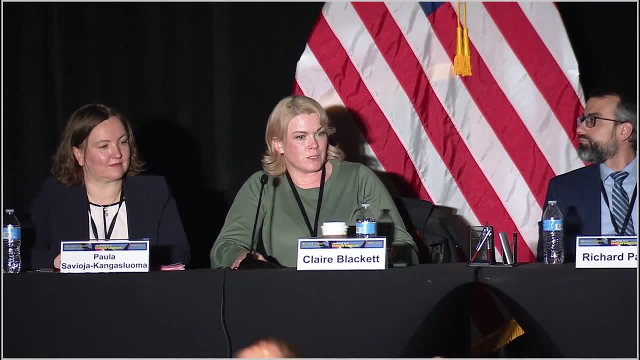 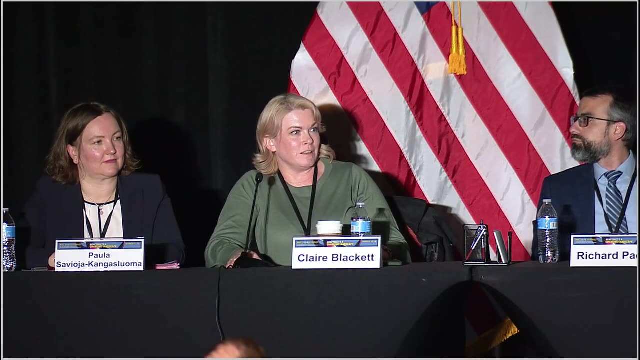 So, if we think about concepts for future designs, we tend to talk about them as being highly automated systems, and so they will be producing huge amounts of data, And we know that machines are much better at crunching data than humans, and so that 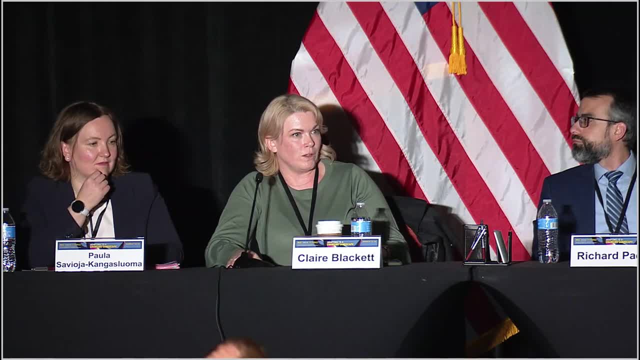 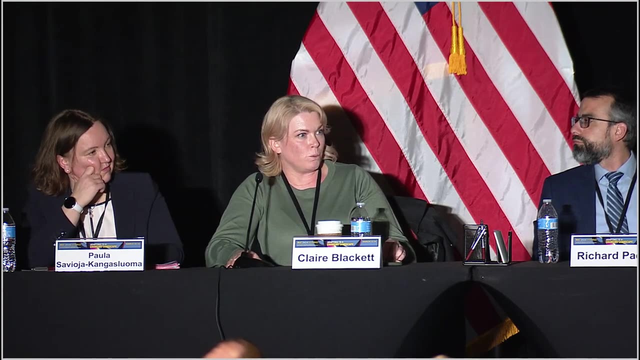 is one area where AI is being discussed is in terms of decision support. It's not clear to me how that will look yet, but at least that's when we talk about it as an operator aid. that's one type of aid that comes up a lot is a kind of a decision. 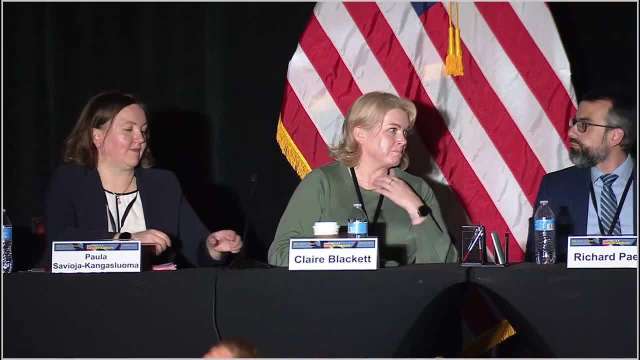 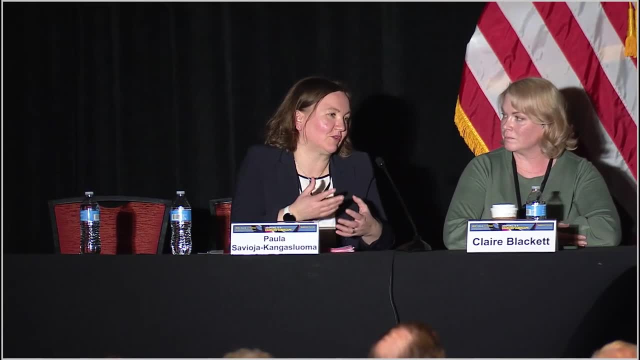 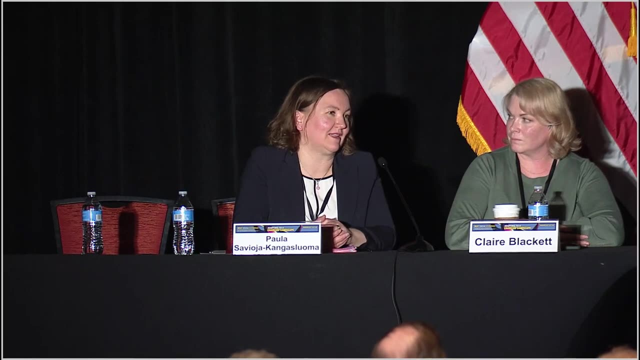 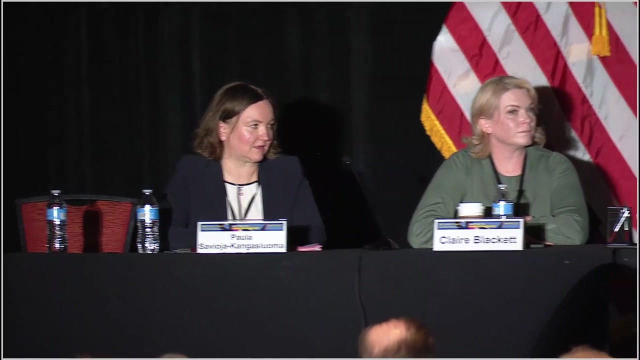 support system. And when saying operator aid, it doesn't necessarily mean the control room operator. It can be any human operator who is benefiting from the results of the AI, And I guess I would add to that when you think about it as a decision aid. so my understanding. 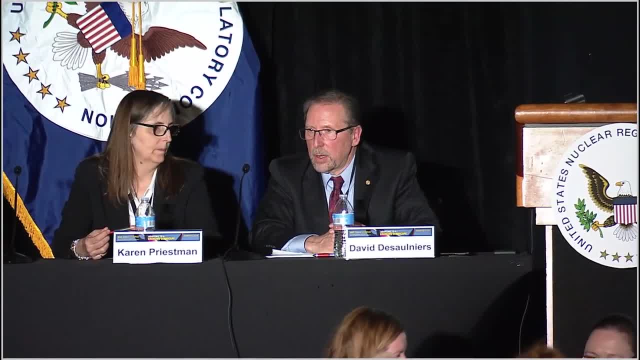 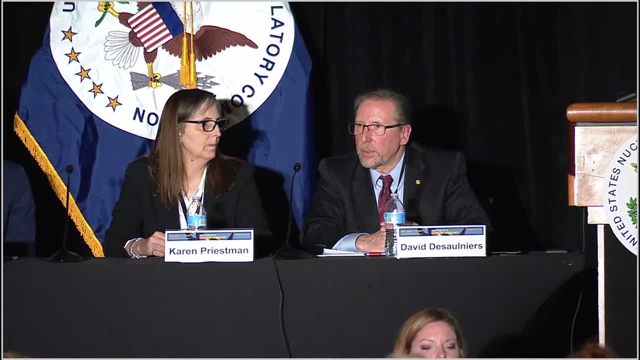 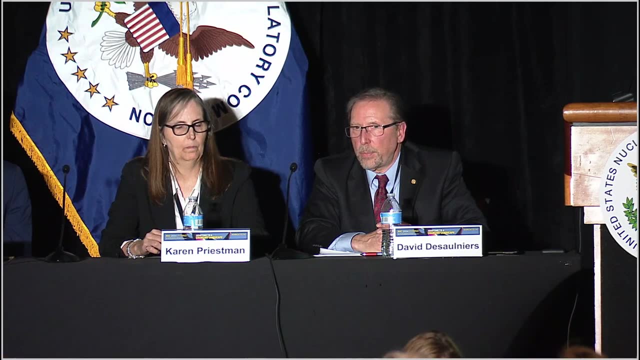 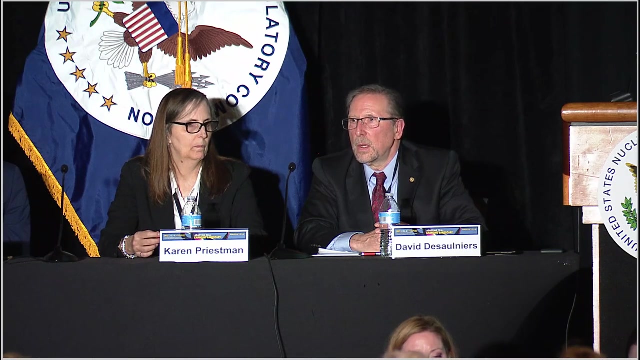 of different types of capabilities that are being developed would be to aid in diagnostics and prognostics of system performance. So you might expect that an AI system might be more capable of picking up weak signals in a system performance that just might seem like noise to a human, but the AI is capable. 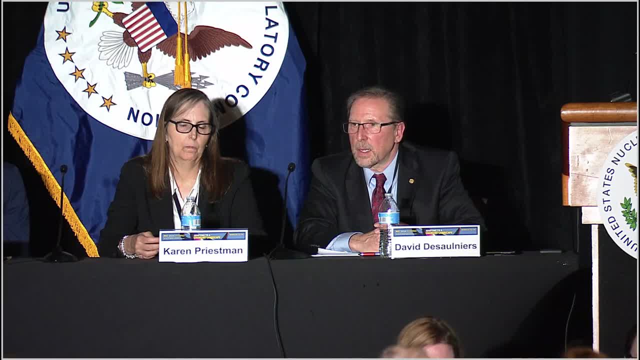 of doing that. So I think that's one of the things that we need to be thinking about in terms of analyzing that vast amount of data and recognizing that there is an anomaly and providing some sort of early warning of a degradation that might not have been picked up. 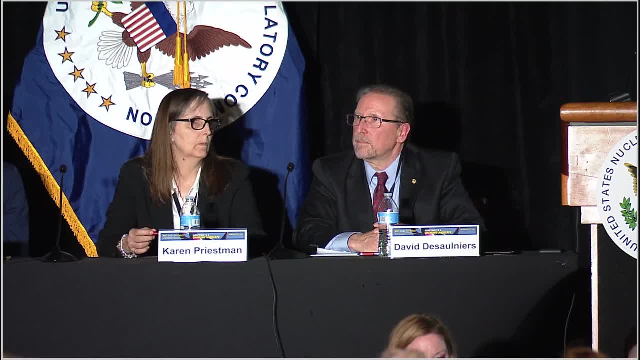 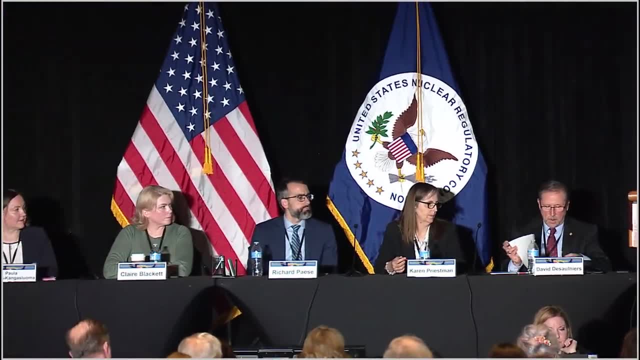 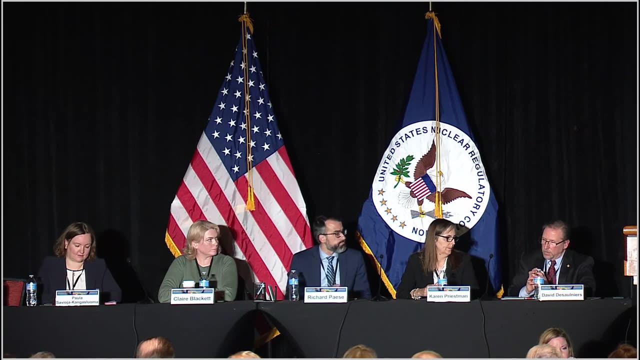 Okay, so I'm going to kind of just talk a little bit about what we're going to be talking about. I'm going to talk a little bit about what we're going to be talking about. I'm going to talk a little bit about what we're going to be talking about. 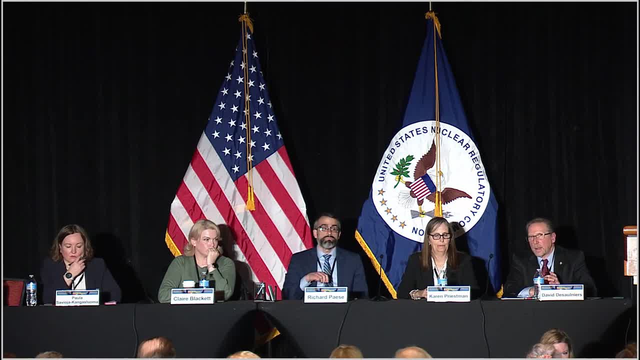 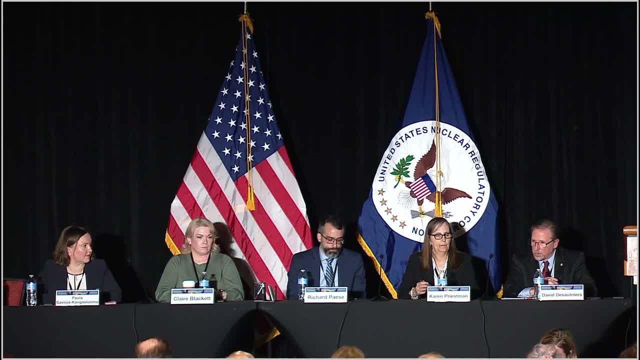 to just the question of automation in general. thinking about it more generally, What do our panelists think about what seems to be a push for more automation in reactors designs, and what might you see as the implications from a human factors perspective? Okay, 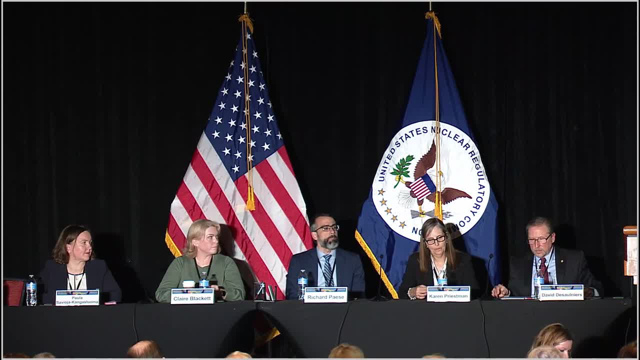 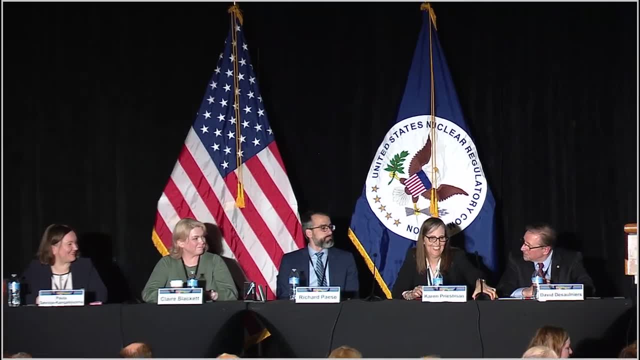 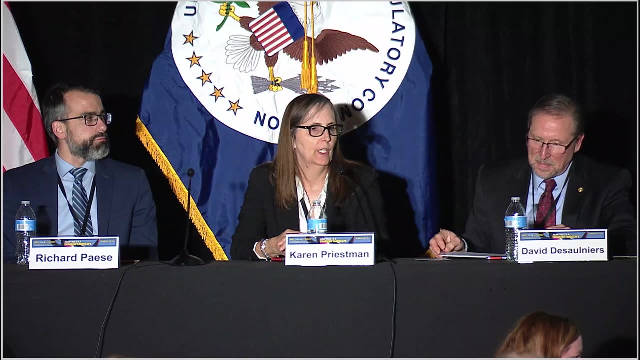 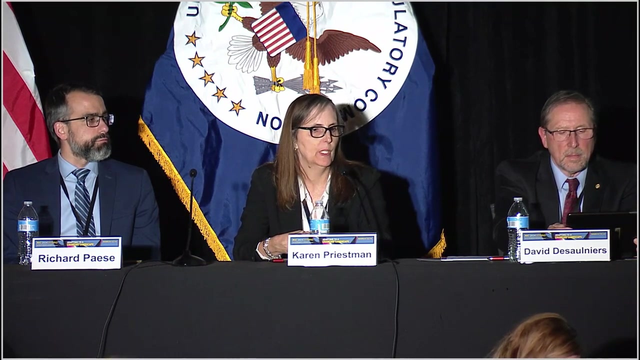 perspective, At risk of repeating stuff I said already and the things that the fellow panelists touched on. I think we struggle to understand the risks when we move to highly automated systems. And they don't lessen, they just move and they change shape, but we don't necessarily. 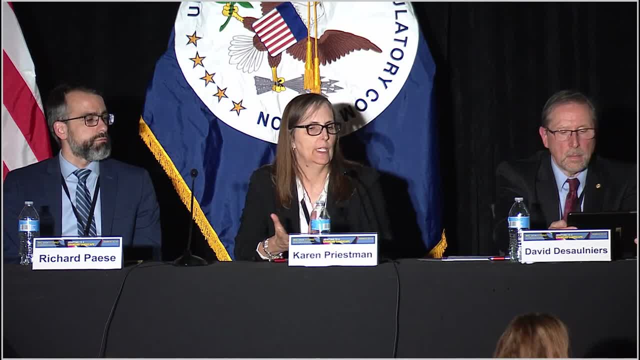 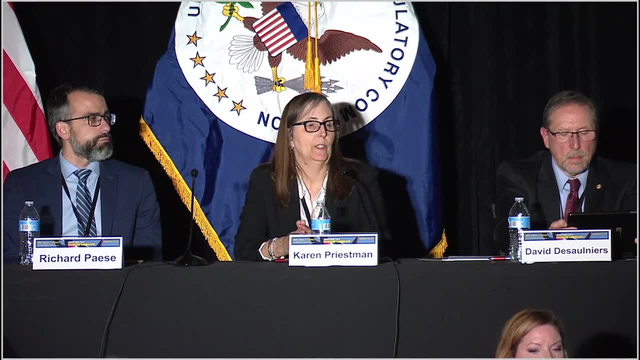 know how to assess those to provide substantiation for licensing. I think that will be a challenge. I think there is a mistaken- actually I've seen both ends of the scale- the mistaken impression that it's a much higher cost to introduce automation. 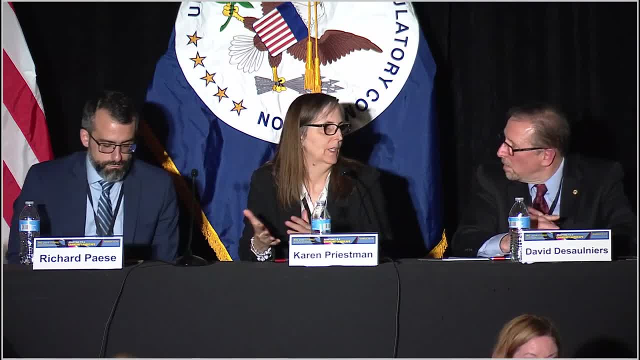 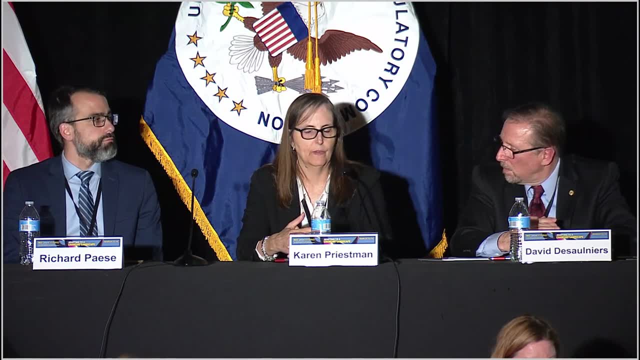 I've also seen that it's a much lower cost to introduce automation, And I don't think that's true. I think the cost just moves to a different- you know different- perspective. There's a point in the whole life cycle And I just think the challenges are different. 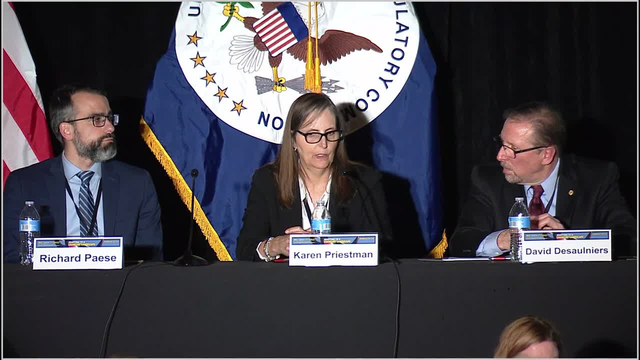 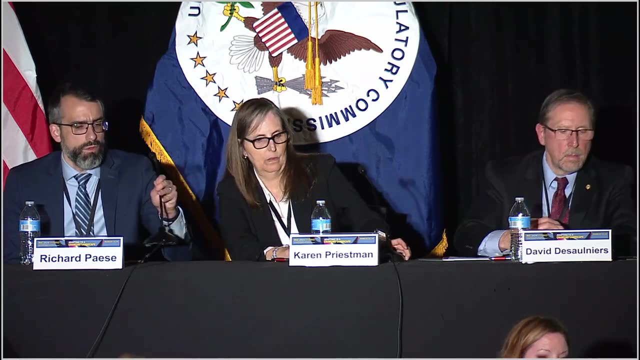 I don't think it decreases the challenges. I do think there's a place for automation and I think there are plans, especially the smaller plans with the lower consequences, where I think it just makes sense to automate. Yeah, I'll say, you know, based on my presentation, of course I am a proponent. 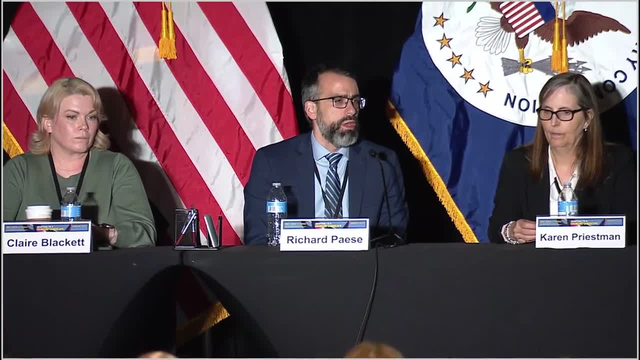 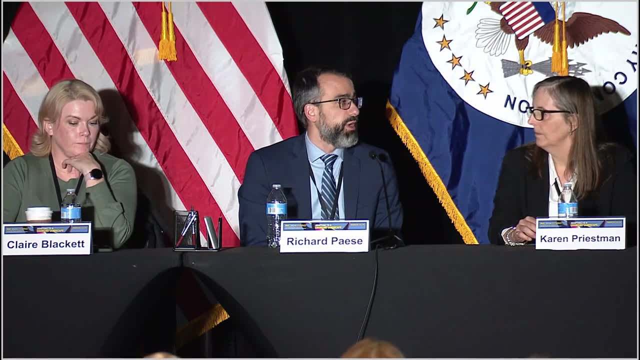 of increasing the use of automation and you know, at the same time, understanding the implications And we've seen, you know, in the industry, where you know direct benefits from the increased use of automation in our existing operating fleet of reactors, where we've been. 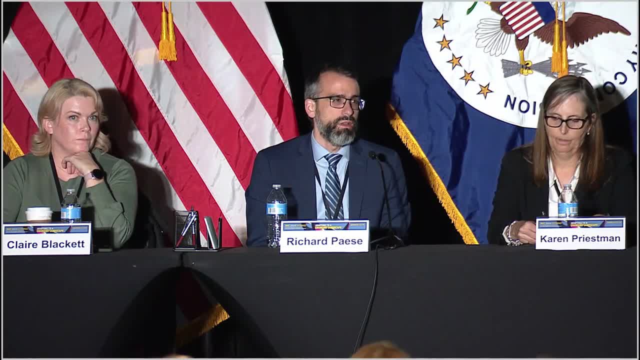 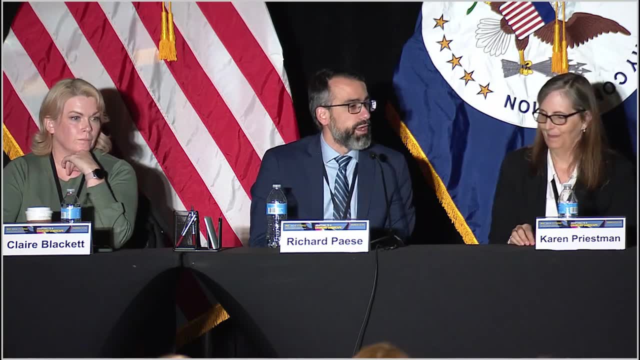 able to. I talked a little bit about self-diagnostics, where the system can detect failures, and sometimes failures that the operators can't even see, And we talked about AI. I know we're going to talk about AI more later, but AI could even enhance that. 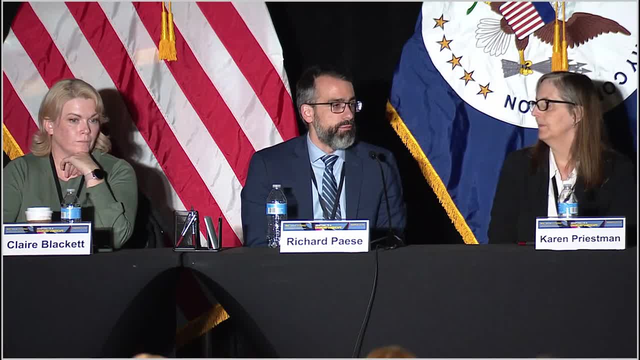 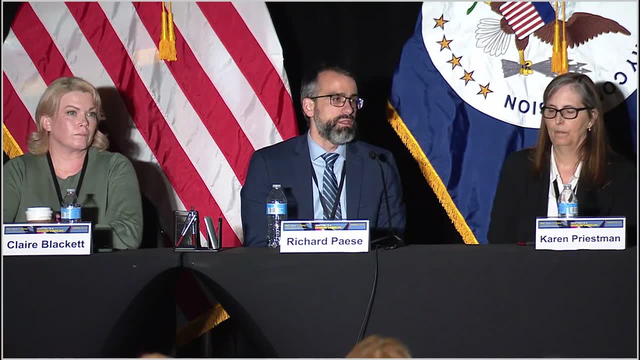 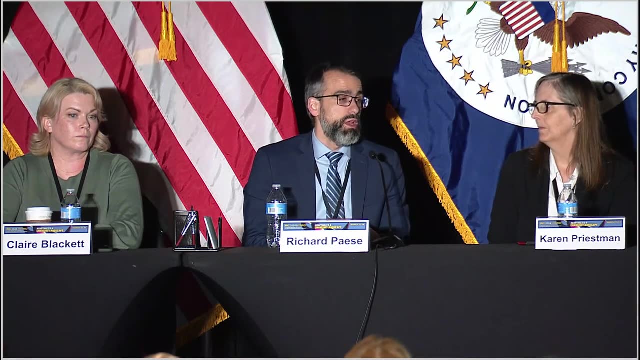 But we've seen real, tangible benefits for that, Also from an operation and maintenance cost standpoint. where think about if you can now credit the system to perform some of these activities. you've now reduced the effort, and not only reduced the effort of performing the tests, reducing the effort to maintain. 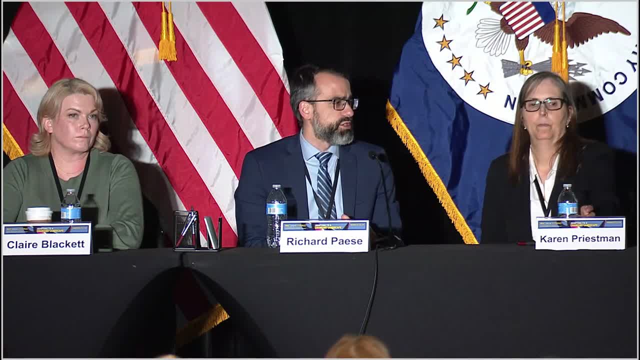 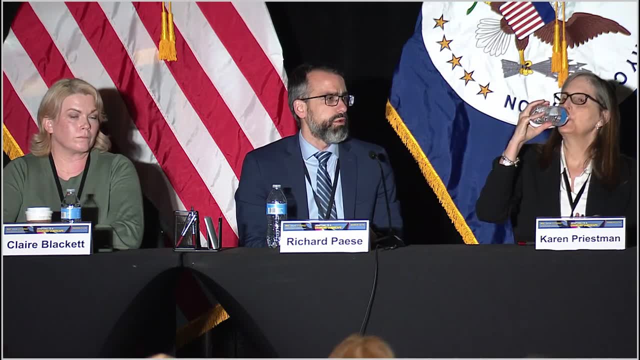 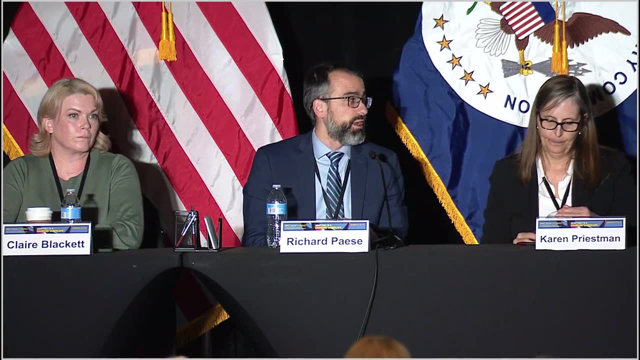 these testing and surveillance programs and procedures and also free up the operators and other support staff to focus on Things that may have more of a safety implication to your plan, And so I would offer that up- that we've actually seen real, tangible benefits today and now. 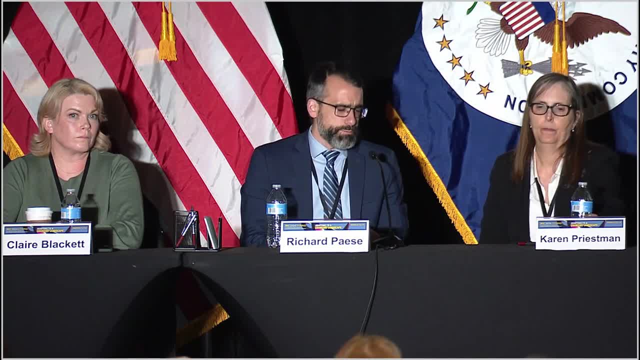 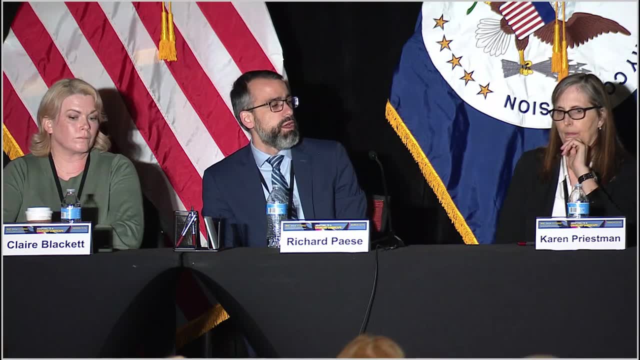 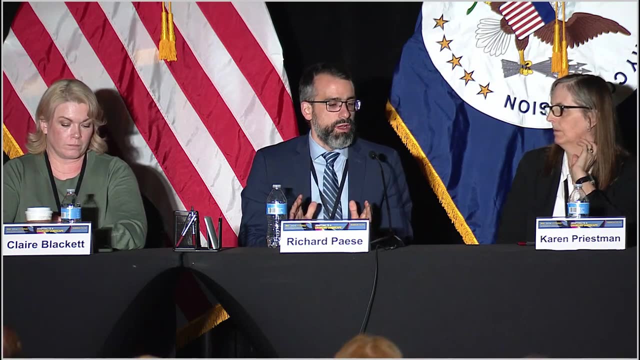 with the increased use of automation. And I'll also say you know we've been talking a lot about this increased use of automation and you know I've talked to this question to one of my colleagues and it was noted that you know there is a potential idea to sort of provide some standardization on the use. 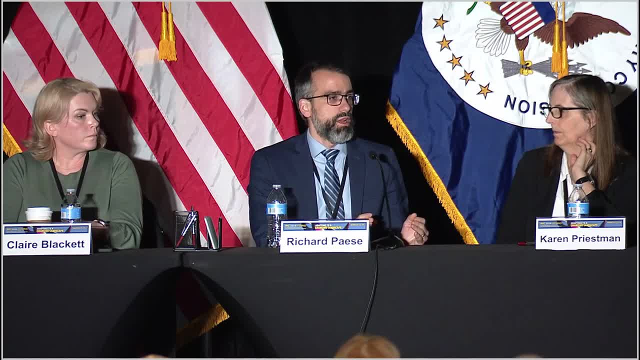 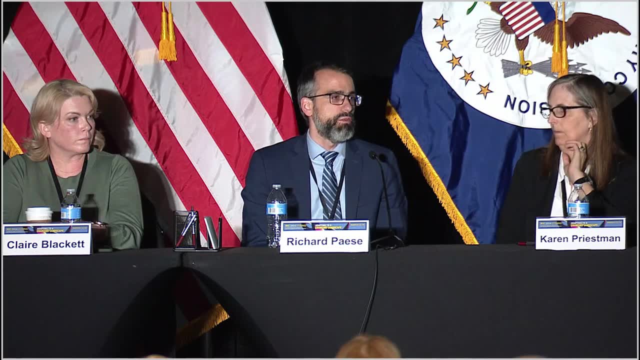 of automation. And so you know, one of the things that we've been talking about is, you know, we've been talking about the importance of automation and the importance of the use of automation and the importance of the use of automation. And so you know, in human factors speak, we talk about function allocation, where you 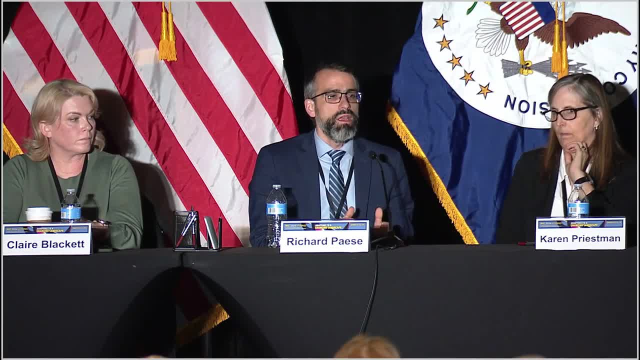 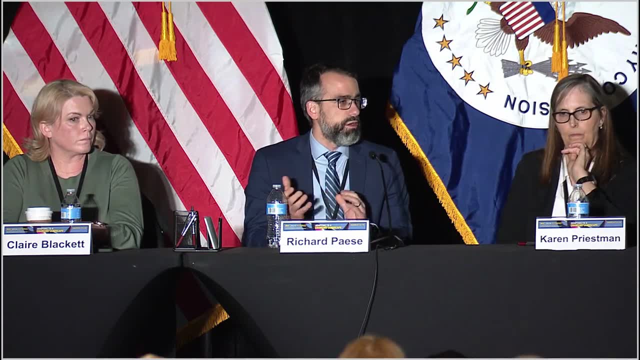 know, we go through all the functions and we say, okay, this is best for automation, this is best for the operator, or this is best for a combination of automation and manual control. And so perhaps you know, as we, you know, think about the functions that are consistent. 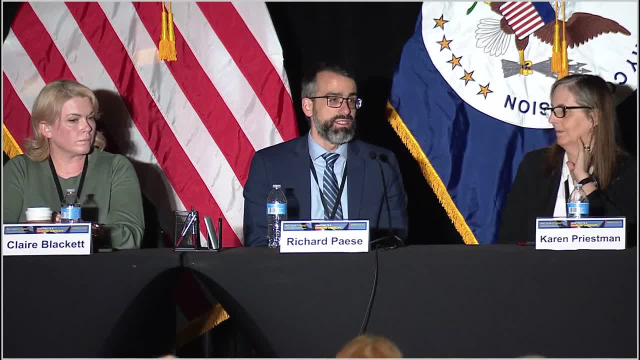 across our designs, which may be more and more of a challenge. And so you know, maybe we can, you know, think about the functions that are consistent across our designs, which may be more and more of a challenge as the design changes. 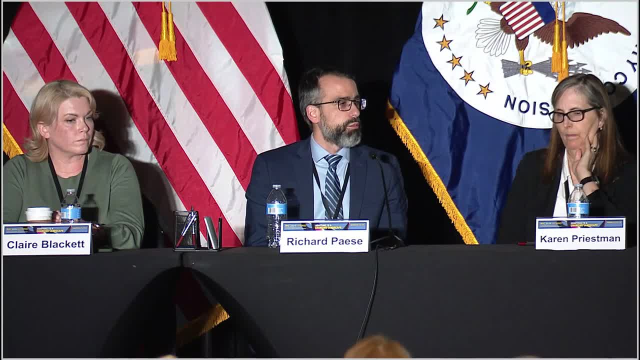 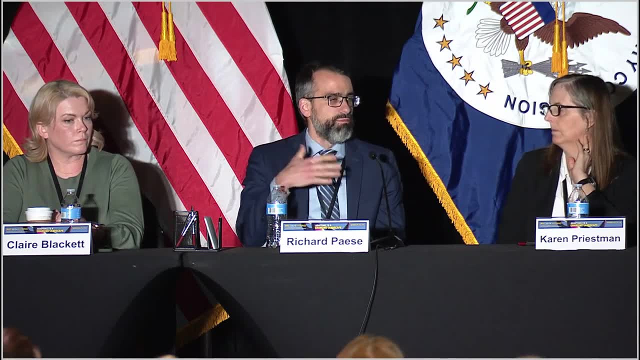 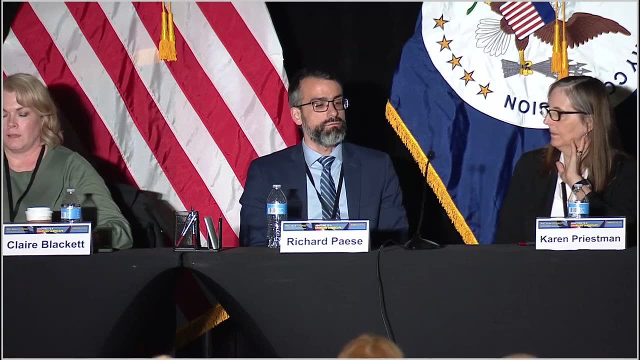 But, as we think through that, maybe there's an opportunity to provide industry guidance within our, you know, within our community to think about, you know, think about these questions from a holistic standpoint and not just from an individual standpoint. so, Yeah, I think that automation is something that is inevitable. 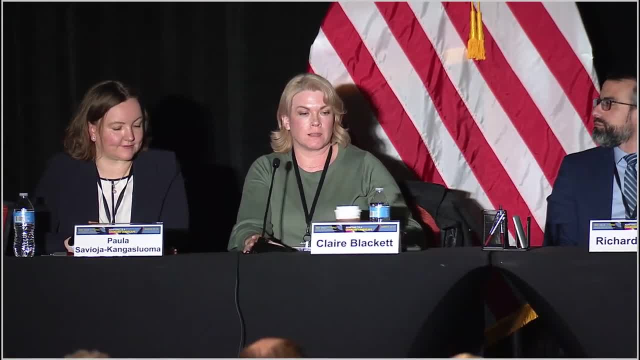 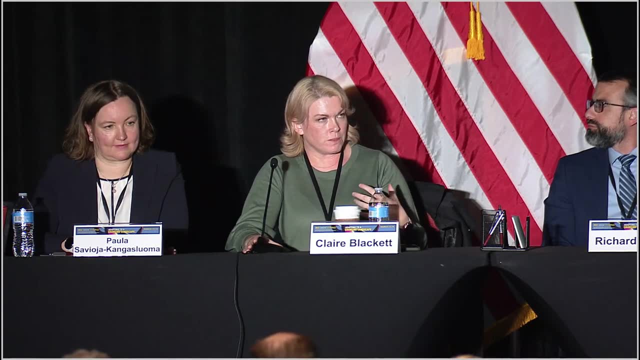 That will happen And I'm glad Rick said that. I'm glad Rick said that, that you actually touched on the function allocation part of it, because I know I'm not the first person to think this. but there is that question of just because we can automate something. 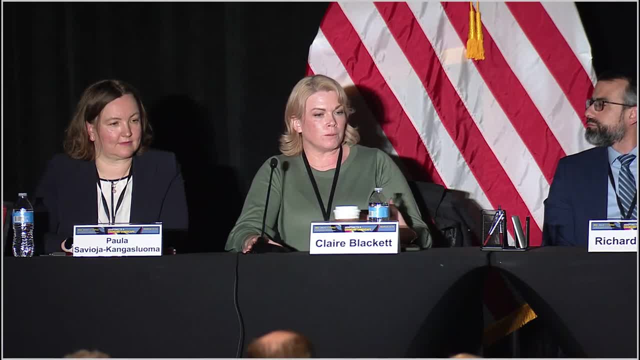 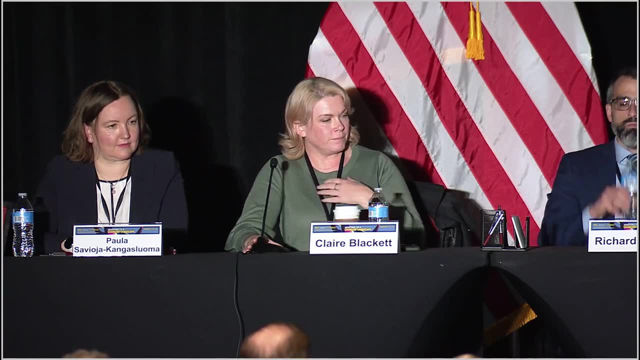 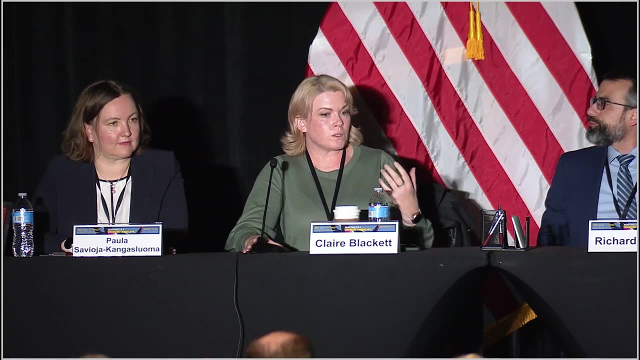 does that mean that we should automate it? So I think that when it comes to automation, we need to be very clear about what are our requirements or our objectives when deciding to implement automation. So one thing that is discussed a lot in SMRs, for example: 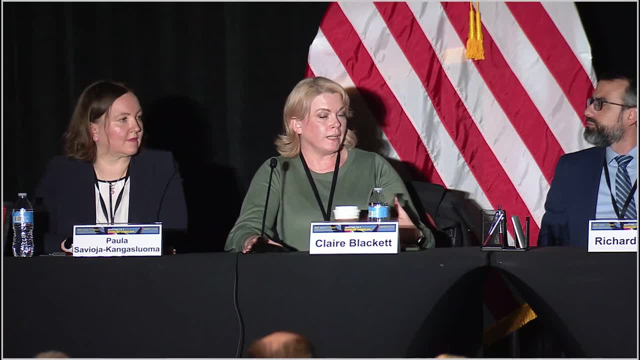 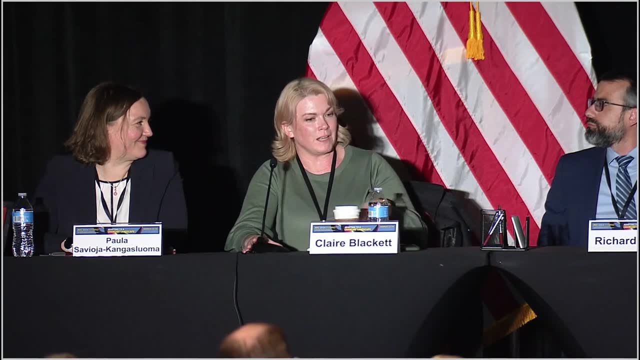 is the opportunity to reduce the number of staff per reactor unit, And I often hear that that is discussed as well. we can automate the plant so we can reduce staff, And it makes me ask the question: are we automating to only reduce staff? 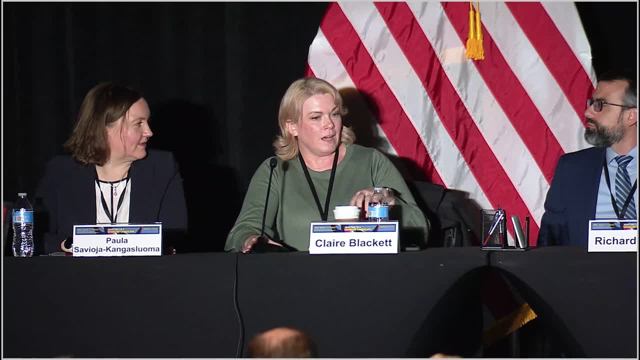 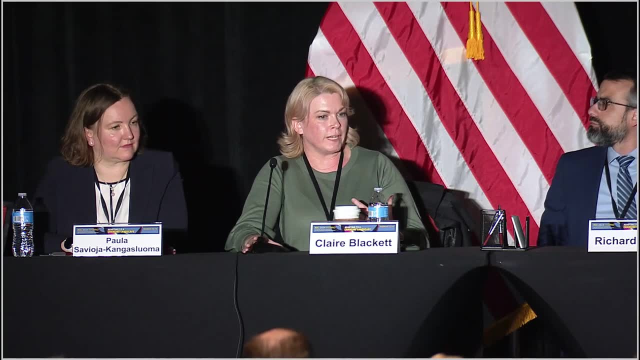 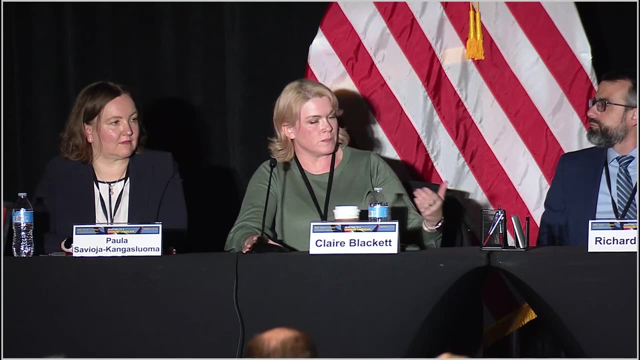 or can we reduce staff because we have automated? And I think that those are kind of slightly different sides of the coin. We need to be very careful about where we are automating and why we are doing that, because it will actually impact upon other systems and subsystems. 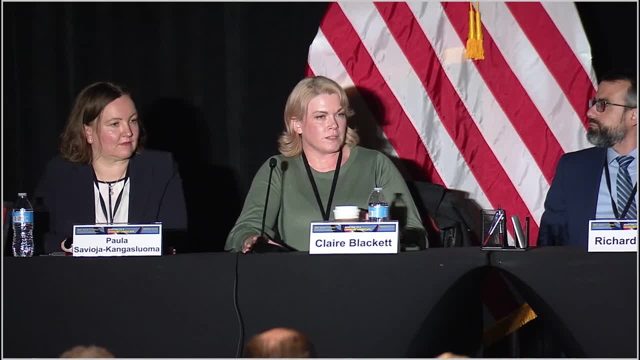 It will impact on the operators. We have this idea that you know, especially in SMRs, because we'll have increased use of automation, increased reliance on passive safety systems- that if something goes wrong, the operators can be hands-off for up to 72 hours. 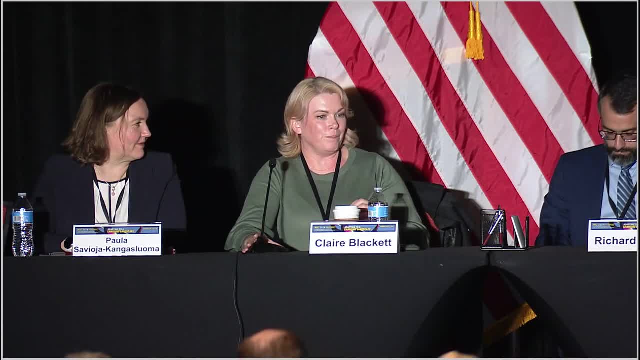 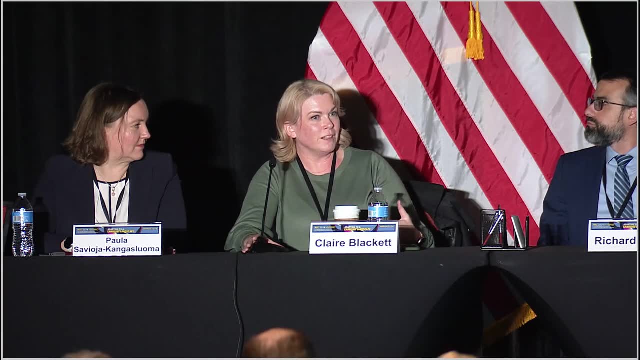 That's not true. The operators will be doing a lot, And so I think when we talk about automation in relation to advanced reactors, we tend to kind of oversimplify what we're talking about and thinking that well, if it's automated, we don't need operators. 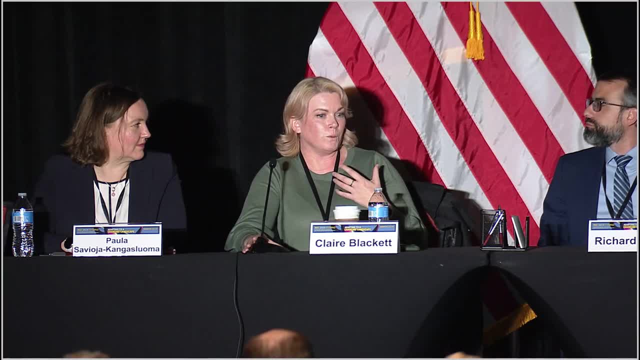 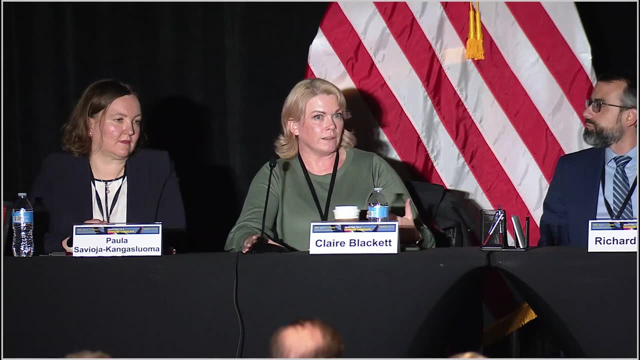 And that's very much not the case. So I just think that we need to approach it carefully and examine it thoroughly to make sure that we're not oversimplifying, we're not overlooking something that could actually fundamentally change how operators work in the plant. 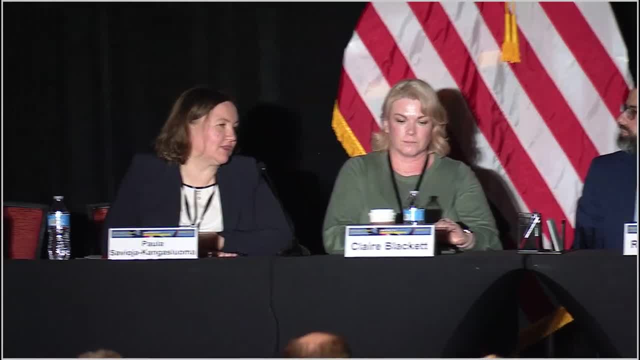 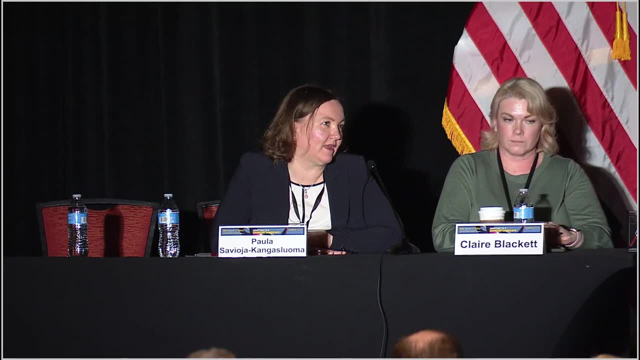 Yes, I agree, And I would like to add to that that, as automation is inevitable, it has to be and it will happen. but it means that automation must be designed with a proper human system integration approach and human factors engineering so that human collaboration with the automation is taken into account. 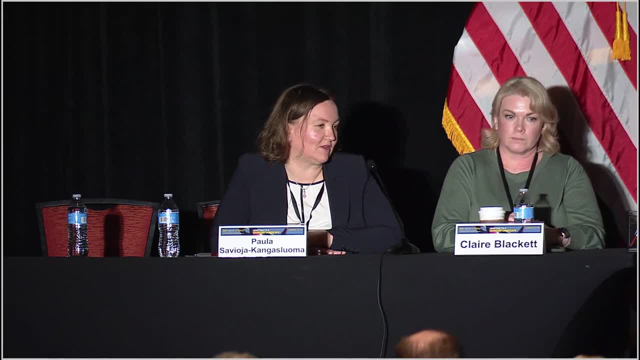 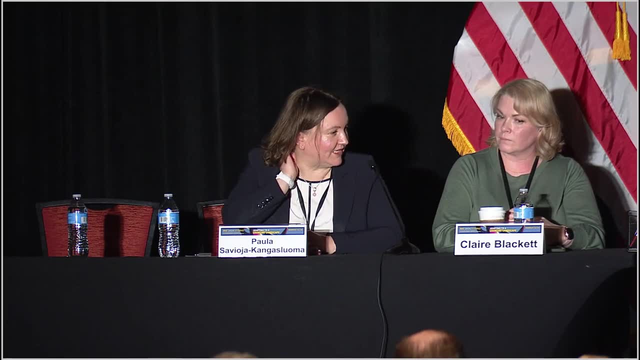 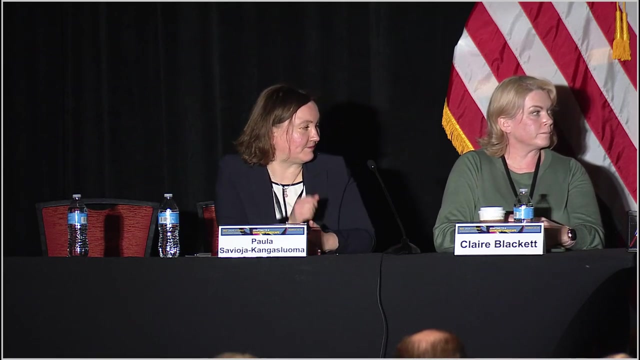 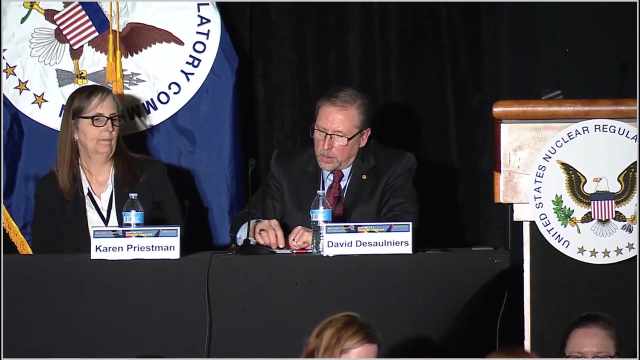 And for this we also Also, as human factors professionals, need method developments so that we can be properly integrated and understand the impacts of the automation on human activities. So I think we need development of methods and approaches, in that The comments, You know, kind of had the theme of touching upon the issue of function allocation. 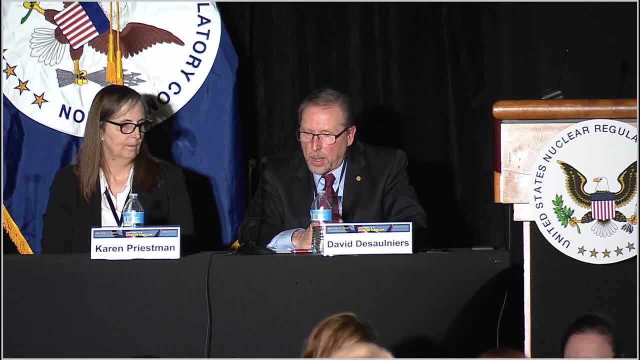 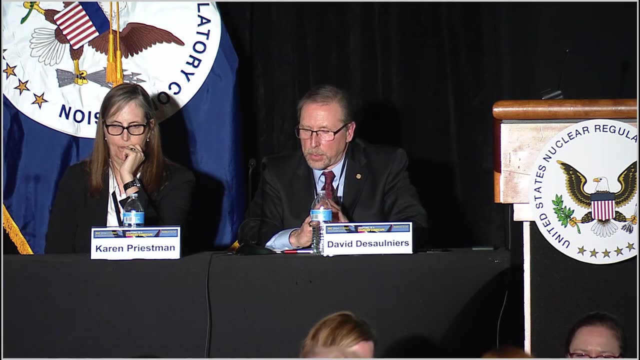 And thinking about this session, I went back to an old paper that I thought had some interesting thoughts with respect to where we are today in terms of automating plants, And I mentioned that acronym, MABA-MABA- Machines for Automation. Machines are better at, men are better at. 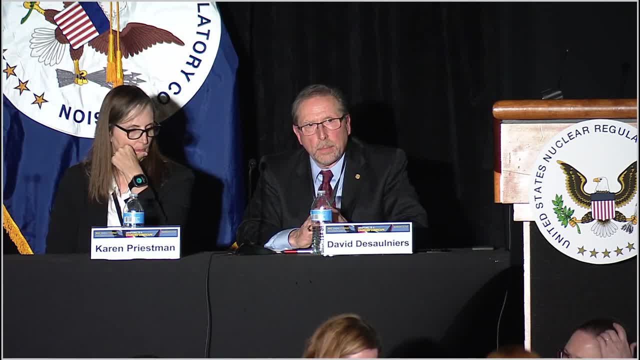 And the paper was written by two leading human factors professionals, David Woods and Sidney Decker, And it was Title in part: was MABA-MABA or abracadabra? And questioned this approach of simplistically perhaps thinking about, you know, just substituting. 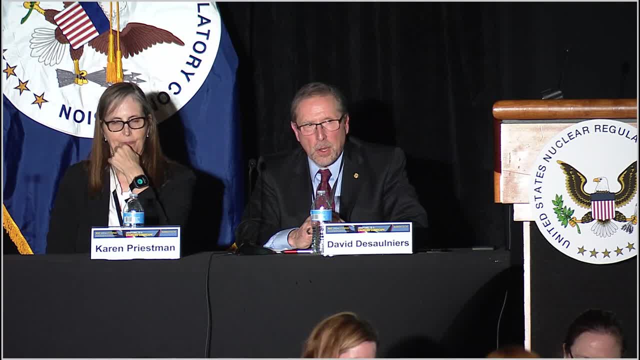 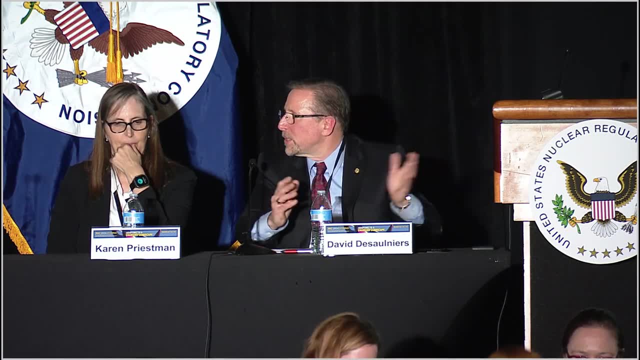 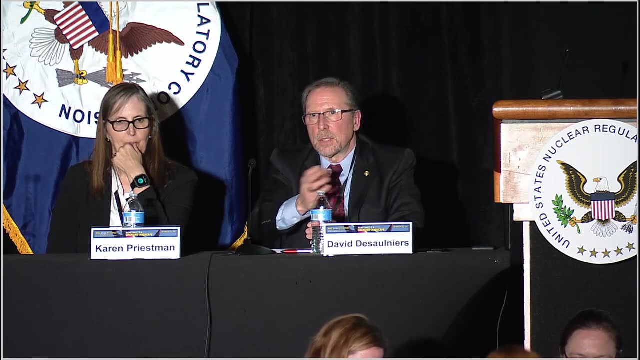 What a human used to do with automation And thinking: okay, you know we've come up with automation that can fix this human problem, problem solved. And you know they described that as kind of substitution, thinking That you were just substituting the machine for the human. 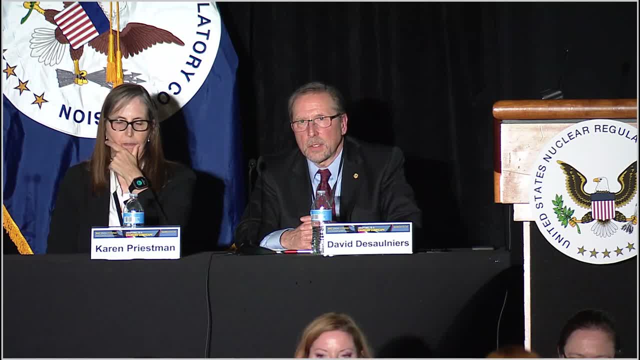 And not necessarily recognizing the kind of downstream consequences of what you've really done now. And more deeply, you know what we're really trying to do is fundamentally change the system and the way work is done, And that there needs to be, you know, more thinking in terms. 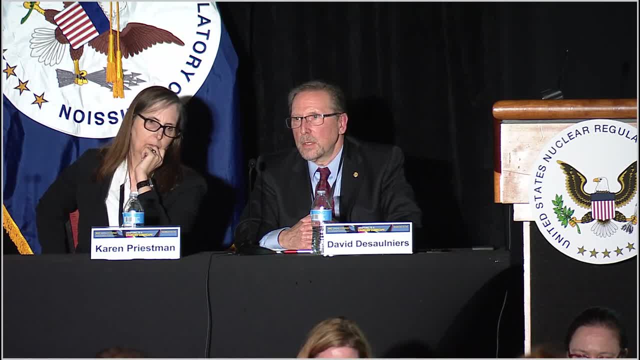 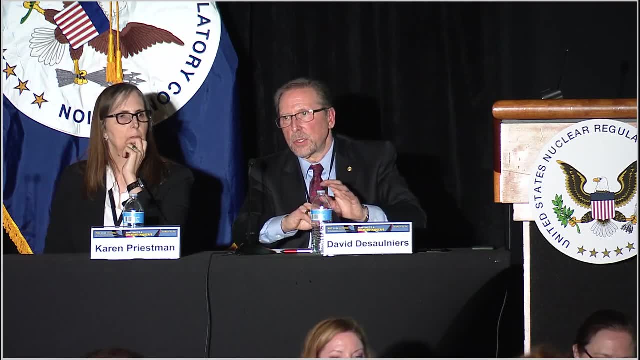 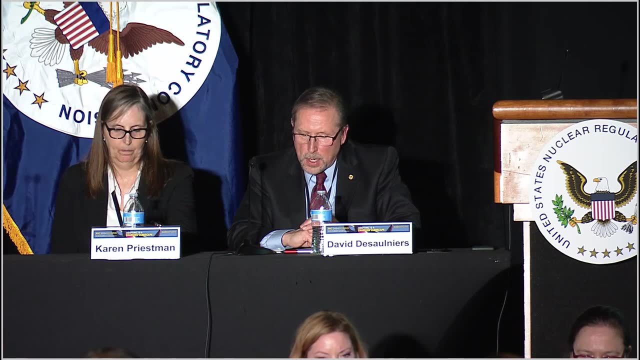 of just how to make humans and machines work cooperatively together, rather than just thinking about this division of labor notion, And I thought that was. they had an interesting statement in their paper that really struck home with me, and so I'm going to quote them. 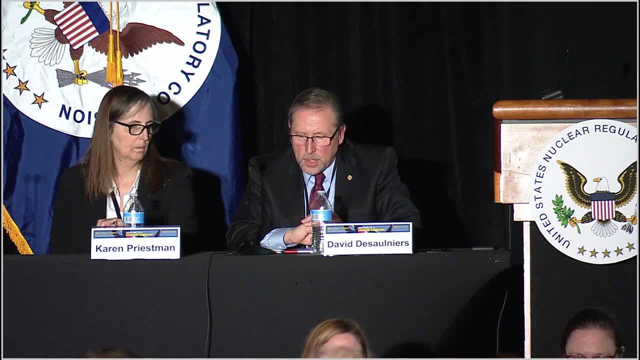 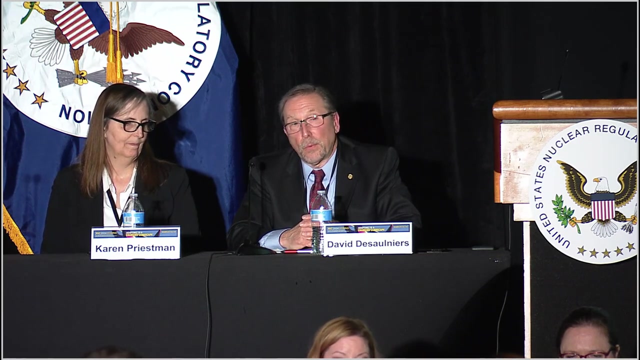 They said, design concepts represent hypotheses or beliefs about the relationship between technology and human cognition, And I thought that was just a very interesting observation. We think of design concepts. that's solid, You've got a way to move forward. But at the conceptual stage it really is. 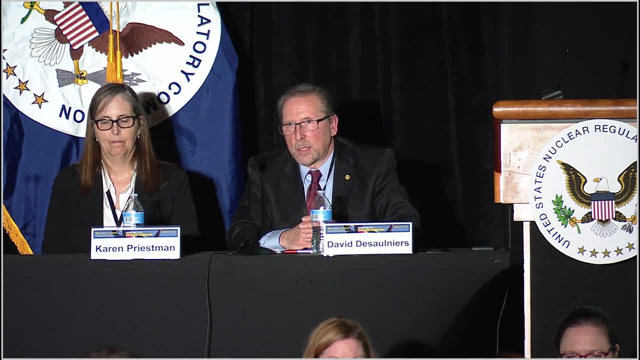 It's a hypothesis, It's a belief about how you think the system is going to work, And so they go on to then elaborate, to say: you know. such designers need to subject these beliefs to empirical jeopardy by search for disconfirming and confirming evidence. 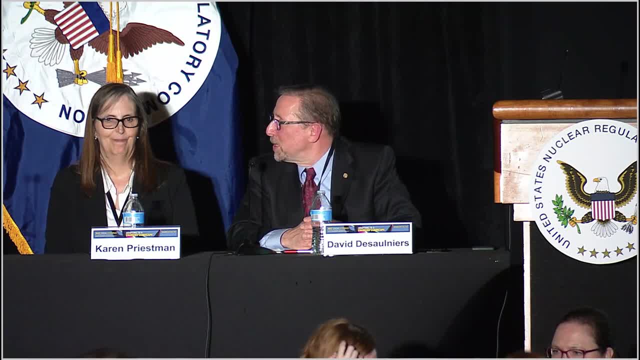 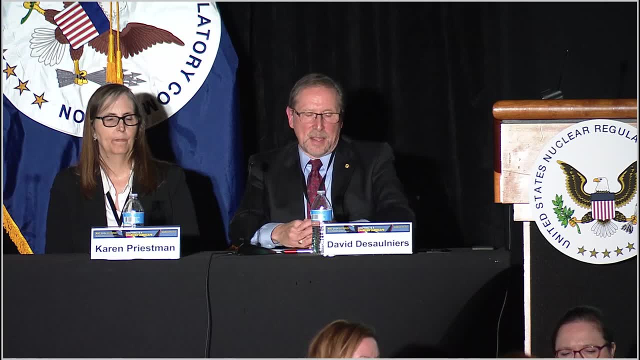 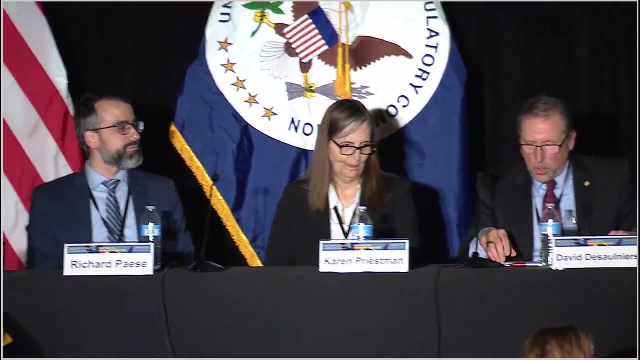 I like that phrase: empirical jeopardy. I guess I just interpreted it to mean validate, validate, validate. So We're getting near the end of our panel time. I'm going to see if we can take one more question quickly, and then we will need to wrap. 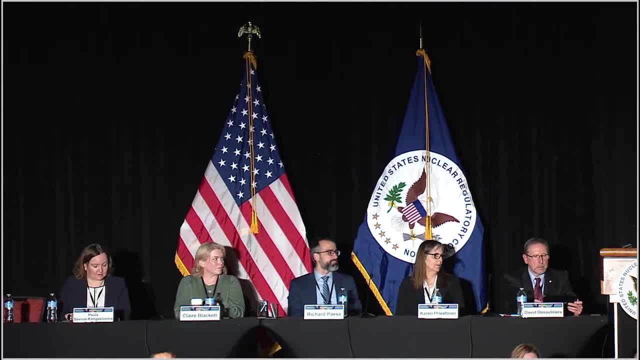 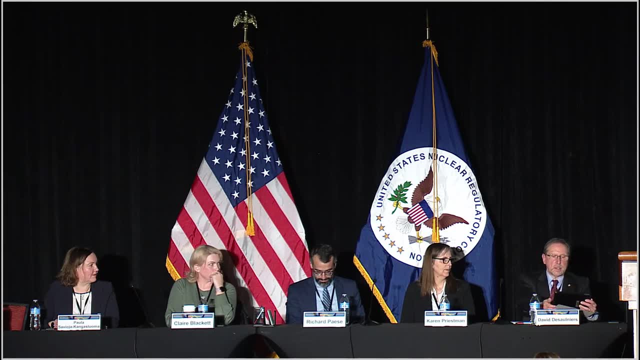 There was a question from our audience. This is an interesting one, Rick. it was directed. It was directed to you, But I invite others to weigh in. Do you think that we are safer shifting the opportunities for human error from operators to designers? 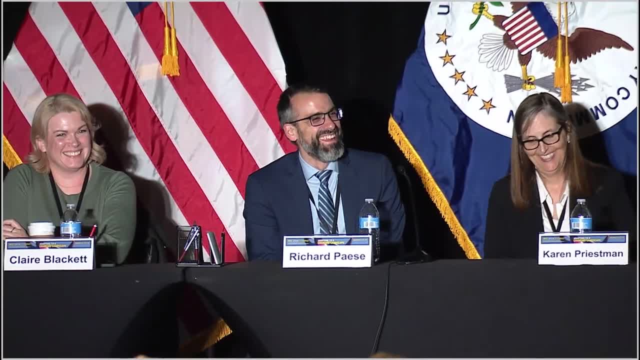 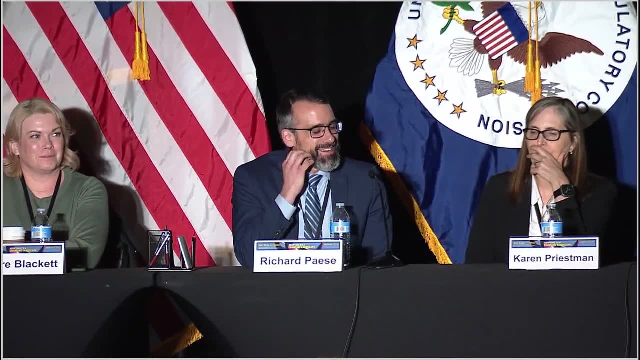 Well, they're both humans, right? So I don't know if there's any shift going on there. I don't know. I think I understand the basis of the question, But, you know, I think it's getting on to the point that I was talking about. 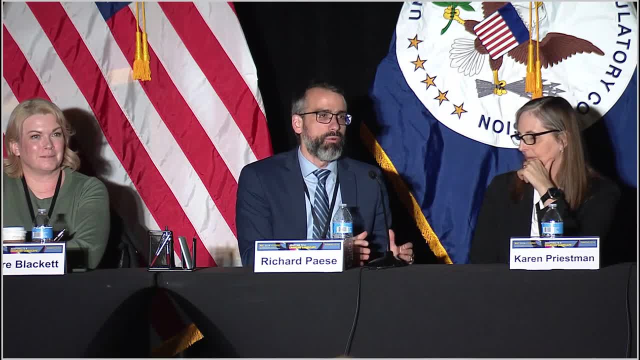 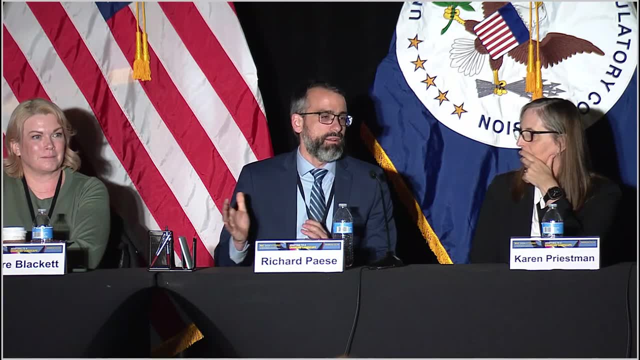 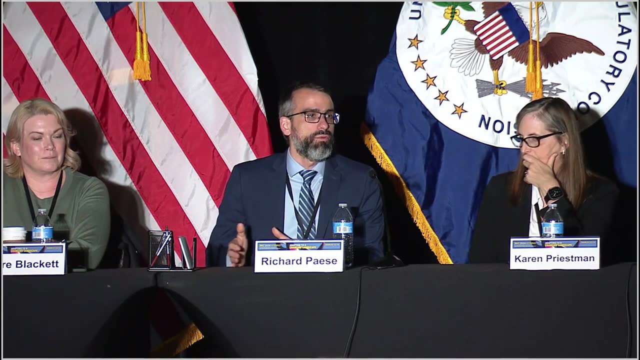 You know we have an opportunity to reduce, you know, human error and therefore making the plant safer by automating, And I think that's true. But you know the second part of that, my thought on that that I presented, was: you know you could go too far, in my opinion at least, too far the other way if you make your system too complex, right? 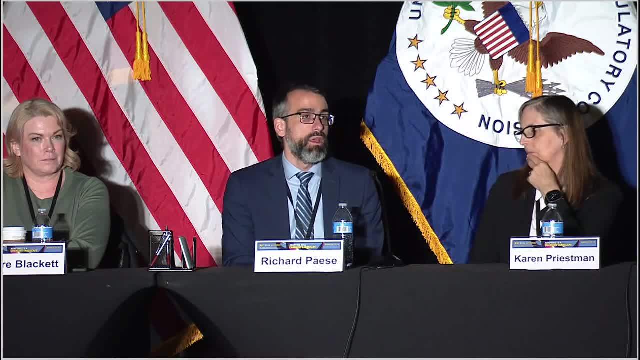 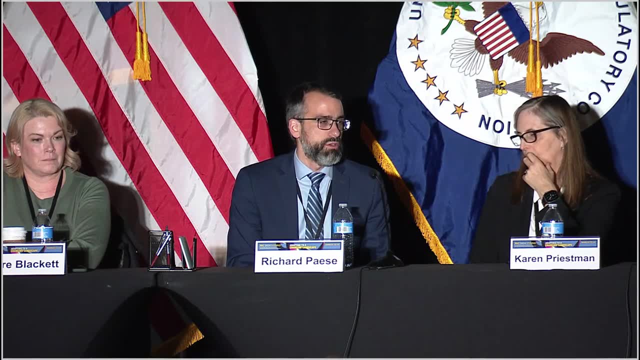 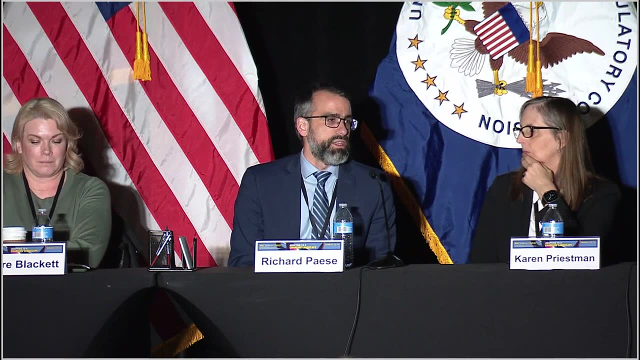 You introduced the potential of making you know maybe a quality error Or a requirements error that goes undetected within the system until you know it manifests itself as an error. So certainly I understand that point and I agree, And so I think the theme that we've all been talking about is: let's not automate just to automate. 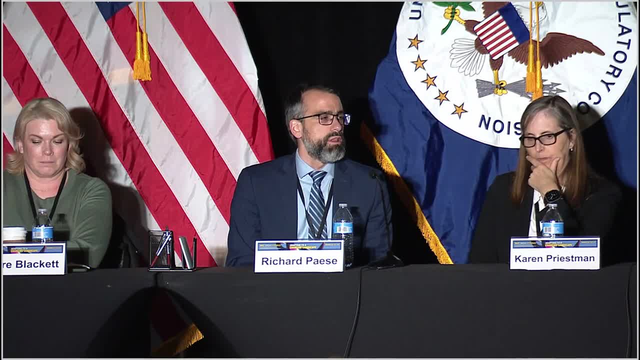 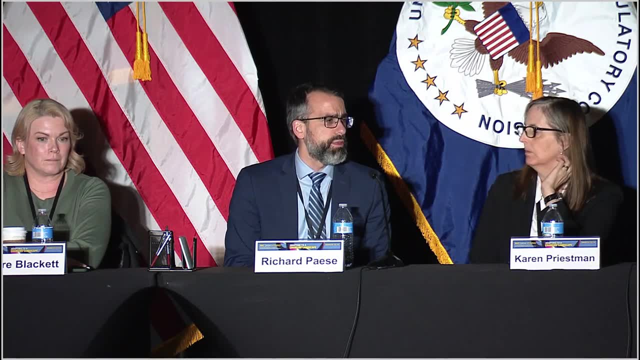 We need to think through the implications and how the operator is impacted to that automation, how training is impacted Training is going to be. we haven't really talked too much about operator training and human training on. you know, as we go to advanced systems, 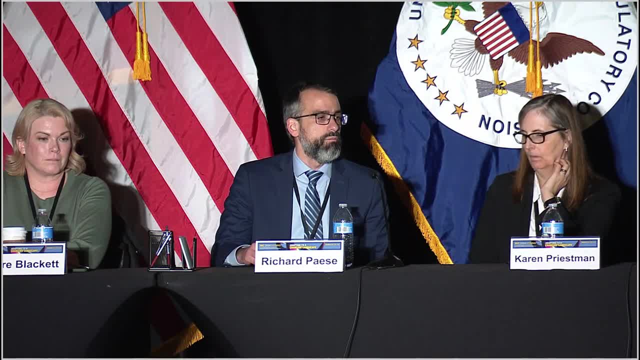 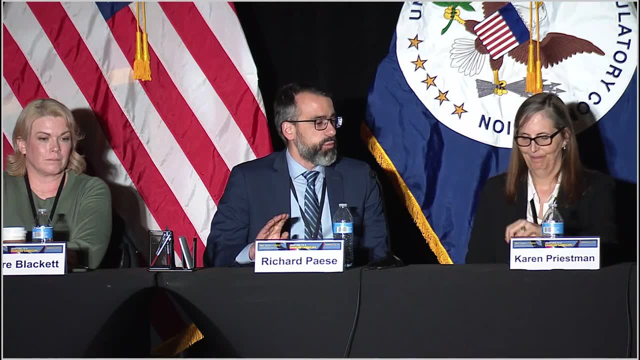 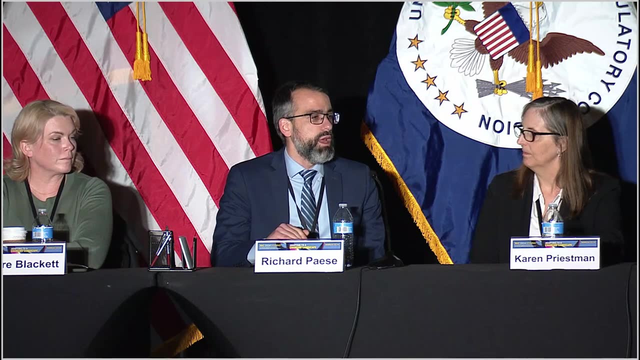 But that's a really key piece of this is one thing I'll say. I know we're short on time, but I really wanted to share this in 30 seconds. this example: You know I've seen operators where using newer systems, where you can actually you know if you where they received a failure of the system and you can actually see within the control logic of the system you know troubleshoot, actually dive down into the control system of the logic to see where the system may have failed. 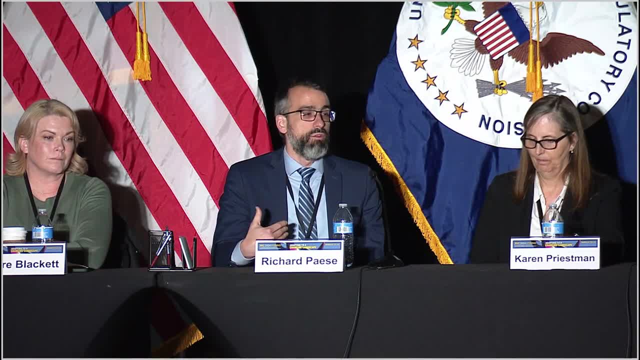 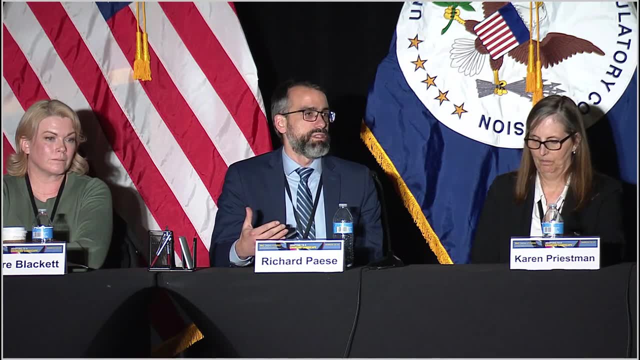 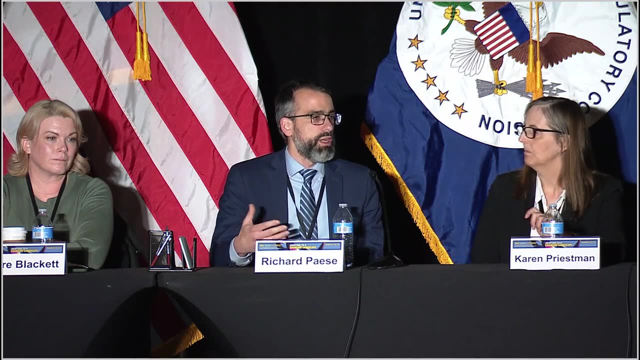 And what I have observed in my personal experience Is that operators are very quick to do that as soon as they get a failure, to drill down deeper into the digital system to figure out what failed in the system- And it was intuitive to them, you know, and so I think there's an opportunity there to retrain, provide more training and more skills to those who interface with the system to be able to interact with the plant more effectively to find these faults. 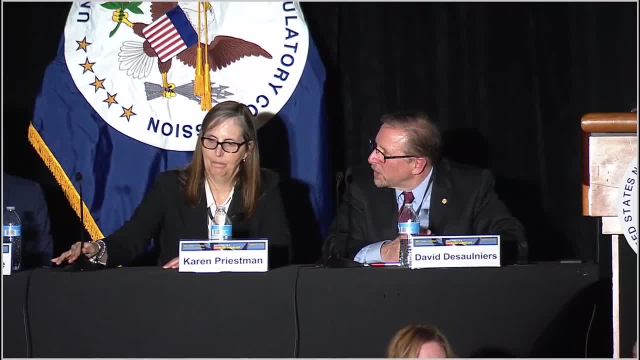 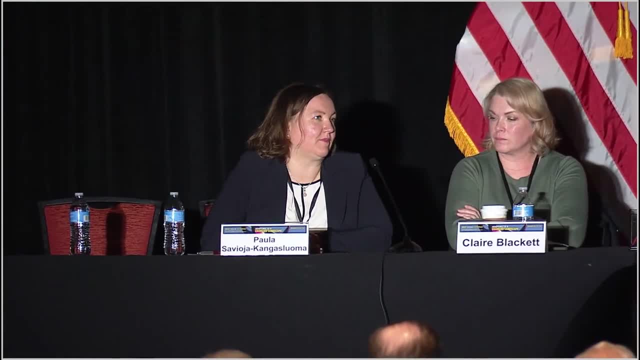 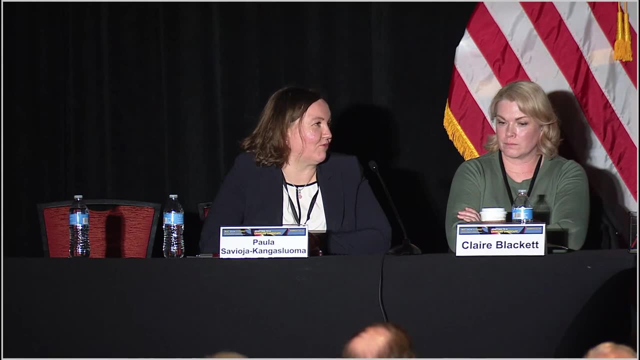 Thank you for that observation. That's a good point. Anyone else want to add on to that? I could add that, with the commissioning of our new EPR and the qualification of our control room operators, that's something that we identified. that must be paid attention to is the automation competencies of the operators. 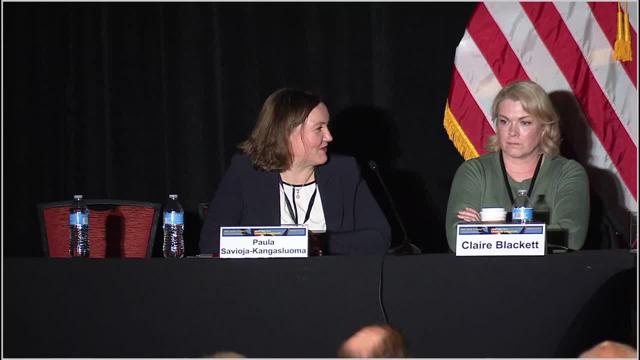 And we really tried to enforce that. So I think it's a really important aspect of this higher level Levels of automation That even when we have the sort of traditional control rooms, the operator abilities might and the requirements on their competencies might change a lot. 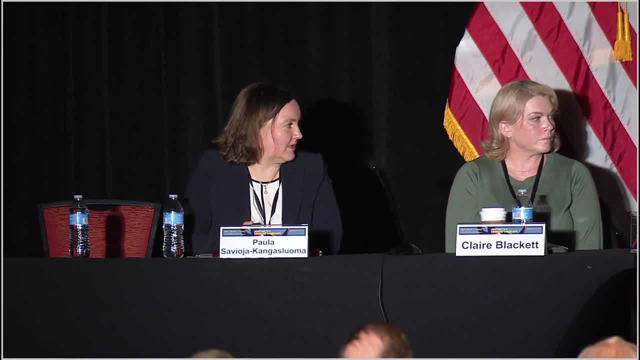 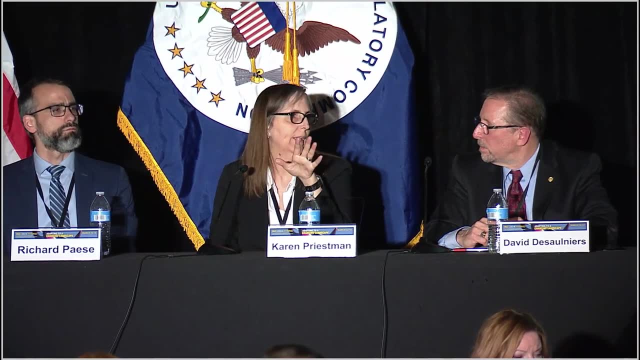 Can I have it? Sure, And I think that's what I meant when I started with- is that we need to understand the risks. They don't go away, They just move. They change The risks to the competency, The risk to the training. 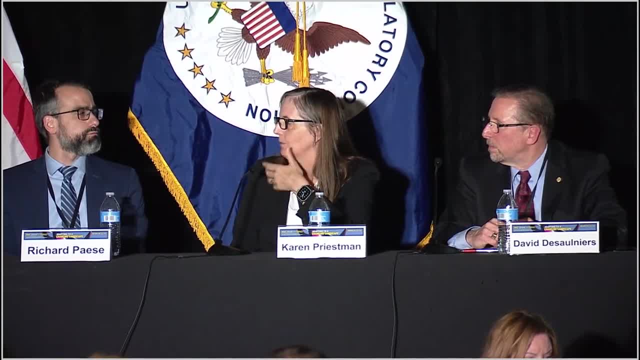 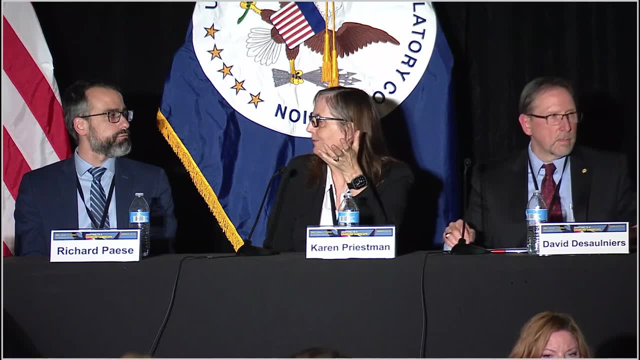 Who it is that's carrying the human error risk when we automate. So I think that's in line with what I was saying. It's this idea that suddenly you've gotten rid of these risks of error and these risks of, you know, humans doing stupid things. 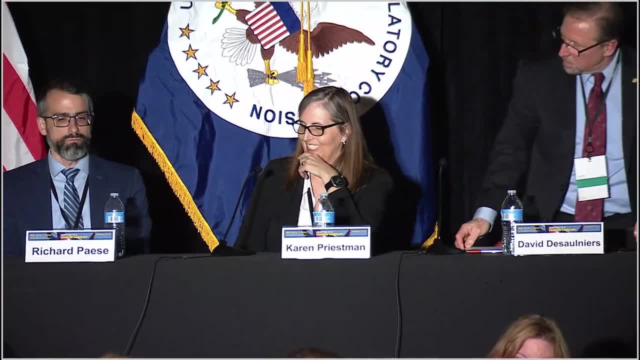 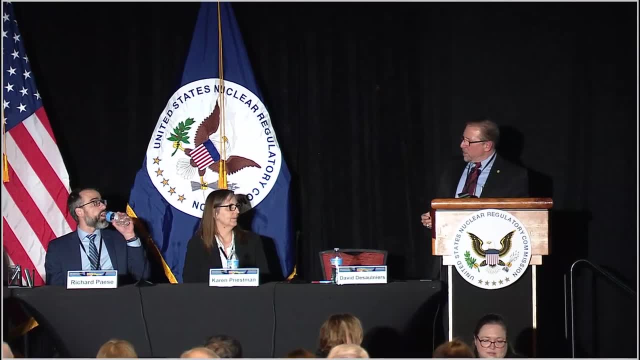 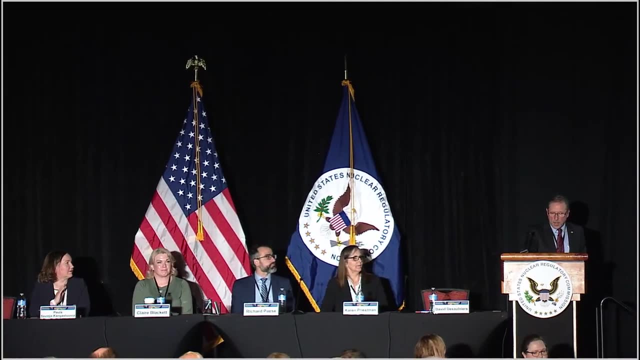 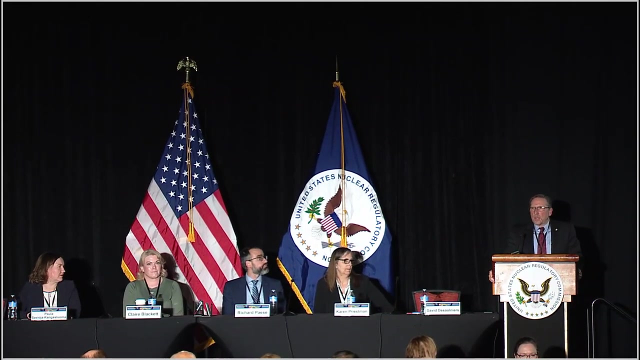 And it's no, we're still in the equation, We're just elsewhere. I'm happy to end on that note, Because I think that's Certainly a matter that I have been kind of beating the drum on for some time now is for us to keep in mind that, as we move to simplified and highly passive designs, we don't even need to be talking about automation really. 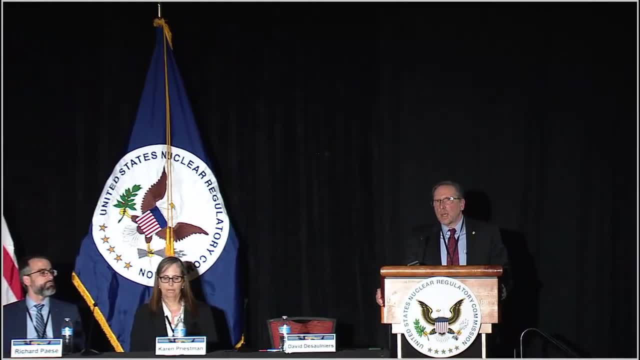 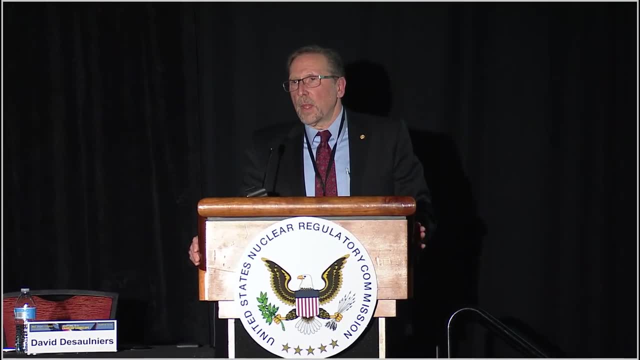 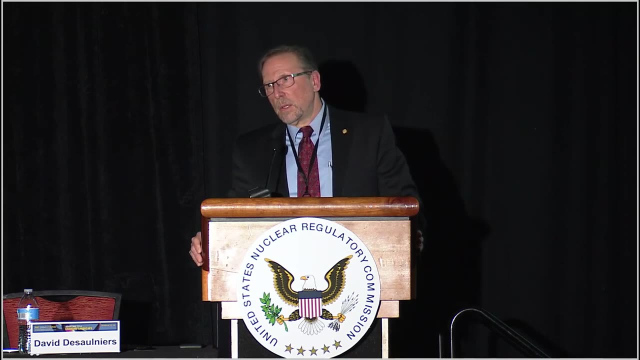 We're just thinking about designs that have now limited the need for operator intervention to address plan upsets. If you're relying on Passive systems or inherent safety characteristics, you are then, as we've just been speaking to kind of shifting where you need to consider the focus in terms of the potential for human error. 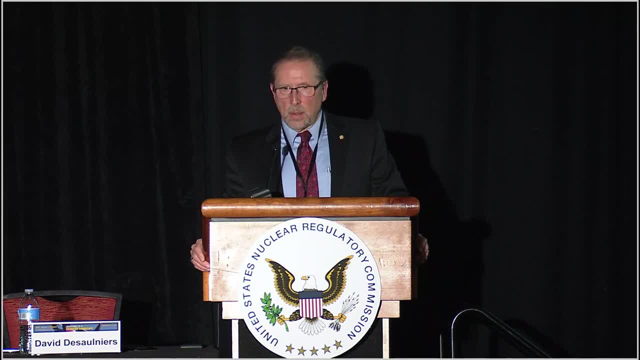 Is it now going to be with the field operator that ensures the proper lineup of that passive system, or the individual doing the surveillance, that's, looking at the integrity of the materials of that system, Or does it go all the way back? That's the first question implied to the design engineer.